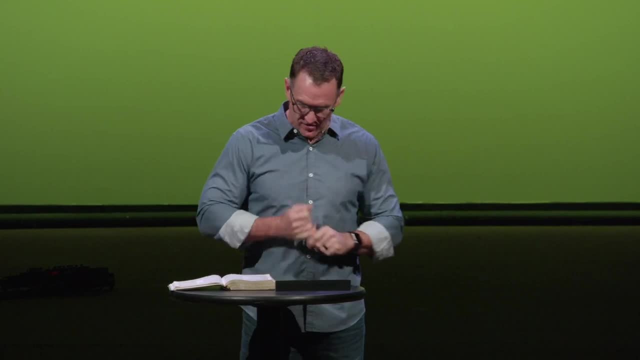 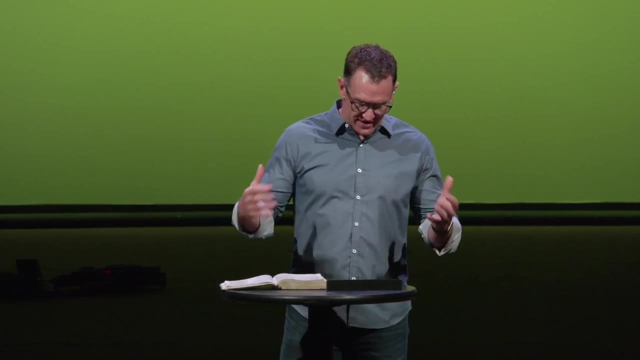 room. So let me explain why we're doing this series. There's two men standing on a bridge. One is about to jump to his death and the other one is trying to talk him out of it. So the man asked the jumper: so are you Christian, Are you Hindu, Are you Jewish? 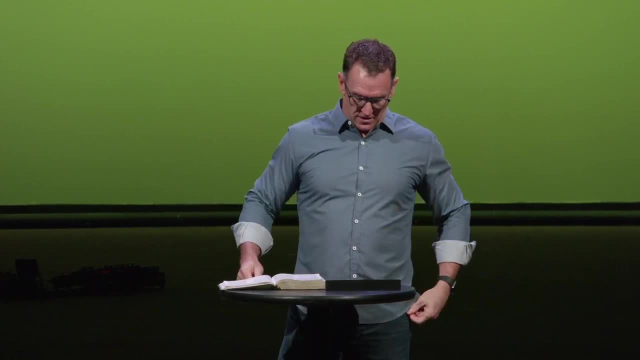 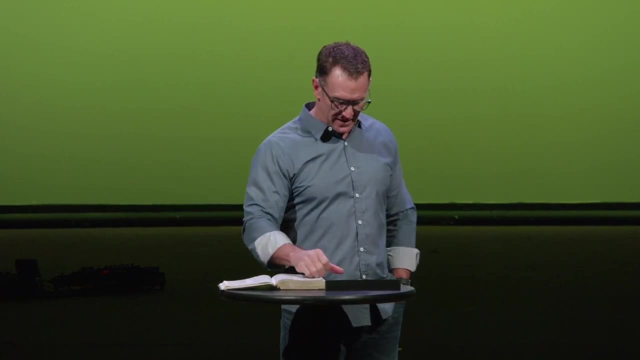 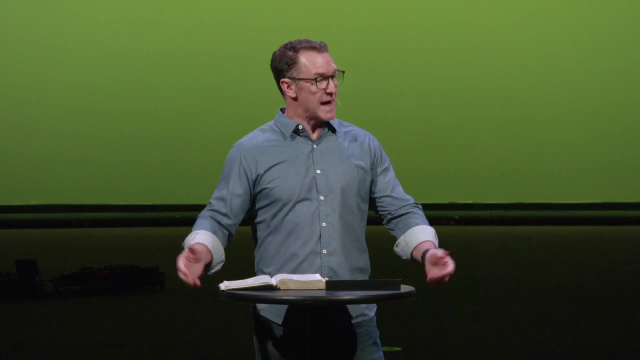 The man says. the jumper replies: I'm Christian, And the man says: small world, me too, Protestant, Catholic Orthodox. And the man says: the jumper answers: Protestant. He says me too. What denomination? And the jumper says: well, Baptist. And the man replies: me too, Southern Baptist. 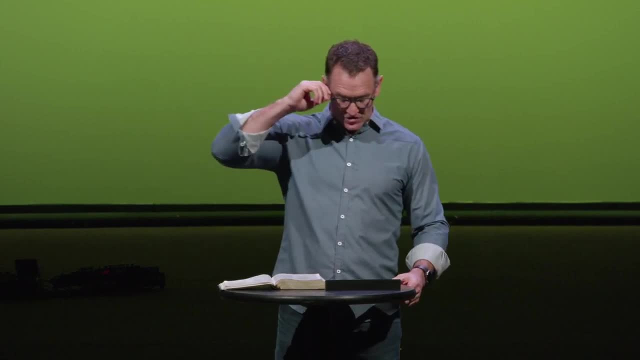 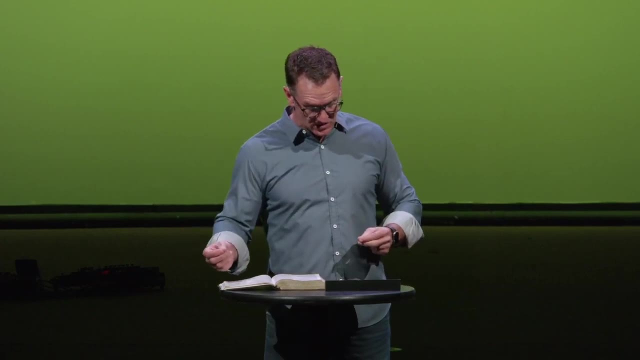 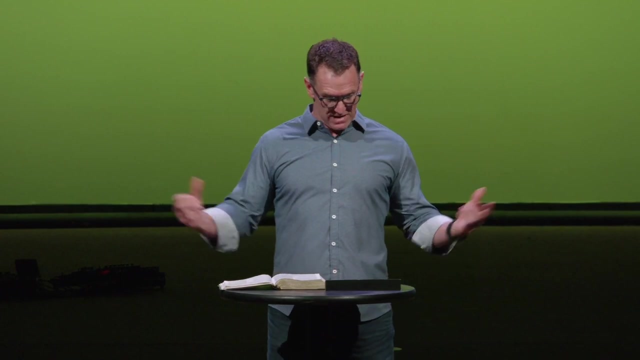 or Northern Baptist, And the jumper answers well, Northern Baptist. And the man replies: me too, Northern Baptist, Conservative Baptist. or Northern Liberal Baptist, And the jumper answers Northern Conservative Baptist. The man replies: me too, Northern Conservative Baptist, Great Lakes region. or Northern Conservative Baptist Eastern region. 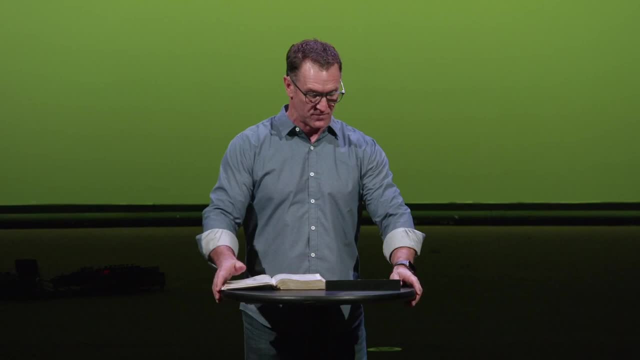 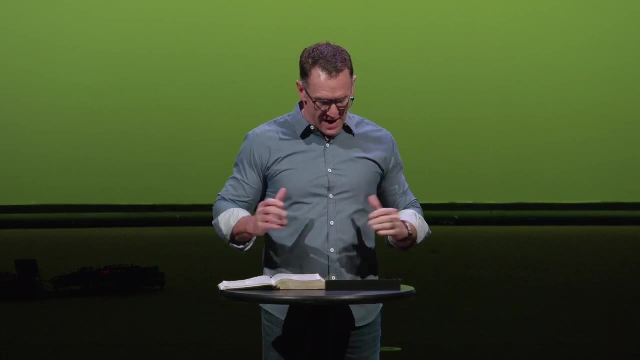 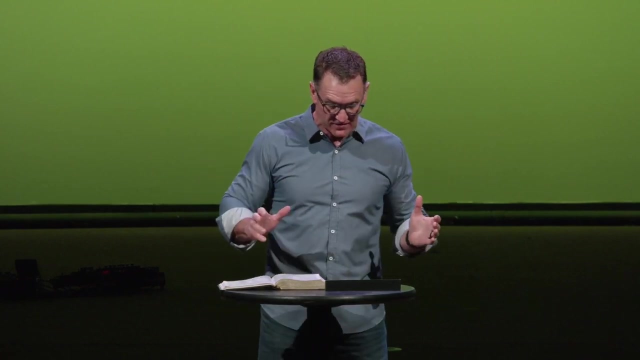 And the jumper answers: well, Northern Conservative Baptist Great Lakes region. The man replies: me too. Northern Conservative Baptist Great Lakes Region Council of 1879 or Northern Conservative Baptist Great Lakes Region Council of 1912?? And the jumper answers: 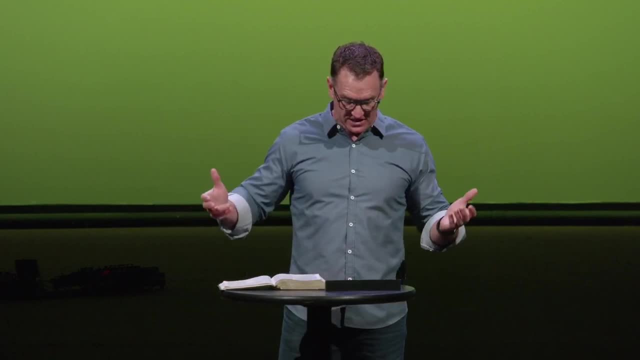 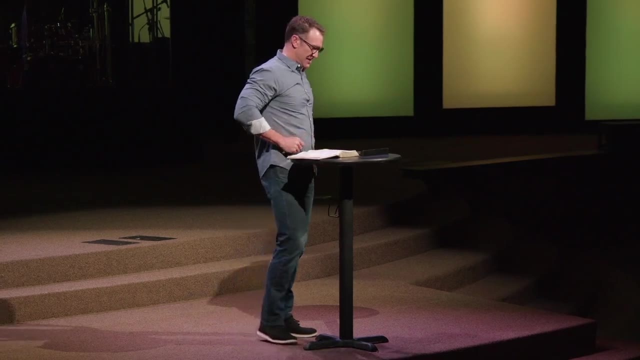 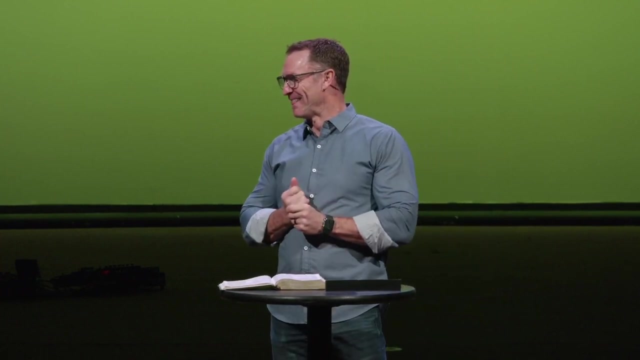 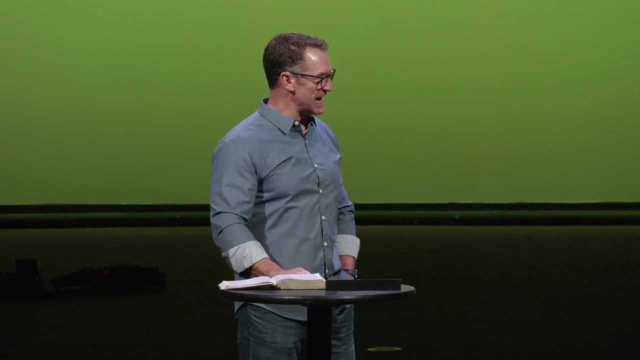 well, Northern Conservative Baptist Great Lakes Region Council of 1912.. And the man pushes him off the bridge and yells: die heretic. I thought that was funny. We live in a world that gets super divided over things And we feel like we have to make our statement about. 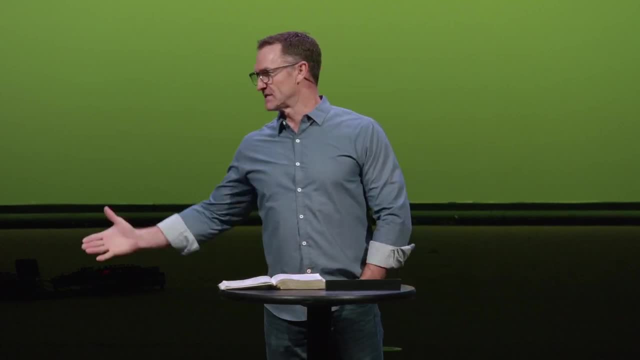 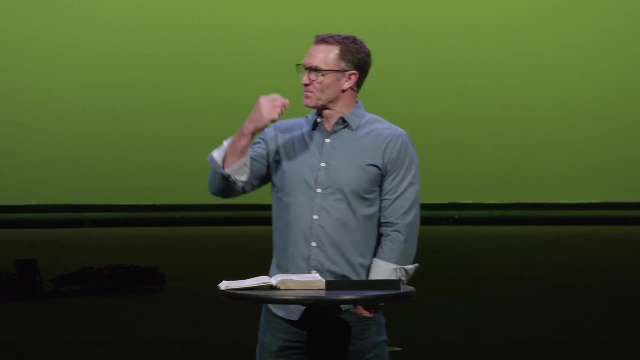 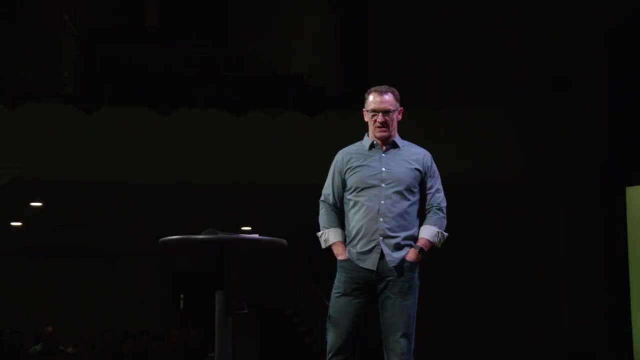 this is what I stand for, and anything that someone disagrees with. we actually can't have unity with them, which is just not the truth, And so we're going to talk about what creates unity for us. Jesus lets his disciples eavesdrop in on a conversation he's having with his dad. 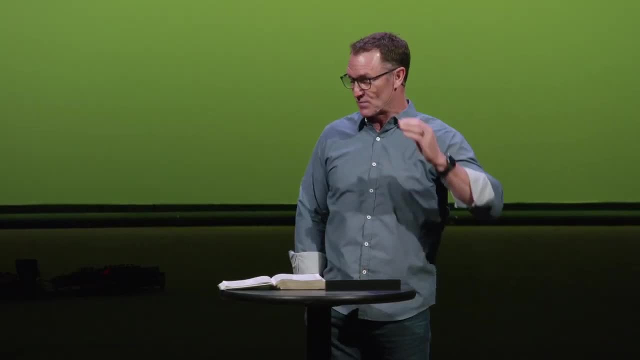 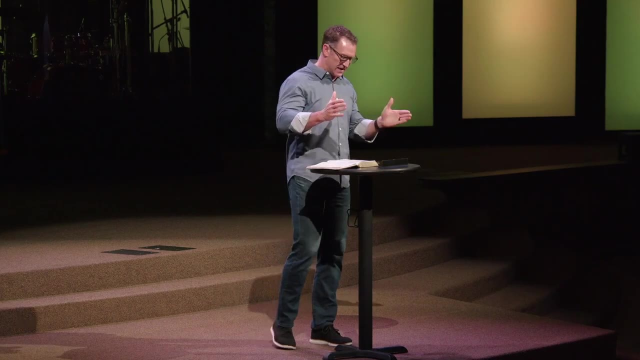 Jesus is praying and his disciples are listening to this prayer And he says, Father, I'm going to pray for all of those who will ever follow me. I pray that they may be one, just as you and I are one. And that same night, Jesus would tell his followers: 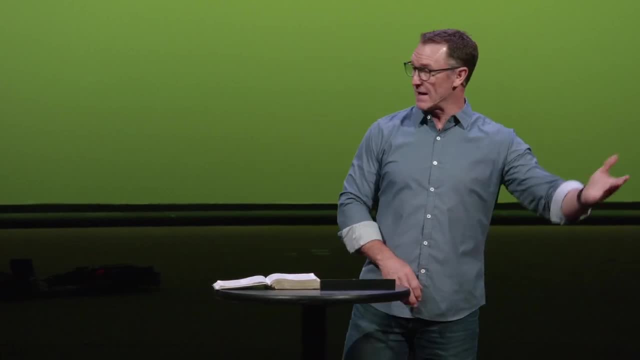 listen, this is how people are going to know. This is how the world is going to know. This is how your family is going to know. This is how your neighbors are going to know that you're one of my followers. It's going to be in how you love one another. 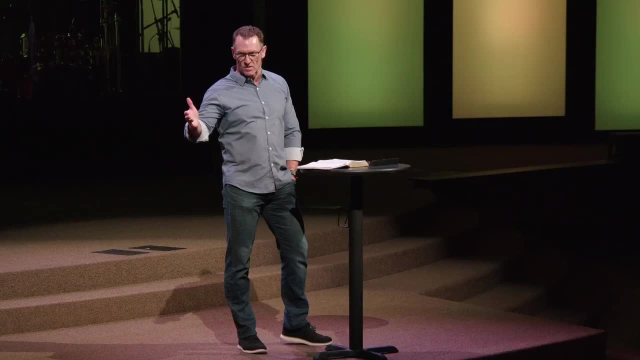 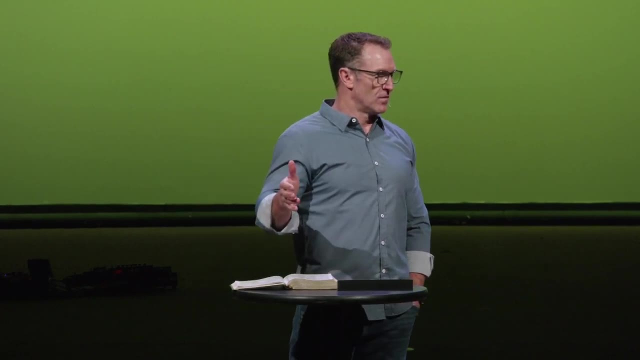 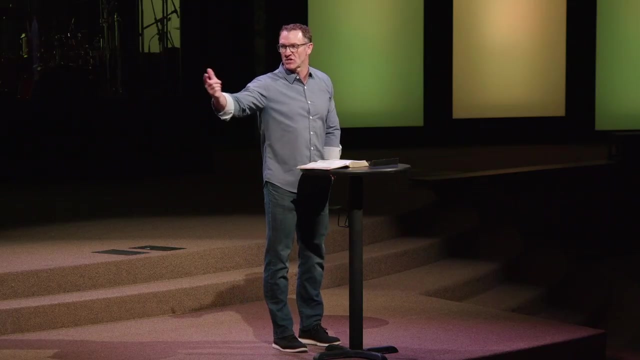 Our main task. this text is found in Ephesians, chapter four, verse three. It says: make every effort to maintain the unity. It's a clear call. Jesus prayed for it, He told his disciples about it, And then Paul writes to say: listen, it's about the unity of believers. 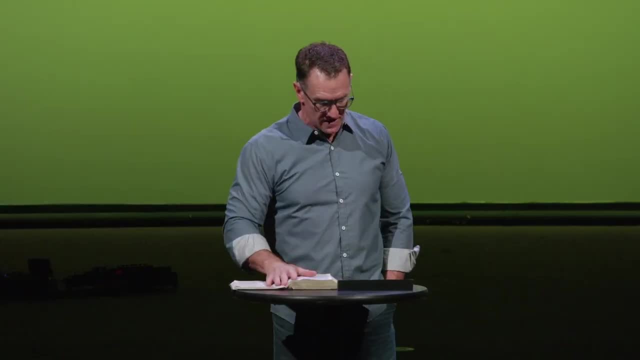 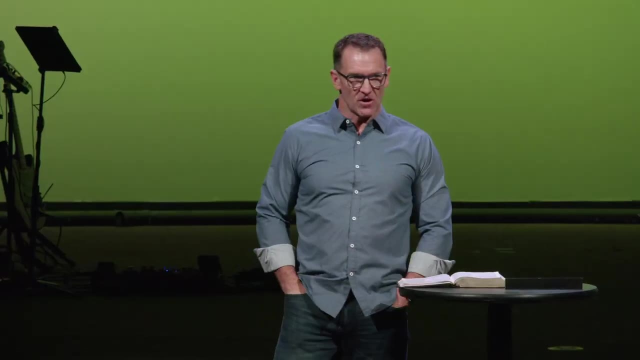 not the unity of the world, but the unity of believers in a church. But our problem is this- And this is why we're doing this series In 2020, the church- not just the world, but the church- faced an awful lot of disunity. 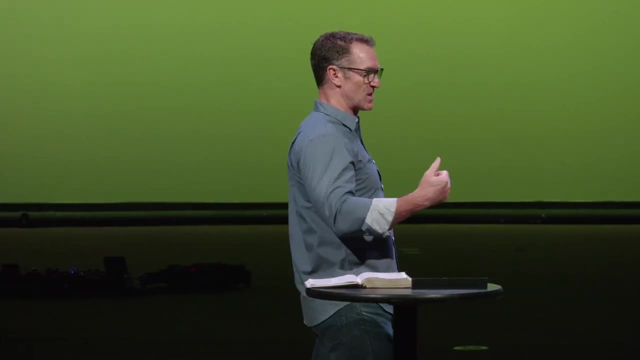 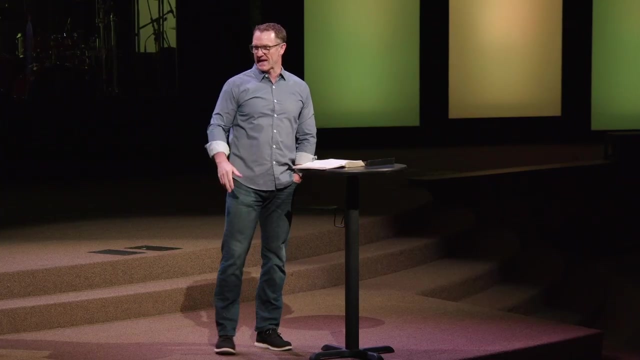 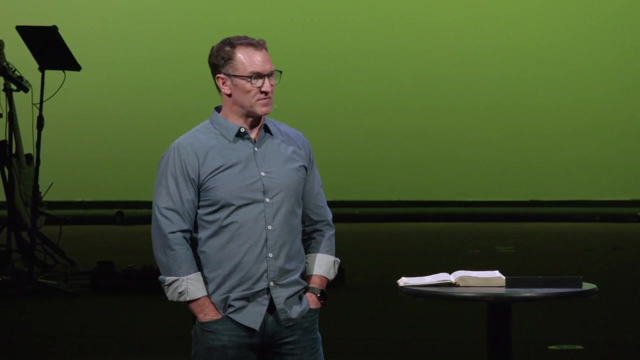 because we had that perfect storm And y'all remember it, it was COVID. It was the church's conflict with the political overreach, my opinion, that they had in making all these kinds of rules for the church. We had racial tensions like we've never seen before. 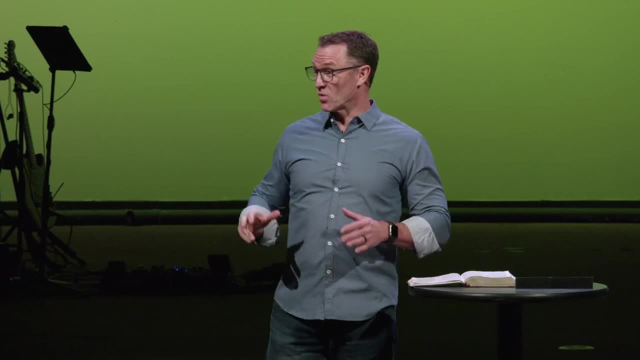 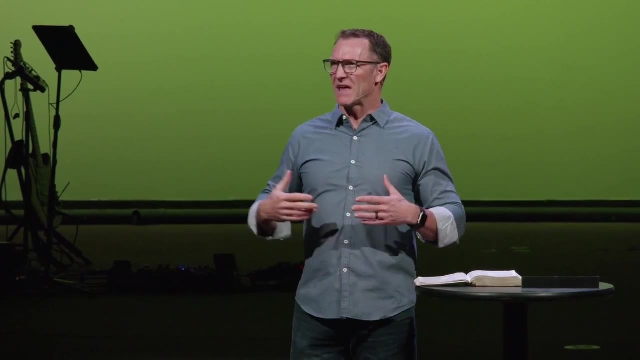 And then in that same year, we had an election and our world lost their freaking minds. But the interesting thing was, so did the church Like. people came to church and Christians couldn't agree on each other. They actually had to. Christians reshuffled the deck. 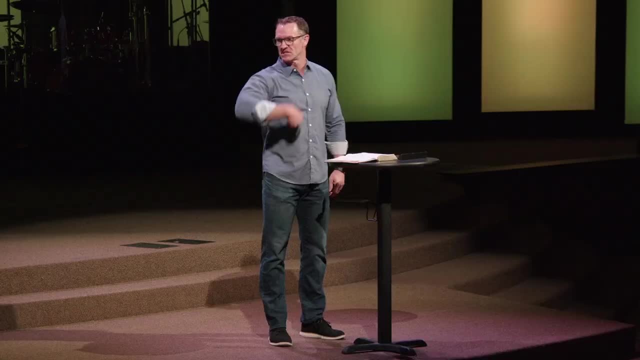 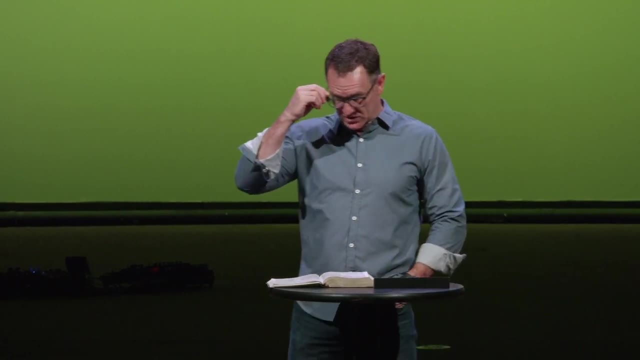 I can't go to that church because they do this, And I'm going to go to this church because they do that, And all of a sudden, people who had different beliefs about things, they could not get along with each other. And so, 2024, we're on the brink of an election. 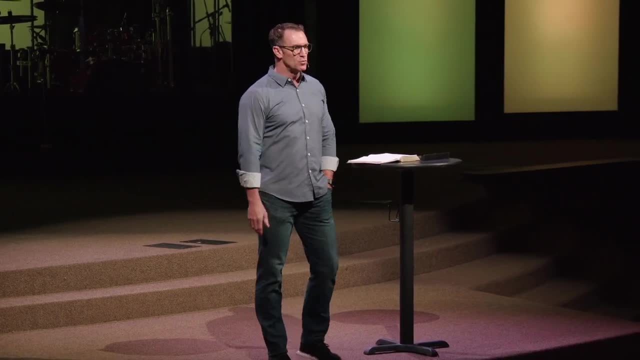 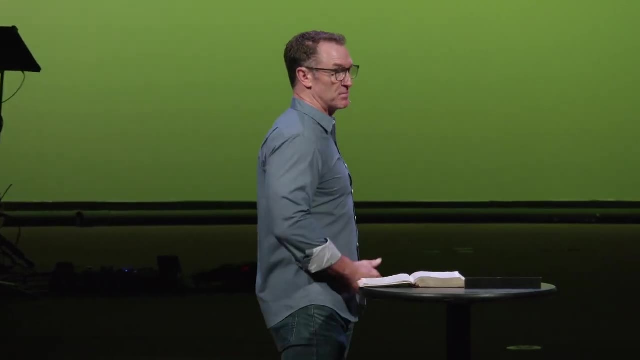 And instead of getting ununited, disunited, broken apart in conflict, instead of reacting to it, instead of reacting to an election, here's what I want to do. I just want to prepare for it So that maybe this fall, when you're tempted to go. 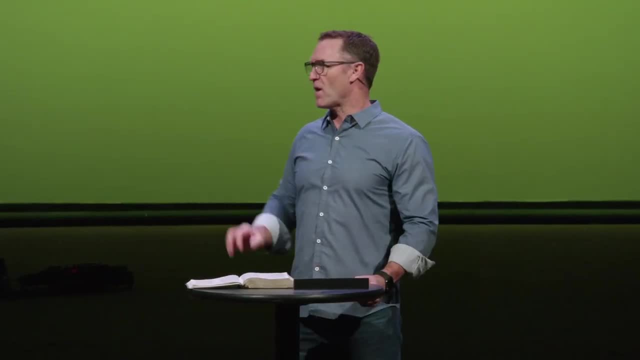 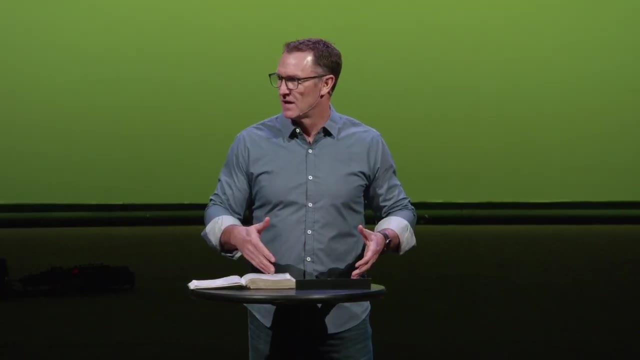 but that person and be aggressive. we might hit the pause button for just a moment and say, well, wait a minute. I know what the scripture says about unity, and the unity of believers, not just one church and the believers that gather under one roof. 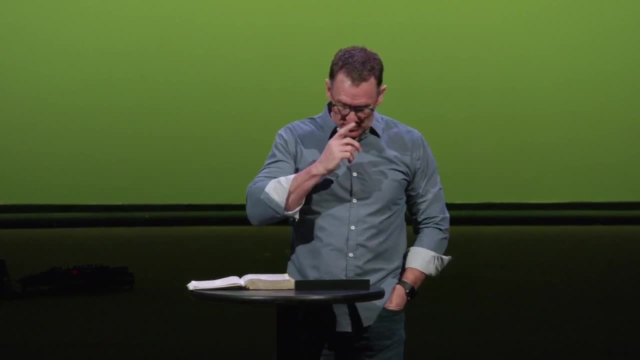 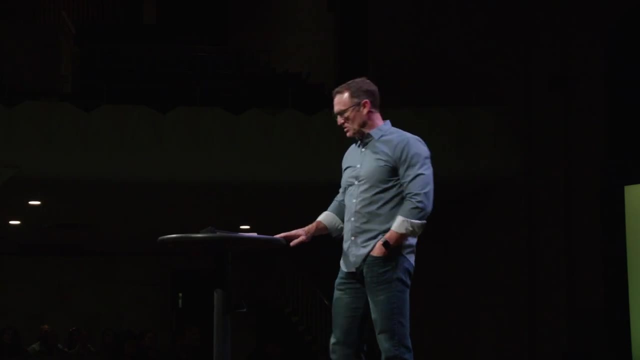 but the unity of God's whole family, And so that's why we're doing this. Last week, we discovered this: that the unity that we have as believers was actually purchased, And it was purchased by Jesus on the cross. Ephesians chapter two. 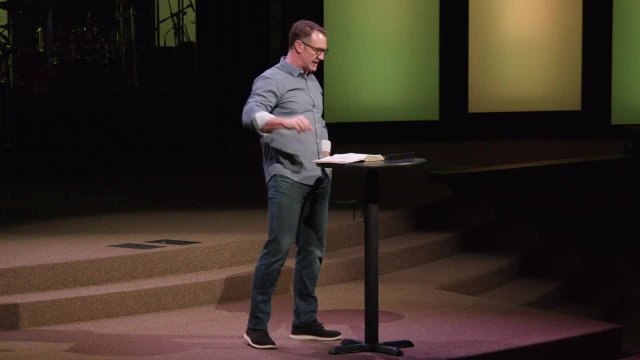 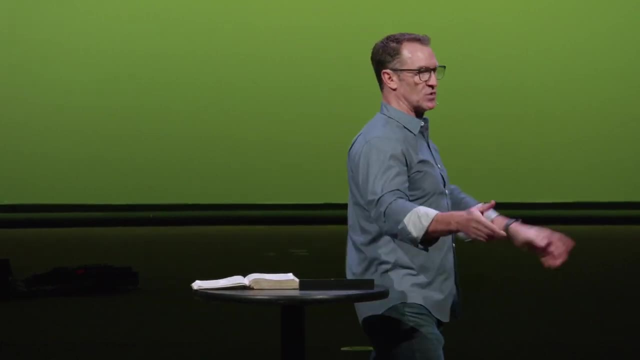 And if you've got a Bible open up to Ephesians, go to chapter four. we'll get there. today It says this: Jesus' purpose was to create in himself one new humanity out of the two, And if you remember this, there's Jews and there's Gentiles. 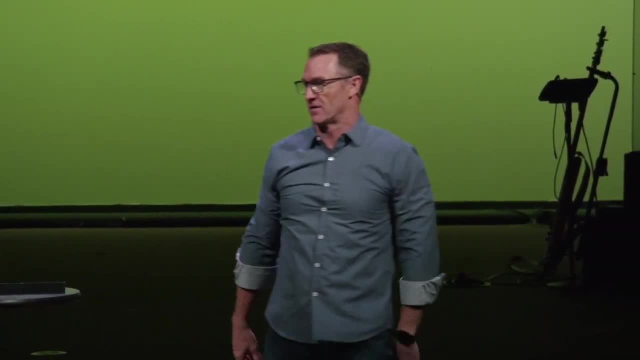 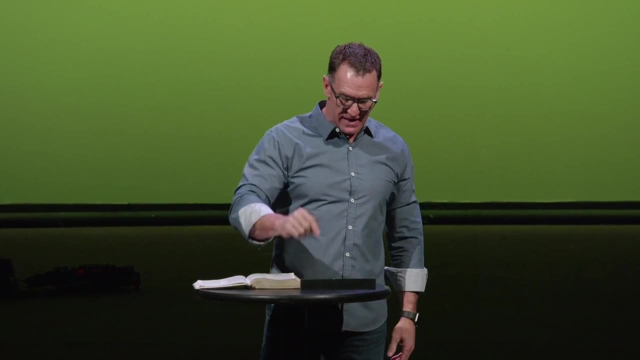 and they were raised totally different. They were raised to hate each other. Jesus is like: by my death, I'm going to create one new humanity out of these two groups Who hate each other, thus making peace and in one body to reconcile both of them to God through the cross. 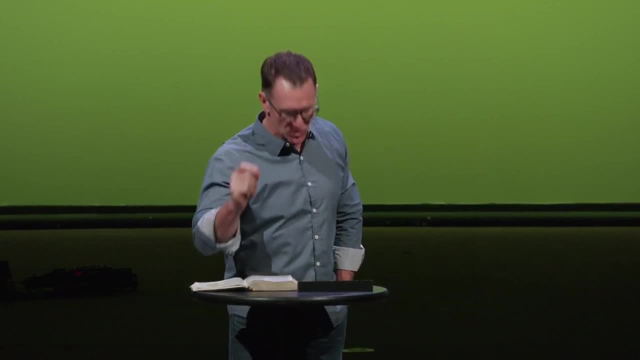 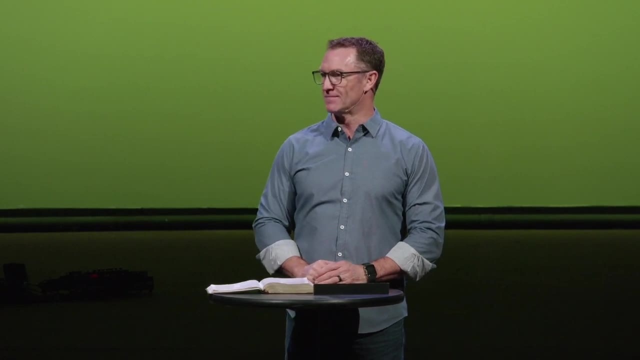 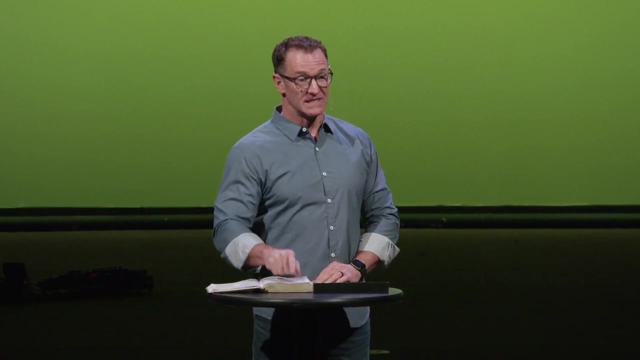 Jesus dies paying for the unity of his family. So the truth that we came to landed on was this: you and I, we can't create unity, because unity was already gifted to the church by Jesus. All we can do is in Ephesians, chapter four. 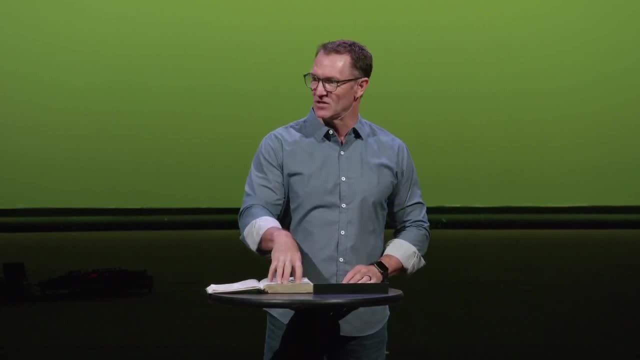 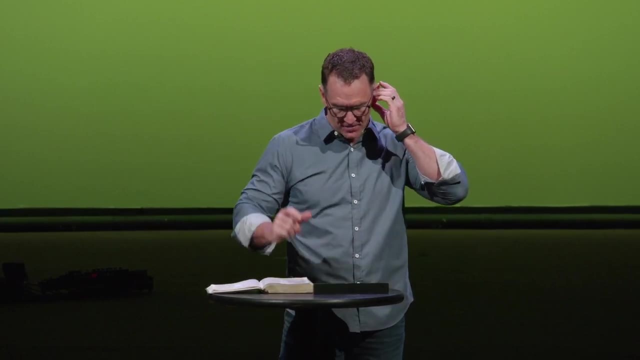 it says: I want you to do everything possible to maintain the unity. You can't create unity. We can only maintain the unity that Jesus gifted to the church. So Ephesians, chapter four, turn there. We'll all be there together. 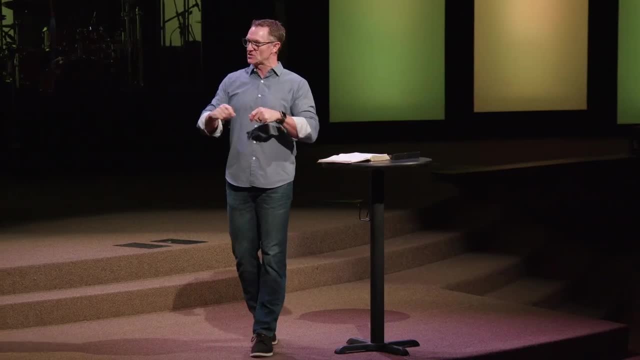 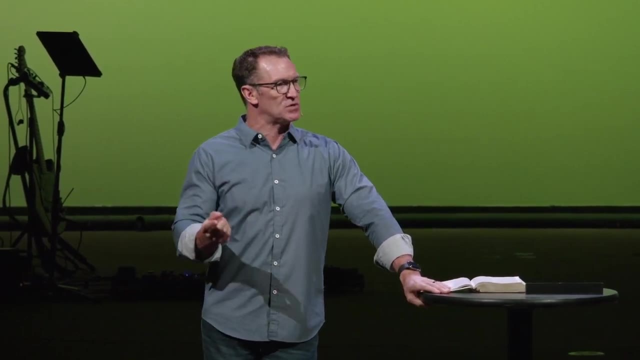 When it comes to unity, though, as you're turning there, make sure you have your notes too, because I want you to see. this Quick question, though: Was Jesus asking us to do something that he didn't do himself? What I mean by that is this: 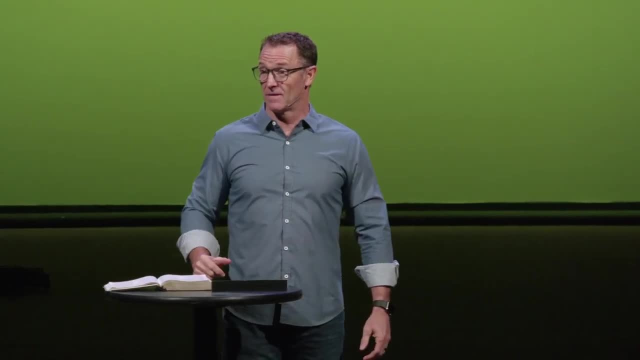 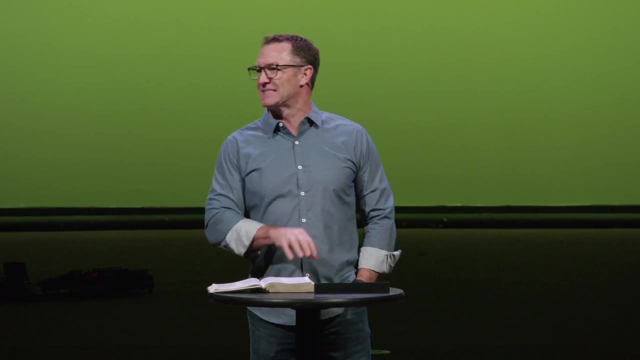 think about the 12 men who were his apostles, his disciples. Who did he gather together? One of the guys he invited to be a part of his team was this guy known as Simon the Zealot. His birth name is Simon. 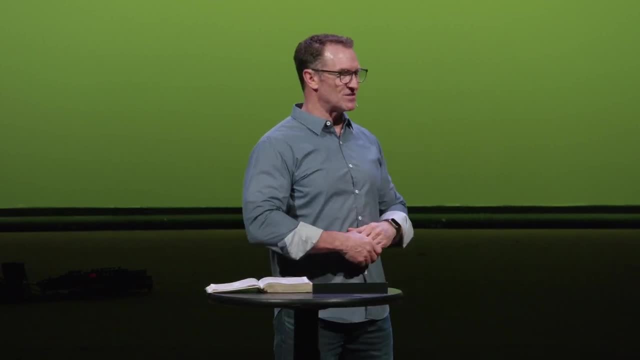 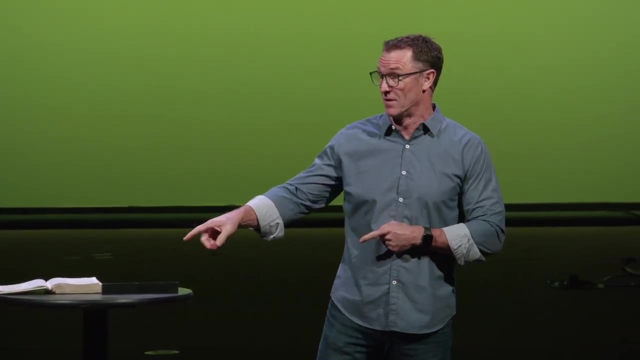 Zealot is his nickname. Some people wonder, like, why is he called Simon the Zealot? I mean, first of all, he has the nickname, So it distinguishes him from the nine other Simons in the Bible. Second, what does it mean to be a zealot? 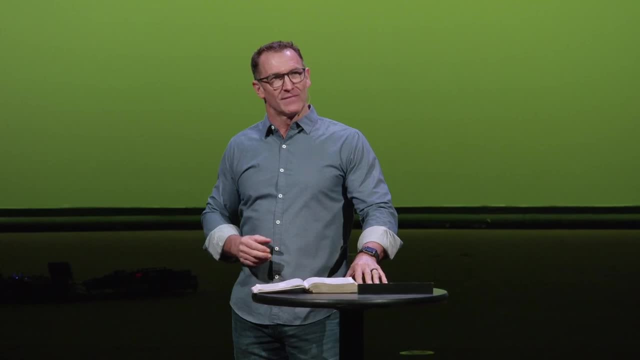 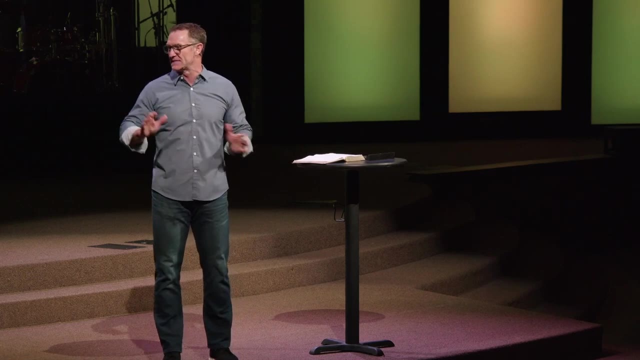 I mean, maybe he was, like I don't know, the hyperactive follower of Jesus. He was just like Jesus, Jesus, Jesus, Jesus. They're like you just quit being a zealot. So he was Simon the Zealot. 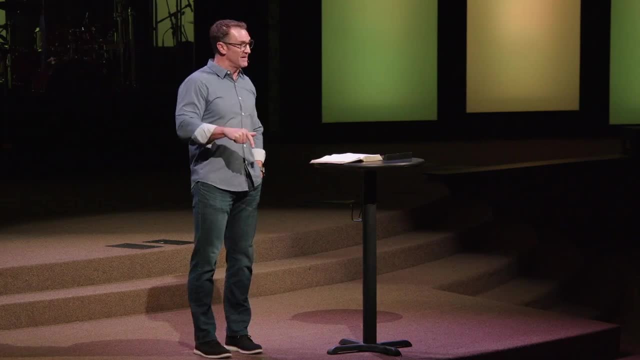 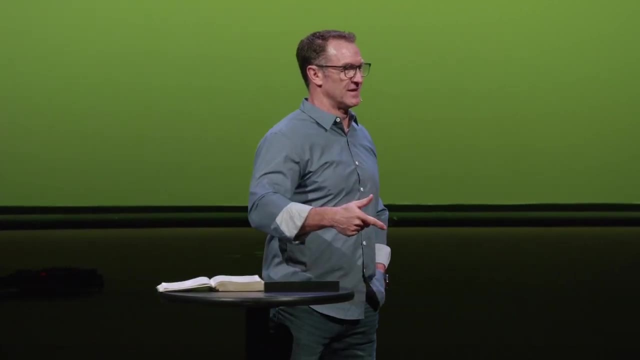 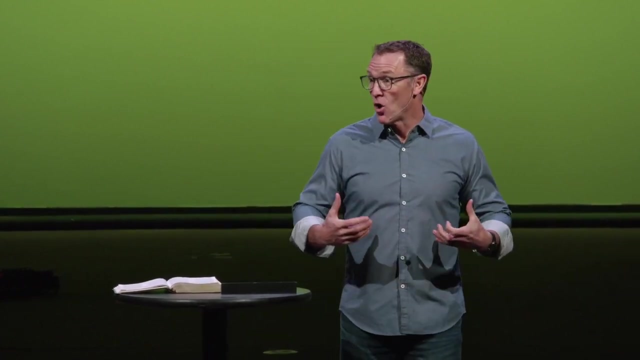 I don't know. Maybe he was really zealous for the Old Testament law. Here's what most commentators think: Simon the Zealot was actually a political designation. It was a group of Jewish people who were focused on overthrowing the Roman government through violence. 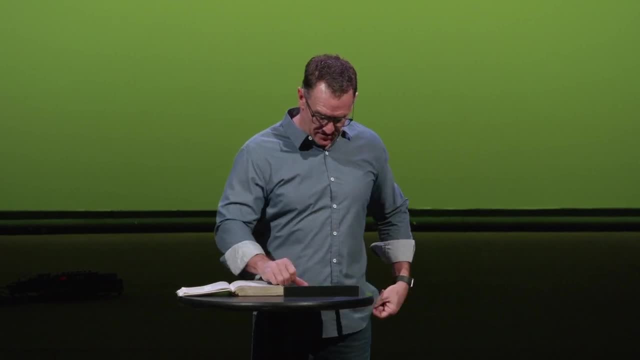 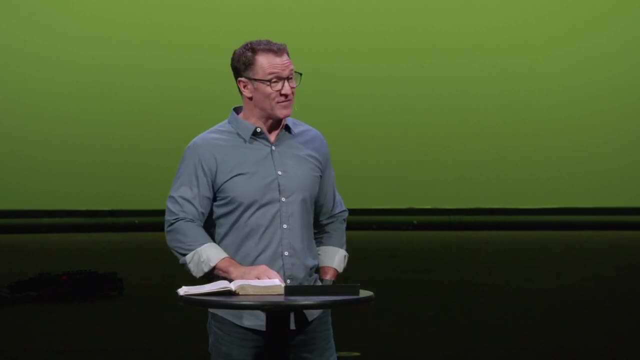 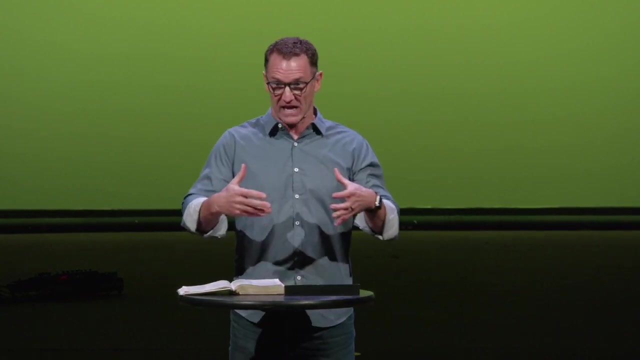 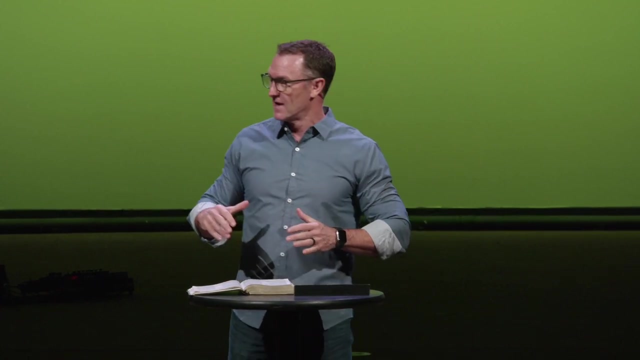 Simon would have considered himself a patriot. Simon would have been the guy who was heavily armed, ready for the revolution to overthrow his government. Are you with me on who this guy was and who he might be today? But here's the problem. Jesus recruited a guy to his team. 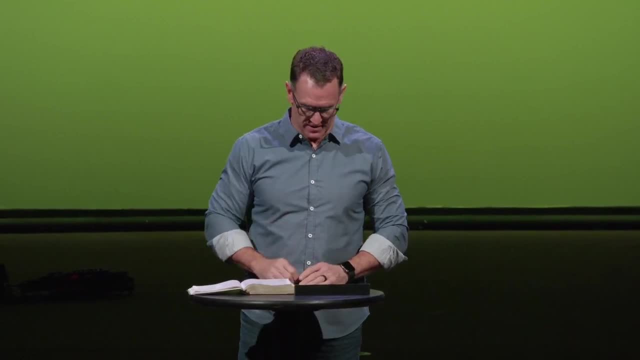 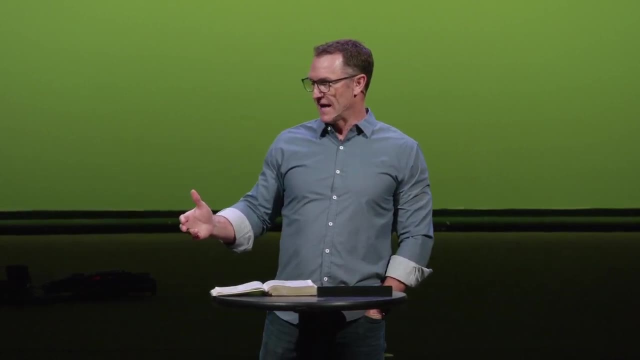 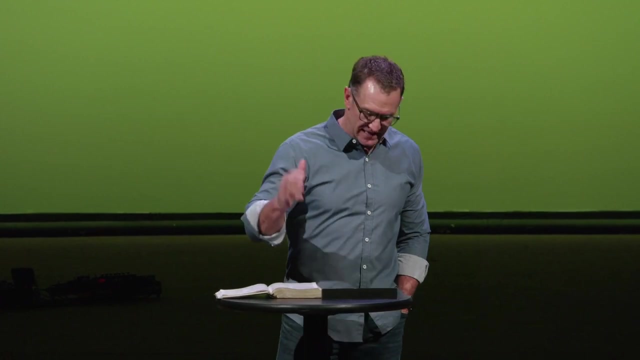 who Simon would have wanted to kill. Follow me in this. Jesus is walking from one town to another and he comes across the toll booth, And at the toll booth there's a person collecting tolls who's known as a tax collector. His name is Levi. 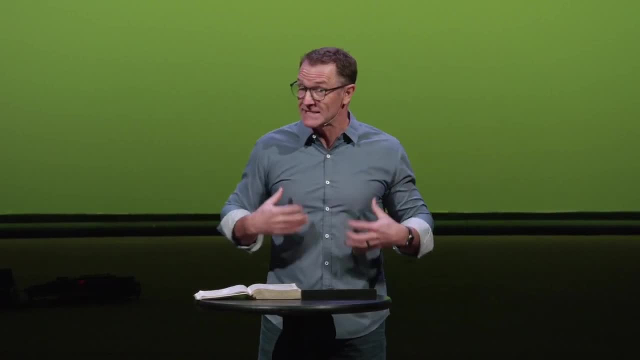 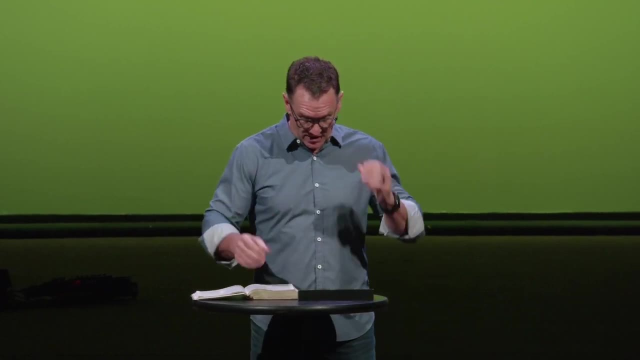 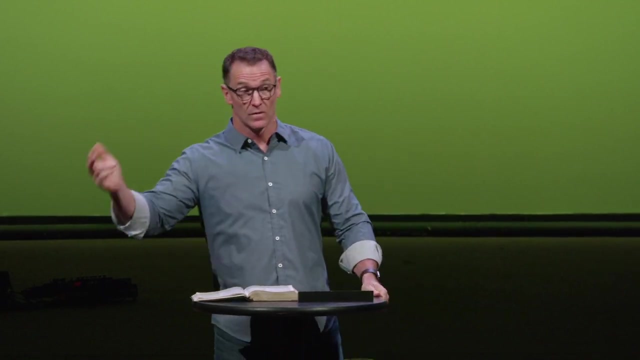 And in Luke 5, Jesus invites Levi to join his team to be one of the top 12 followers, where Simon the Zealot already belongs. Now who is Levi? Levi collecting taxes for? He's collecting taxes for Rome. 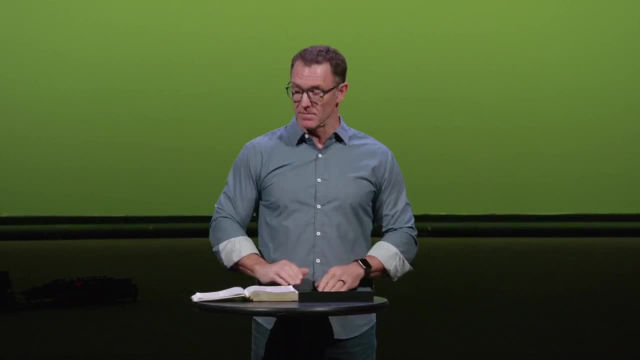 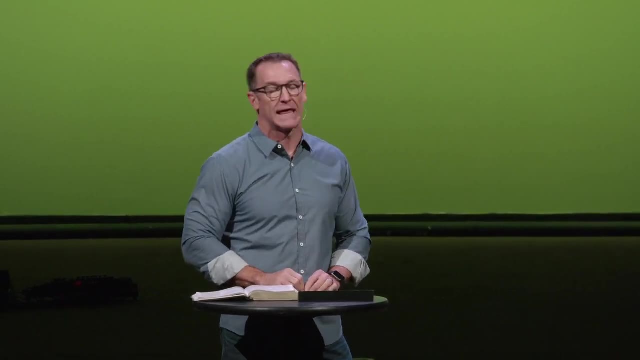 Wait a minute. So his mentality would be this: If you can't beat him, join him. The problem is, Simon the Zealot's philosophy may have been: if you can't beat him, then you got to kill him, And those two guys are now on the same team. 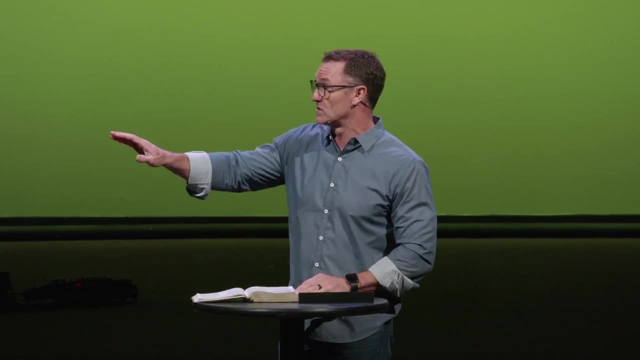 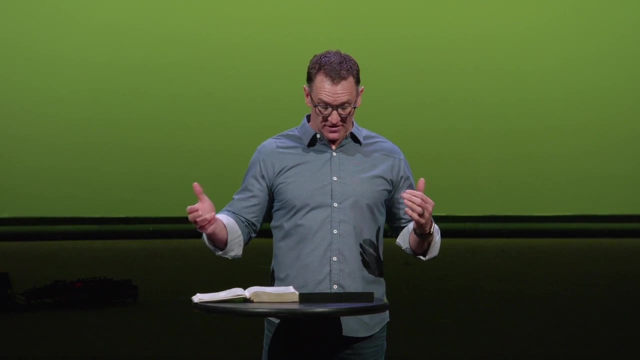 Here's how this reads: Luke 5, 29.. Don't worry, we'll get to Ephesians 4.. Then Levi held a great banquet for Jesus at his house, And a large crowd of tax collectors and others were eating with them. 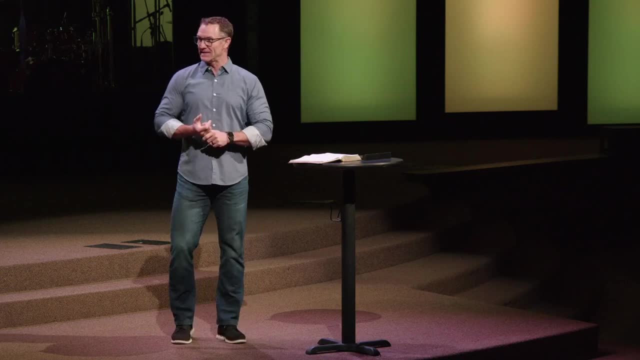 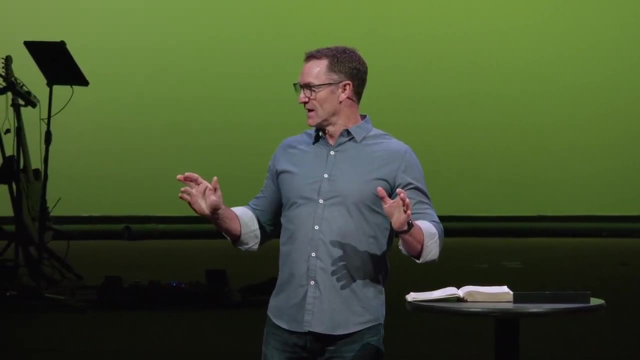 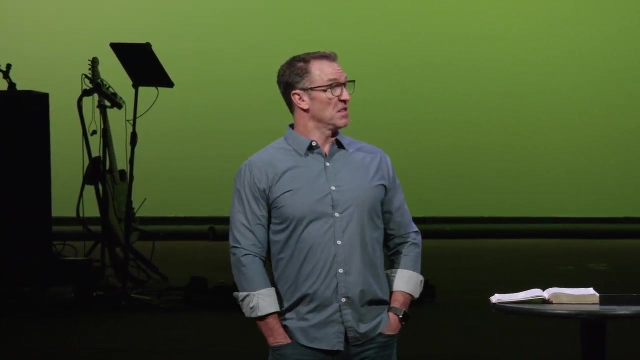 Now just imagine for a minute that Simon the Zealot walks into Levi's- also known as Matthew later Levi the Trader's- house. He walks in. he's like big house, really nice, Purchased off the backs of our countrymen. 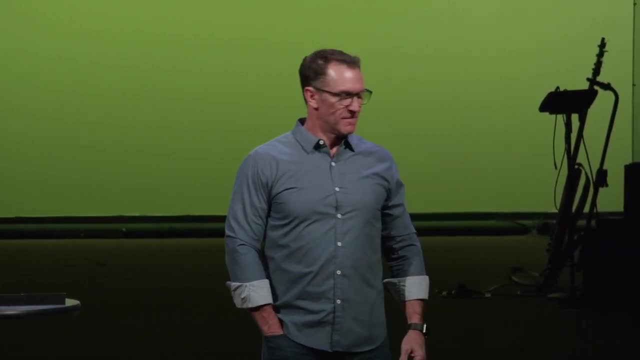 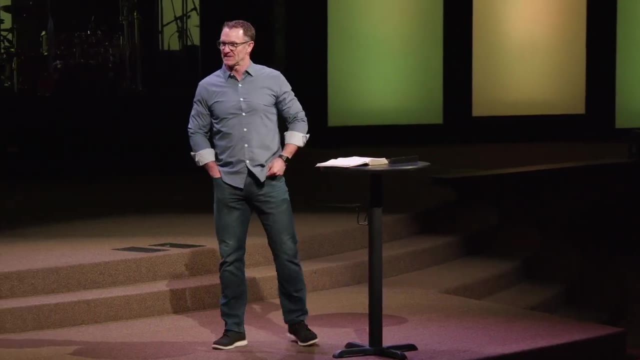 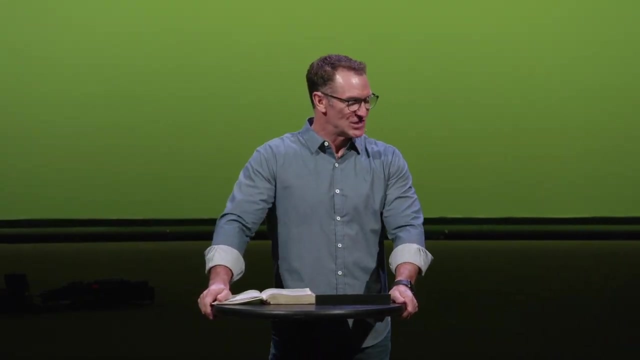 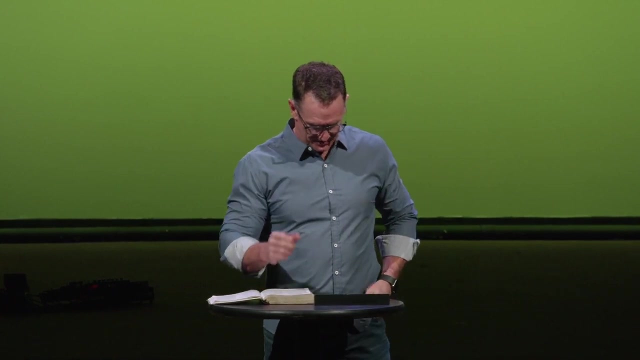 which you stole And look at this great banquet, all this food purchased by a trader who stole from us, And Simon the Patriot. the Patriot is looking around the room and it's all Levi's friends who are traders as well. Simon the Zealot probably hated most of the people. 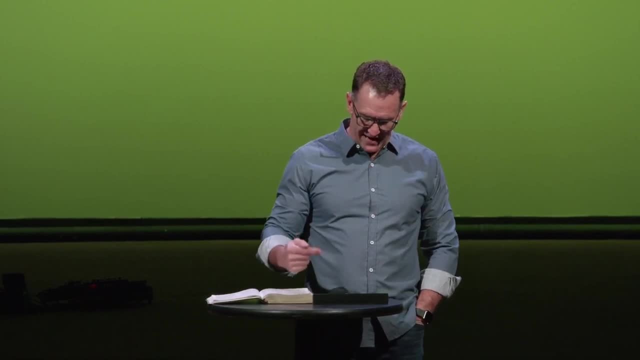 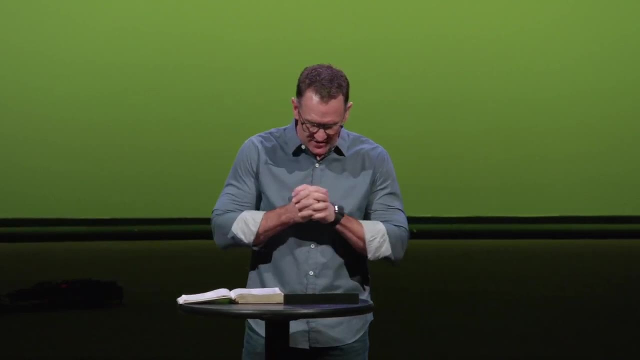 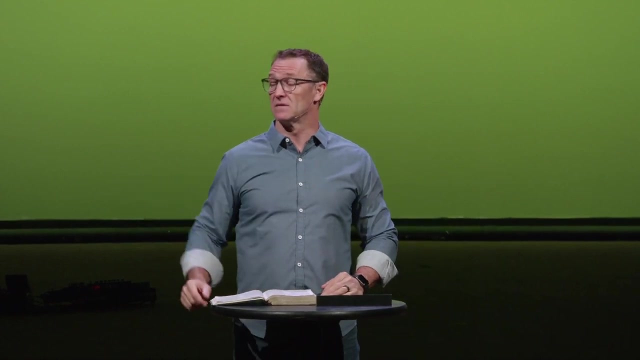 in that room And Simon had to wonder why Jesus would invite Levi. It was this group of men, Simon the Zealot, Levi the Trader, who Jesus would ask: Father, would you make these guys one May? the thing that distinguished them. 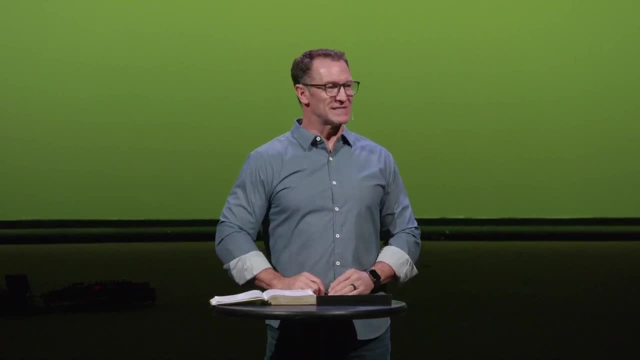 be their love for one another. See, Jesus wasn't asking us to do something that he didn't already do. He brought together two groups of people Who didn't like each other, One of whom probably wanted to kill the other, And he said: we're going to be one. 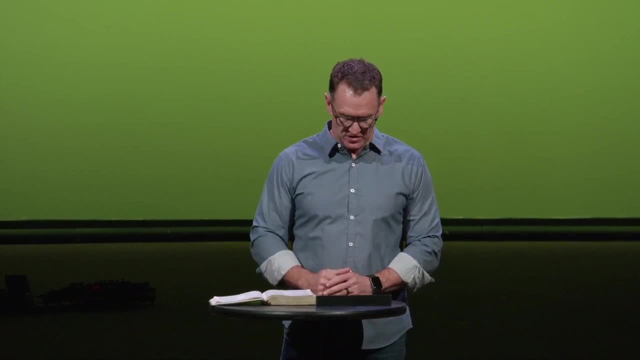 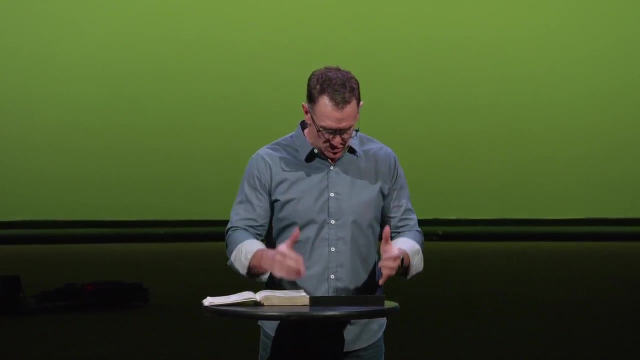 We're not going to be enemies, And the world will know that you're mine by the way that you love each other. Brings us to Ephesians, chapter six, where Paul writes this letter to the church so that there might be unity. 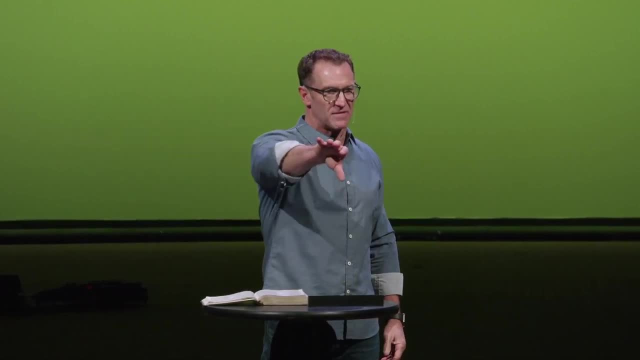 And here's what we're going to do. Chapter four: I want you to read it in your own Bible, So you see it. If you've got a paper Bible, great Should be one of the chair in front of you. You have it on your phone either way. 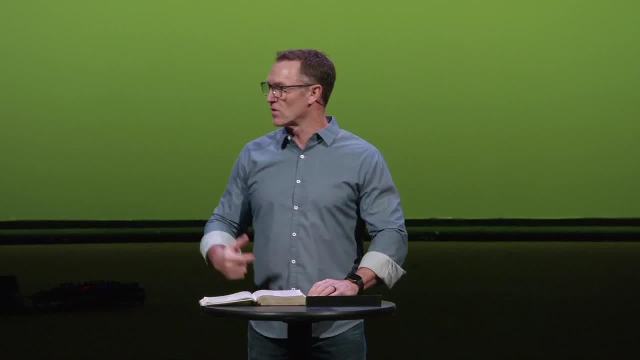 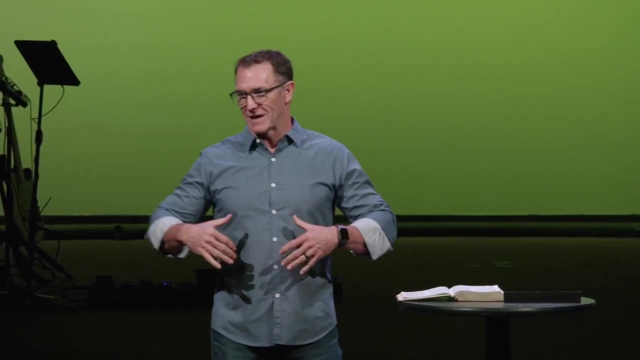 Let's just make sure we're looking at God's word because, honestly, God's word is our authority. This is what's going to drive us. You're not going to hear the pastor's opinion this morning. You're not going to hear what the most I don't know. 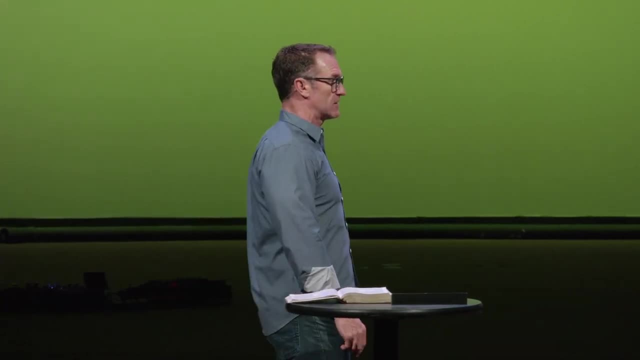 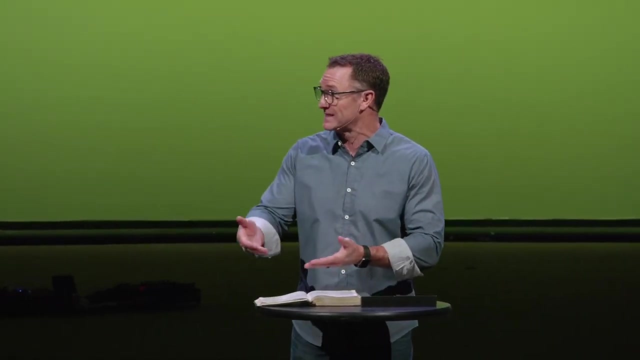 the trendiest thing is out there in the church today, Or you're definitely not going to hear the trendiest thing in politics today, or Christian politics or nationalism. You're not going to hear any of that. We're going to center this message on God's word. 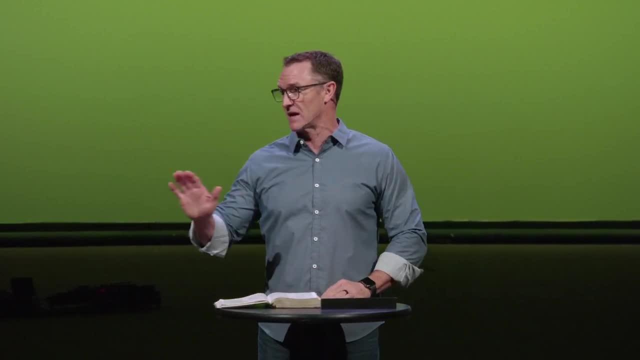 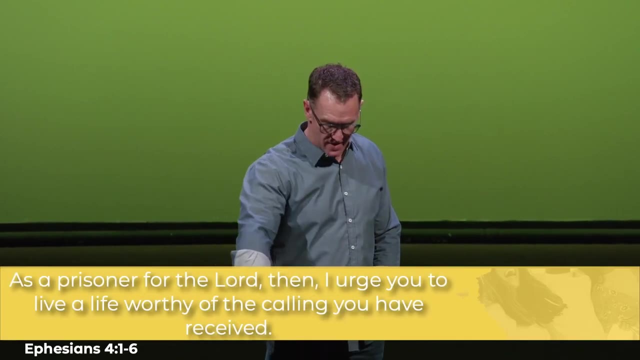 because that's the authority in our life And it stands high above everything else. It reads this way: As a prisoner for the Lord, he's writing from prison in Rome. Then I urge you to live a life worthy of the calling you've received. 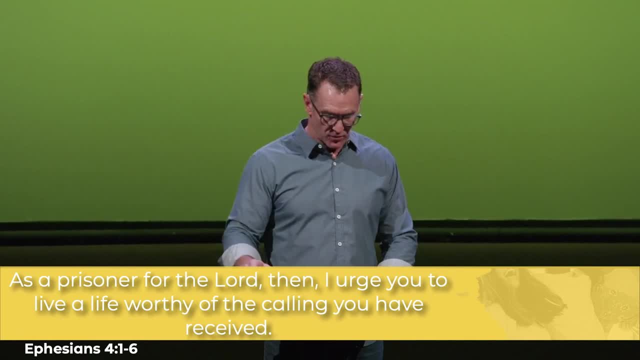 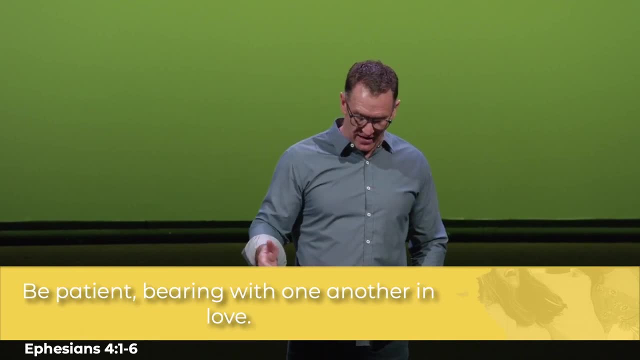 Your followers of Jesus. right He's writing to his church in Ephesus. Here's how you live a life worthy of the calling you received. Verse two: be completely humble and gentle. Be patient, bearing with one another in love. Make every effort to maintain the unity of the spirit. 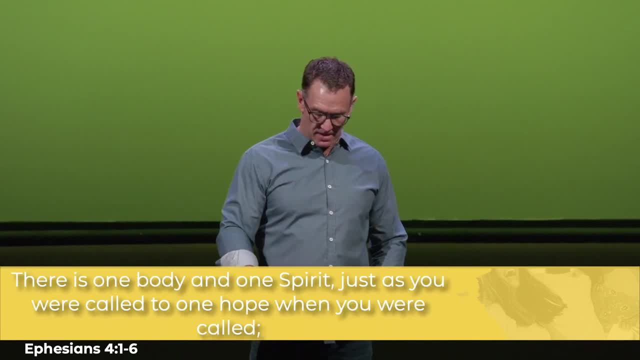 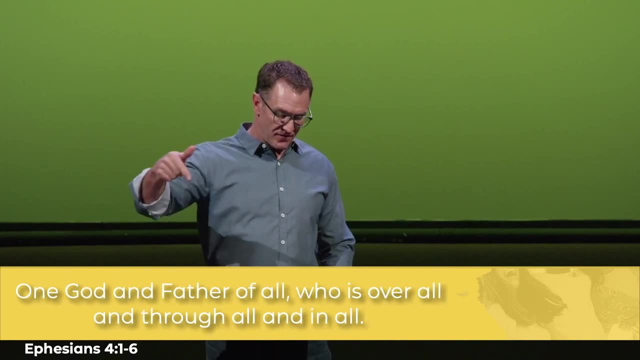 through the bond of peace. There is one body and one spirit, Just as you were called to one hope when you were called one Lord, one faith, one baptism, one God and father of all, who is over all And through all and in all. 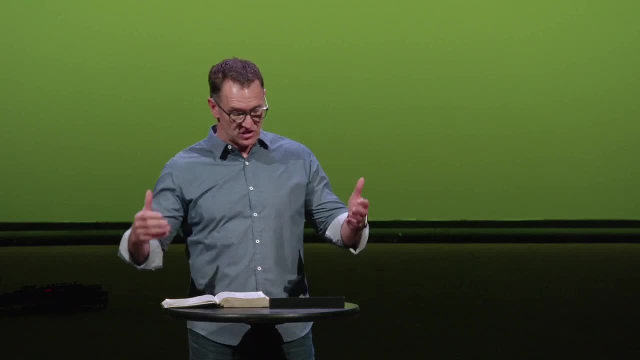 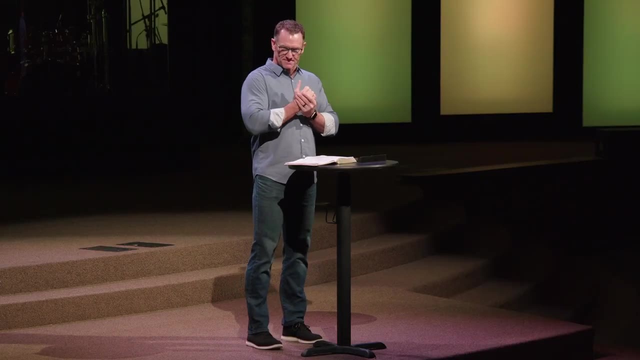 So we're going to try and understand these verses today. How do we maintain this unity that Jesus purchased on the cross? I want to think about it in this terms: okay, I want you to think about walls and I want you to think about bridges. 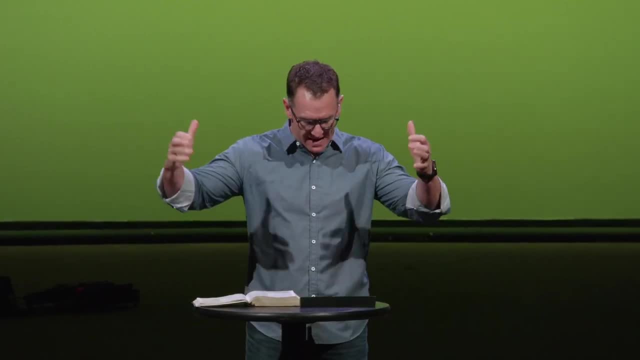 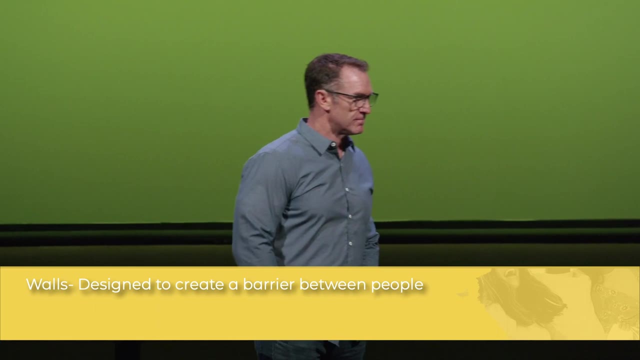 They each have a purpose. Walls are designed to create barriers between people. Walls keep your kids from running in your bedroom. Walls keep people out while you're going to the bathroom. Right Walls distinguish on my street what belongs to me and my family. 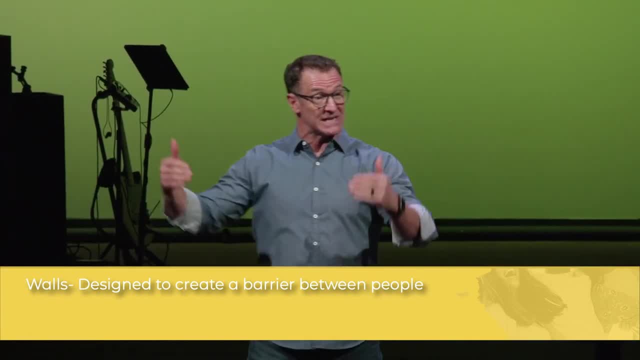 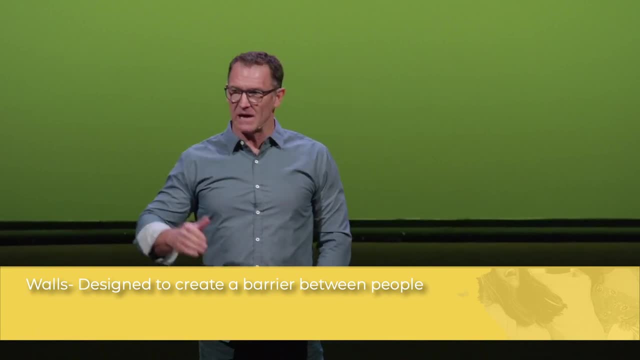 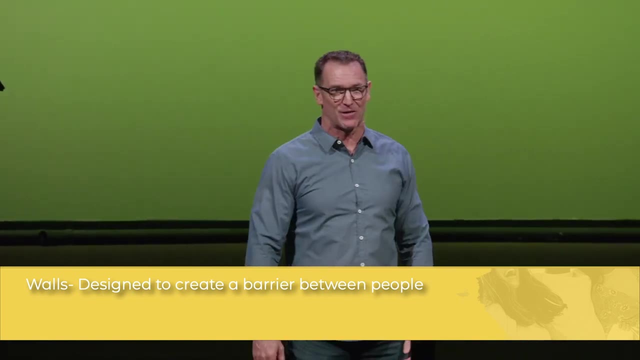 And it creates barriers so that my neighbors don't think that my space is their space. right, Walls are good, Can be good. Walls actually keep bad people out. Walls also keep bad people confined to a place where they can't hurt other people. 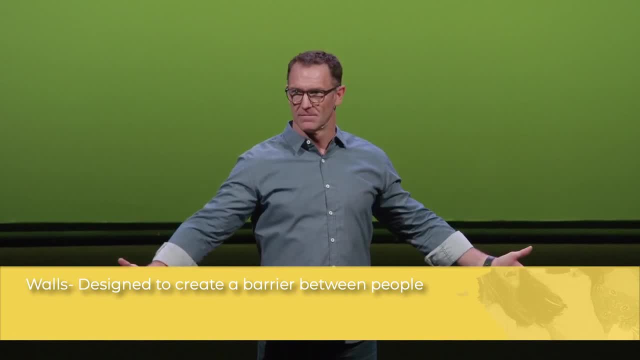 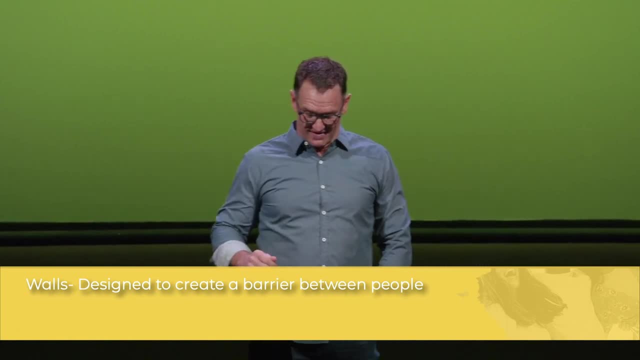 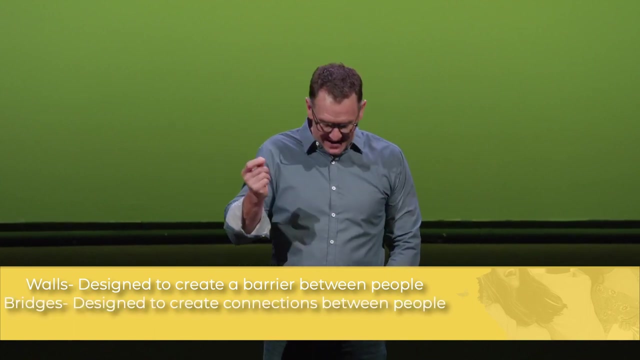 We all love walls, don't we? You should start nodding, If not, open your front door and let whoever you want come on. in Bridges, though, think about the design of a bridge. They're actually designed to create connections between people where natural barriers exist. 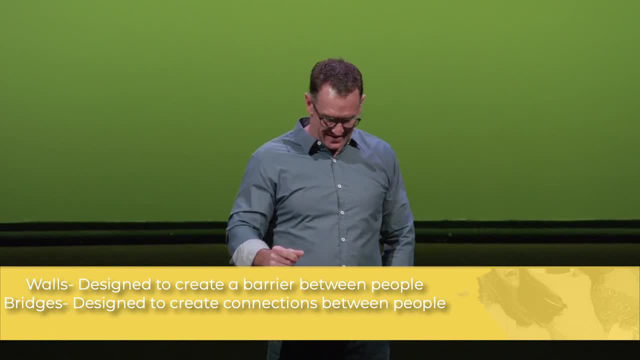 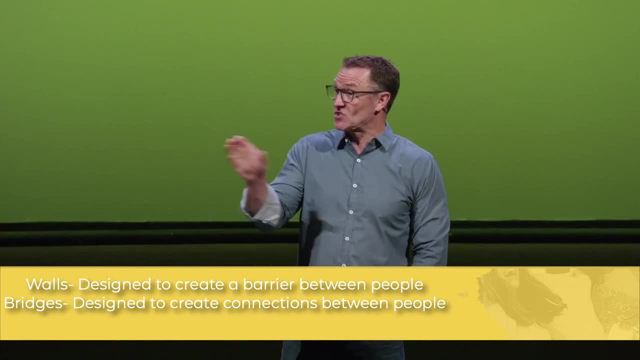 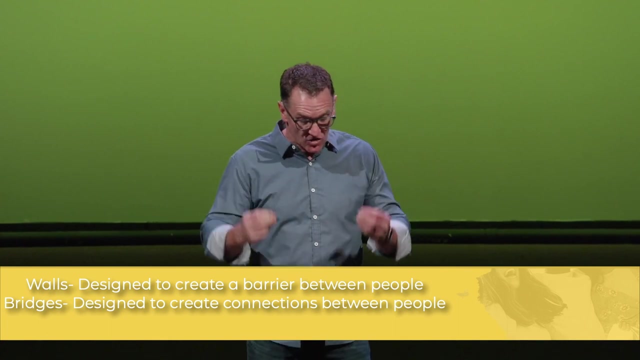 Where do you build a bridge? Over canyons, Over rivers, Over streams? A gully, Sometimes, where there's a dangerous street crossing, you would build a bridge so that people could cross Any place that is dangerous or difficult to cross. 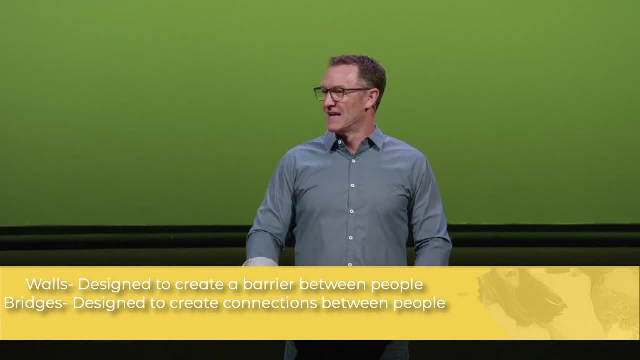 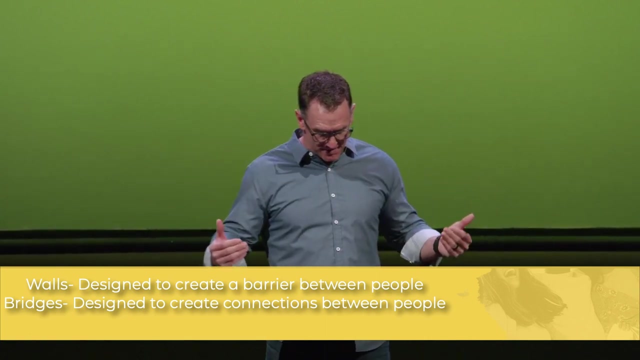 is a good location for a bridge. It's so people cannot just get from one side to the other. It connects locations, but it actually also connects people who have a natural barrier between them, preventing them from from connections. So bridges, I will admit this though. 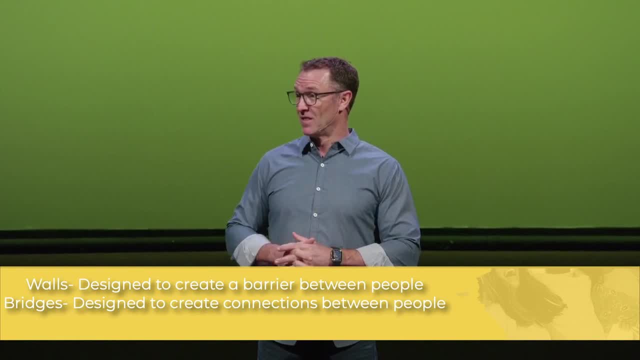 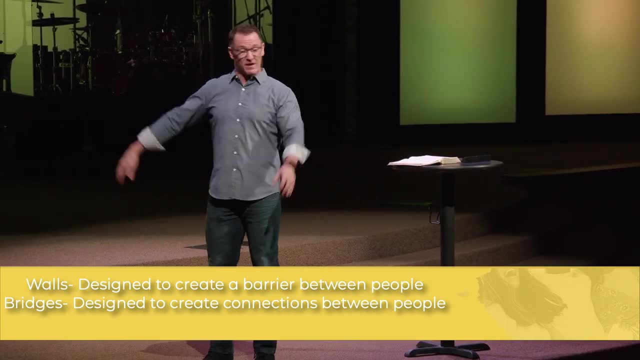 Bridges are way more difficult to build than walls are. I mean it's a wall, right. I mean you got a firm foundation for something You've got. you can just start stacking. I mean you can create a wall out of almost anything, right. 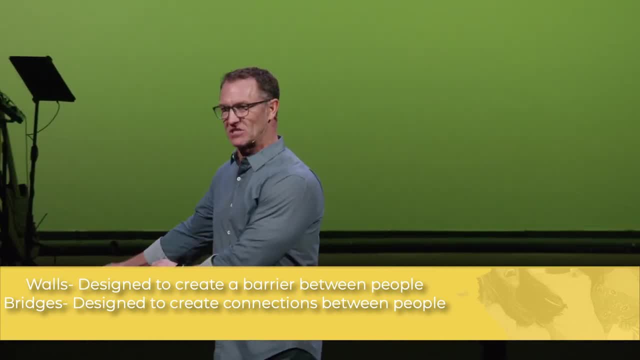 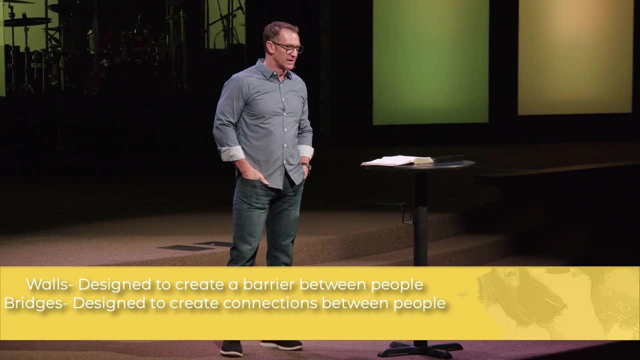 I mean, you've seen stacked stone walls. You don't even like have to mortar them in. You start stacking stones on each other. You can create a wall out of that. You ever try to make a stacked stone bridge. They're harder. 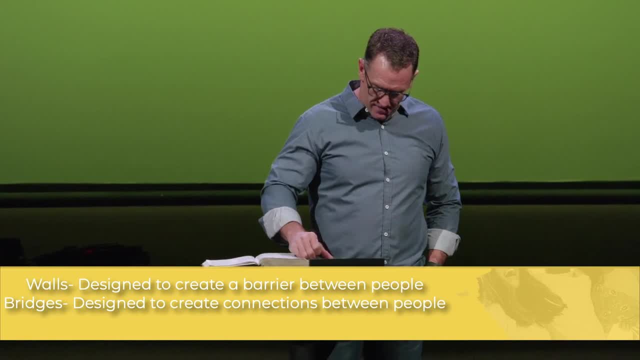 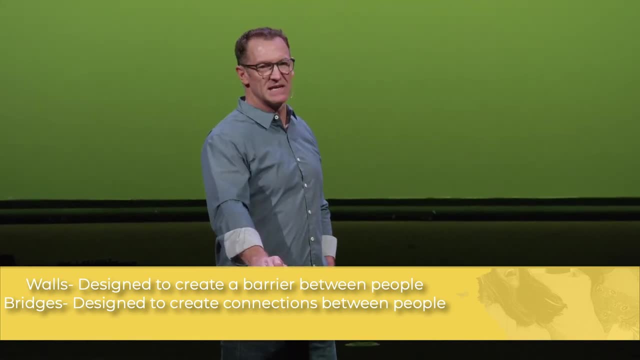 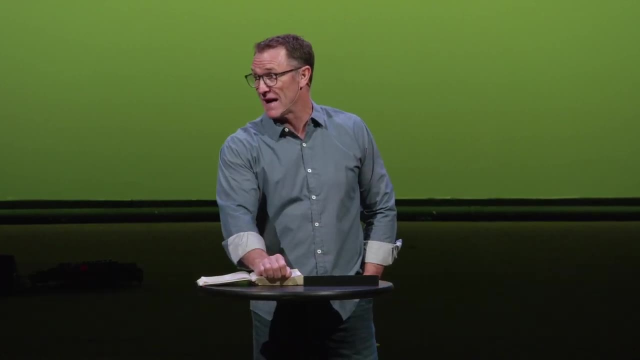 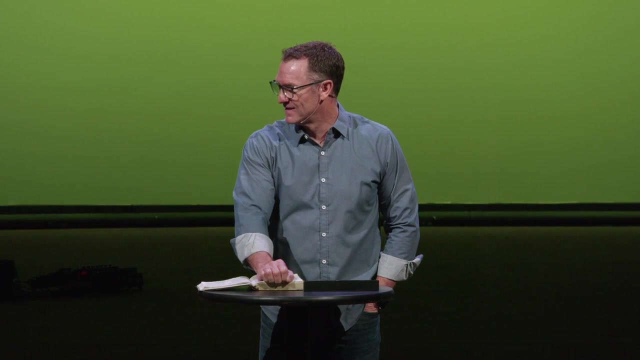 To build than walls. One of the things that we sometimes falsely believe is this: Love is easy and unity is natural. It's just not If you actually read the Bible. love is hard, It's difficult And unity is unnatural because we focus on what is different. 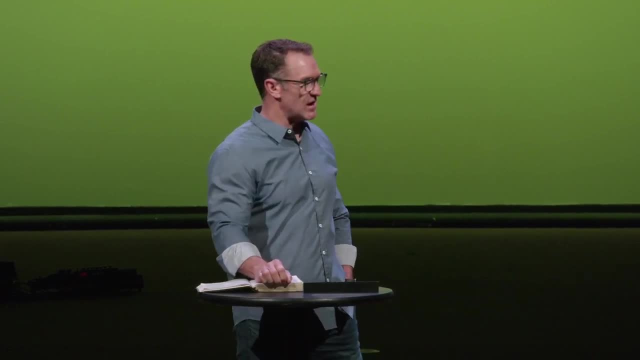 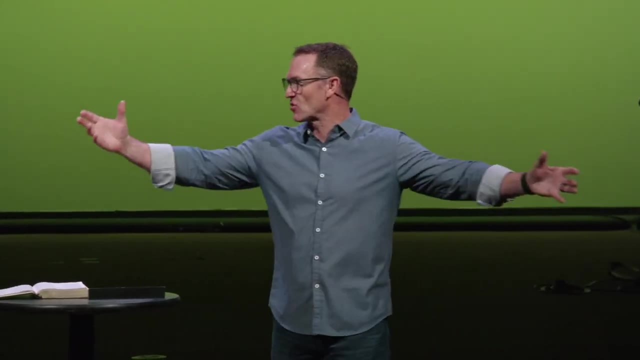 as opposed to what is natural. Unity is what unites us, So here's how I want to do this. I want to focus on this: How do you build a bridge? How do you build a bridge from one person to another, Not just across a canyon or a gully or a stream or a river? 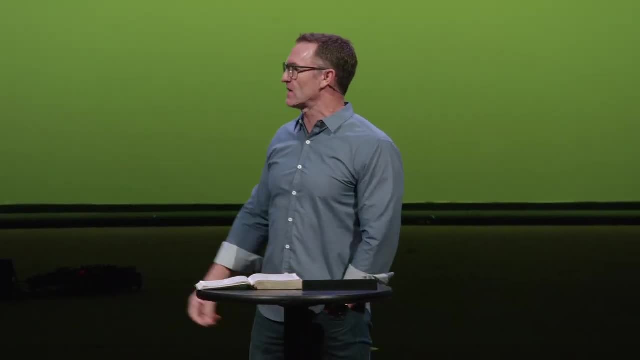 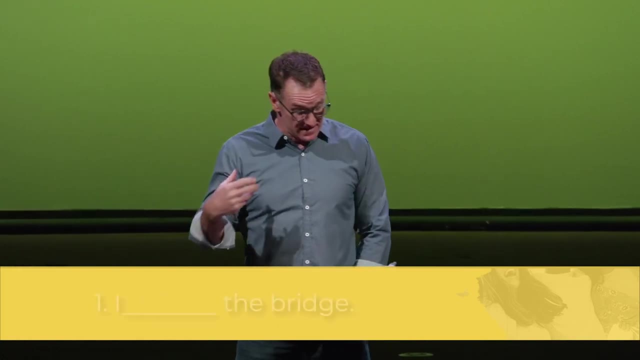 but how do you build a bridge between people? So a couple of things in your notes here. The first is this: you have to imagine the bridge, You have to build it in your mind. by this, We have to first agree that unity matters. 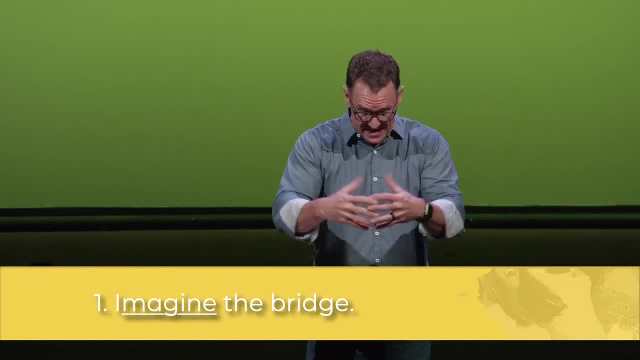 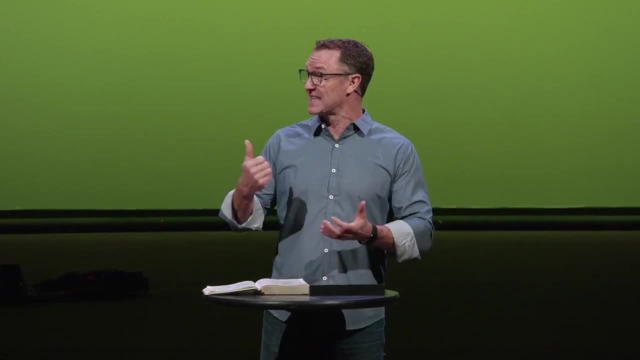 Jesus calls us to it. It's not an option that we're designed to connect And there is no plan B. Do we agree that bridges need to be built? Do we believe that Jesus has given us the gift of unity? That much of that was discussed last week. 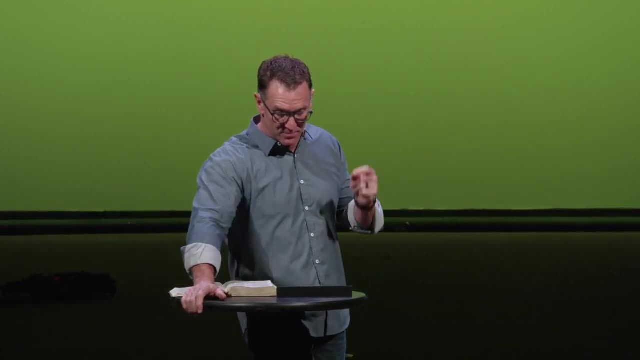 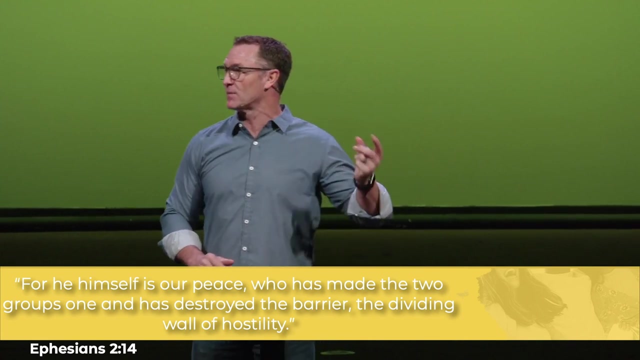 when we came across this, we covered this, For he himself is our peace. who's made the two groups one has destroyed the barrier, the dividing wall of hostility. You got to build the bridge in your mind. I think it's this. 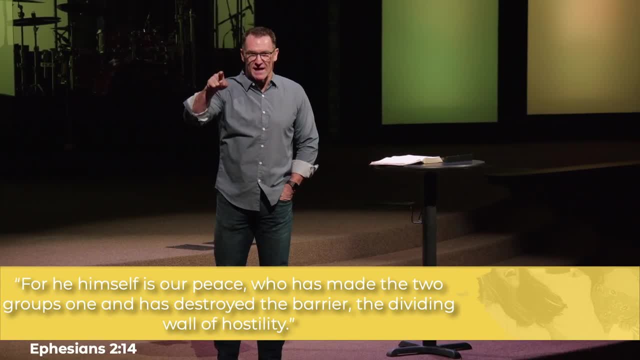 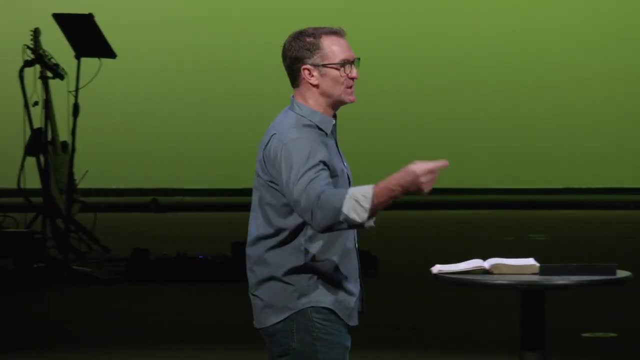 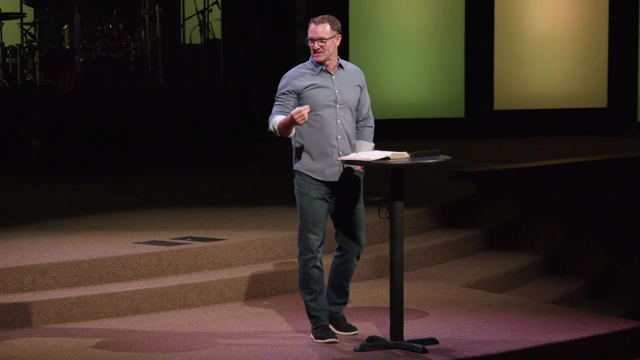 Are you convinced that you, as a follower of Jesus, must build connections with people, That you have to maintain this unity of relationship, First of all with the people in this room? some of you need to have a different mindset because, honestly and by the way, if you're new, 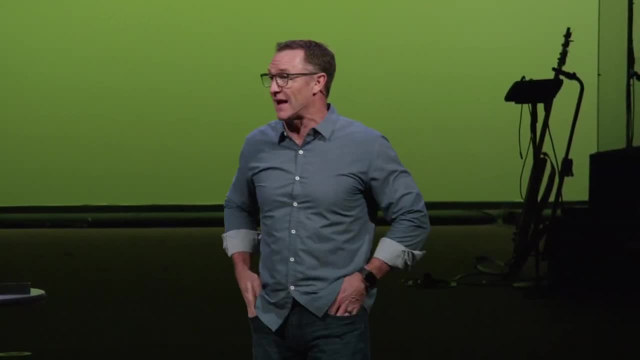 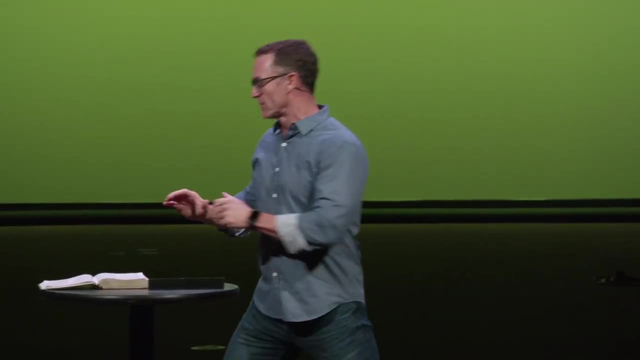 like there's a progression to this. I realize you came in today and you might be like I'm just seeing if the people here are weird. If we ever want to come back, like welcome. Yeah, there's weird people here, So you should feel right at home. 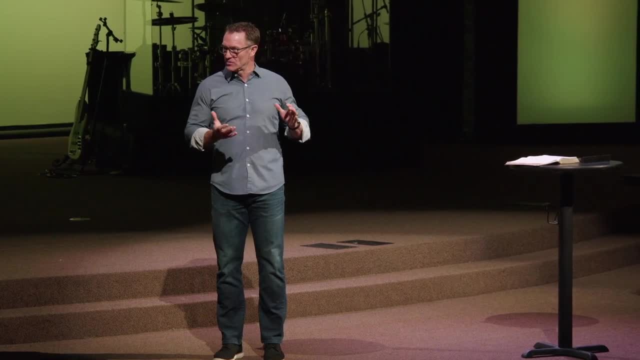 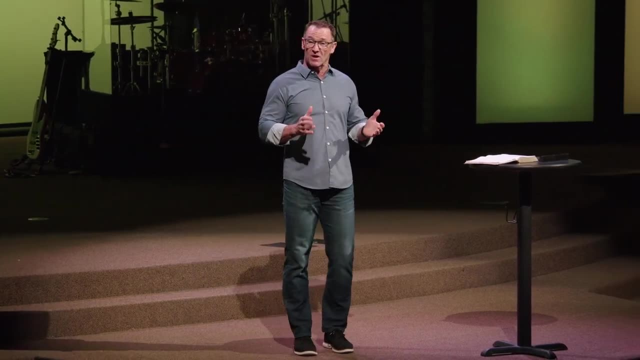 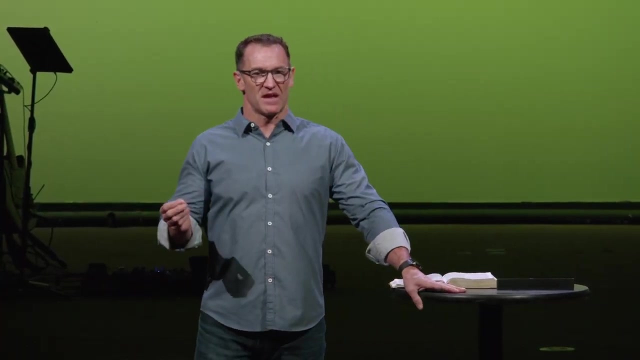 Get to know us. It's going to take a while for you to move from isolation to community, But here's the problem. Some of us have been around for a long time and we're super comfortable with our isolation. because- here's the deal- walls are safe. 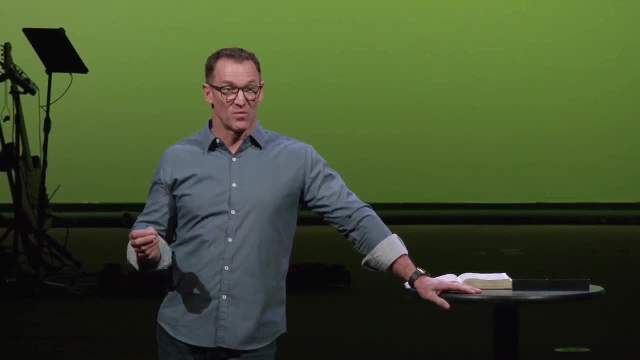 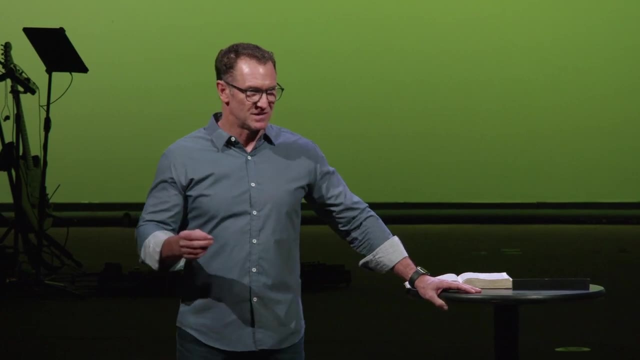 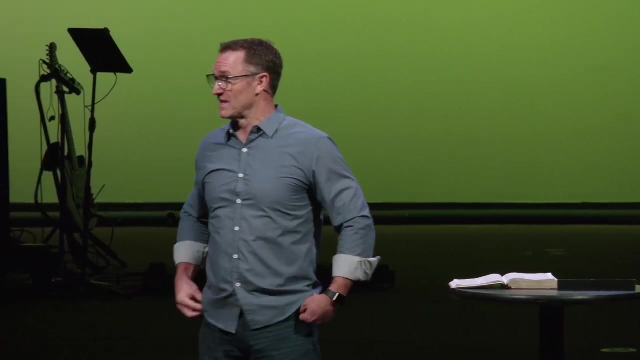 Bridges are dangerous. We found this out a couple of weeks ago, right, Because bridges can collapse under the wrong pressure, the tension, a collision that can happen and bridges collapse, And we found out a couple of weeks ago that people perished in that. 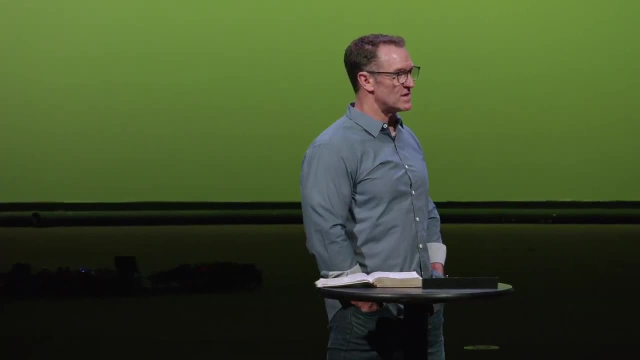 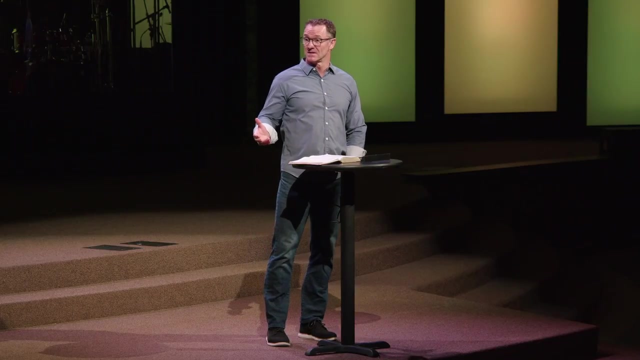 Walls, listen. walls are comfortable and walls are safe. But in this church, in God's family, God wants bridges, not just walls, And so Paul writes this: I urge you to live a life worthy of the calling you've received. 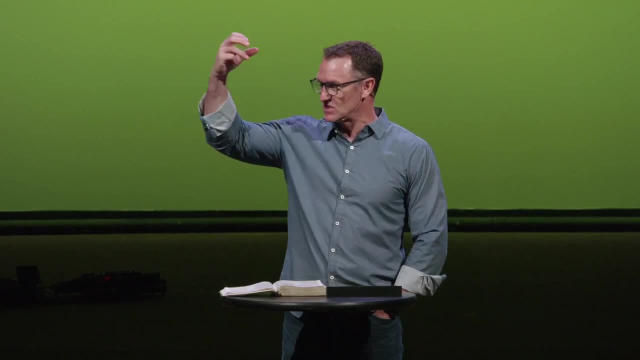 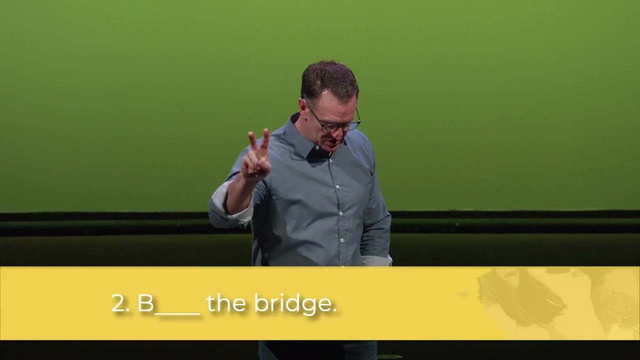 So once you imagine this, you have the conviction this is the right thing to do. I'm going to build a bridge. Question: what will it cost you? If you're going to build the bridge number two, here's what it will cost you. 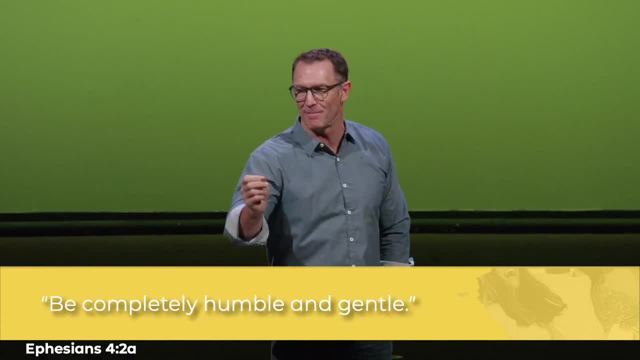 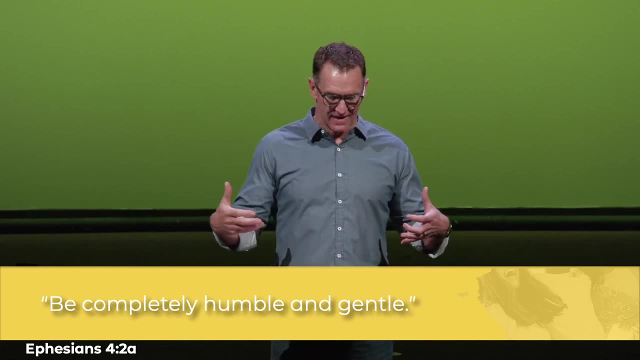 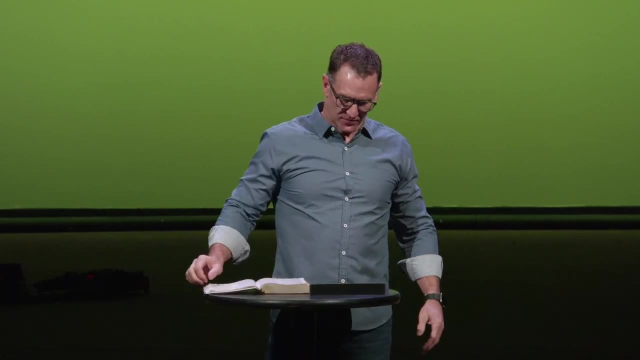 The raw materials of be completely humble and gentle, What it costs Jesus for unity, What cost him his life on the cross. He died paying for the sins of both groups so they wouldn't hold their sins against each other. What does humility look like? 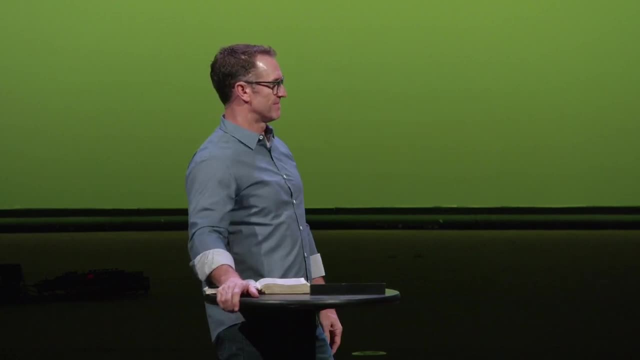 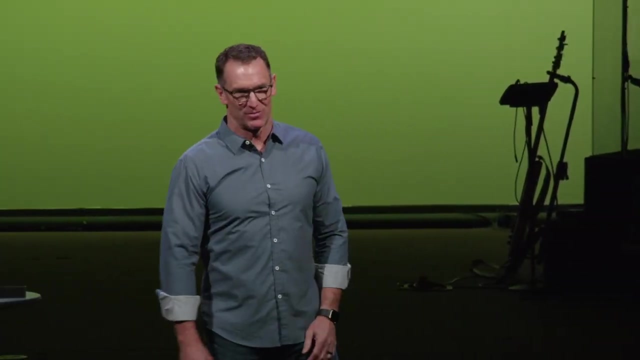 Humility says this: you first, Not me first. I don't mean like, hey, you have to make the first move to come to me and then I'll come. That's not humility, That's arrogance and selfishness. Complete humility is this. I want to put your needs first. Hey, I want to care for you. I want to consider who you are, what you need, maybe what hurt you, what makes you tick, And I want you to feel safe. I want to help you feel loved. 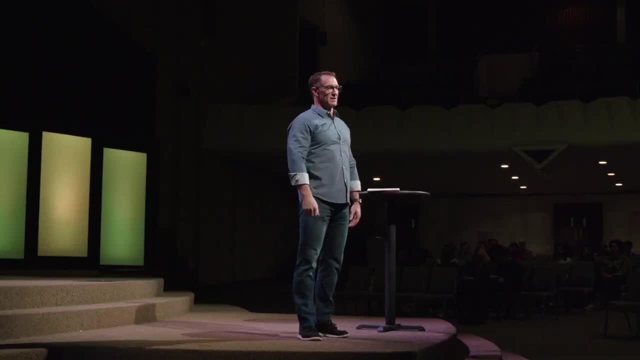 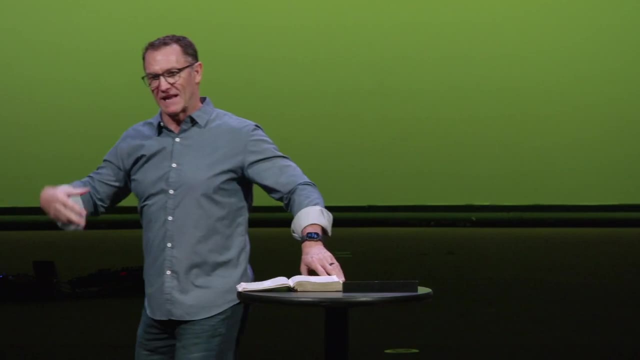 I want to help you feel encouraged you first, Which means I take my needs and I put them on the back shelf for just a little bit, With the hope that, in their trust that we've built with each other, they will look at me and say: 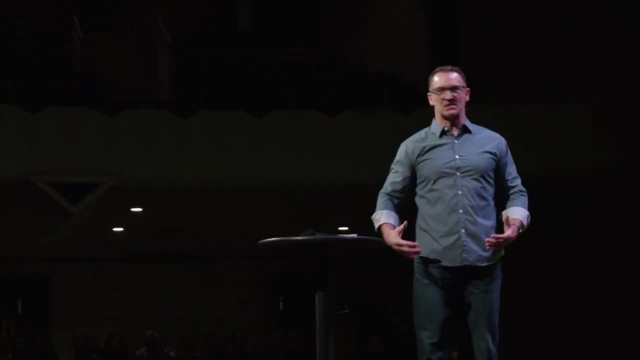 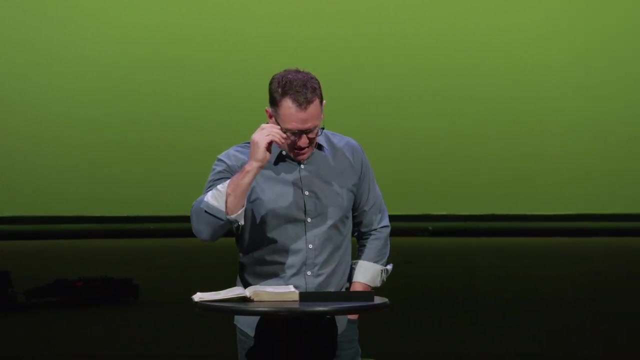 tell me about you- who are you, What are your needs, What are your hurts, What's your story- So that we can actually connect. It's not a one-way connection, but a two-way connection. Here's what's so interesting. 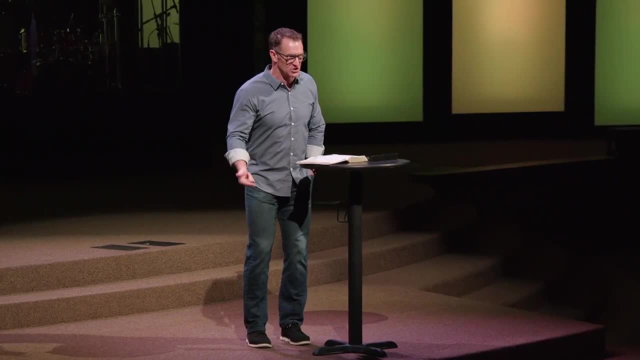 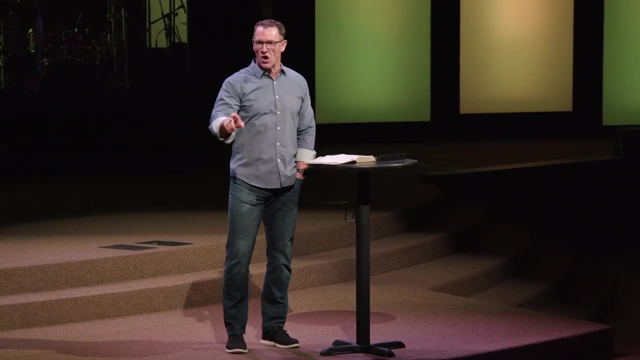 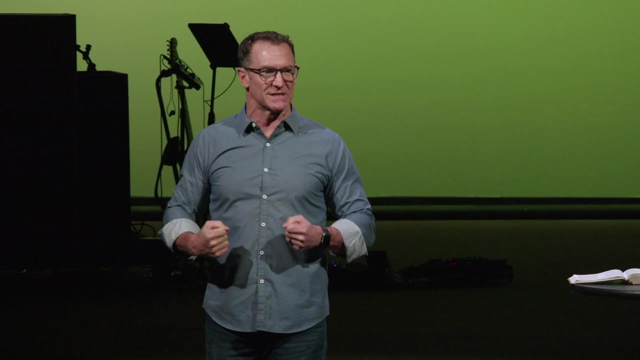 In Roman times, humility was not a virtue. Did you know this? In the world, humility was never a virtue. It was always a weakness, because humility allowed someone else to take advantage of you. And the real virtue in the world was this. 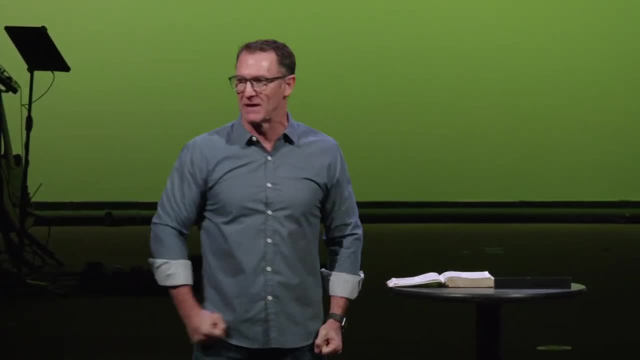 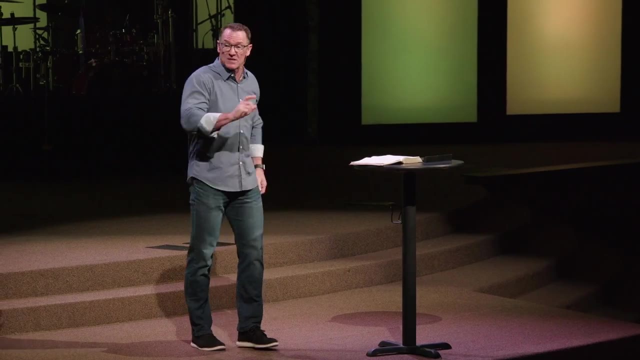 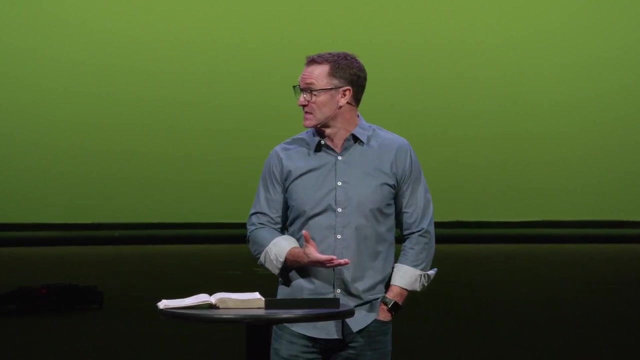 whatever I can do to win and dominate and overpower people, it just mattered whether you won. When Jesus showed up on the scene in the entire world, this is the first time that humility was ever a virtue. Jesus turned the world upside Down with this concept. 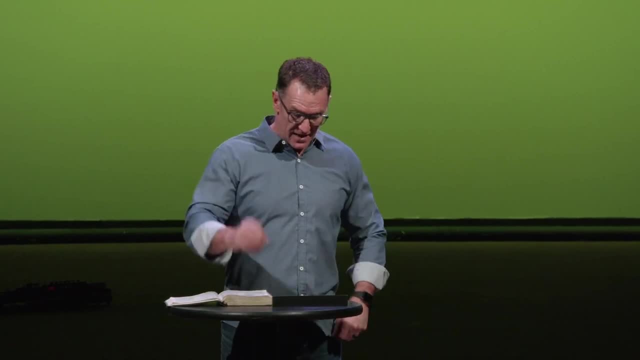 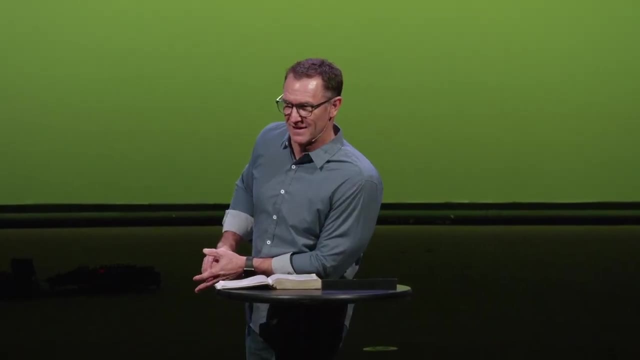 And Paul gets it. He says: be completely humble. So that's crazy, Not a little bit humble, Not fake humility Like, oh, I'm going to serve everybody else. You know what fake humility looks like sometimes It's when you serve people. 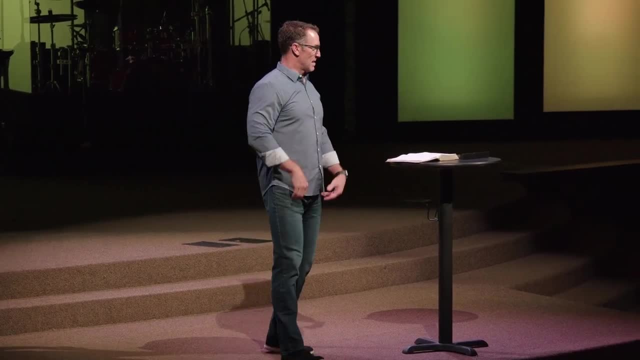 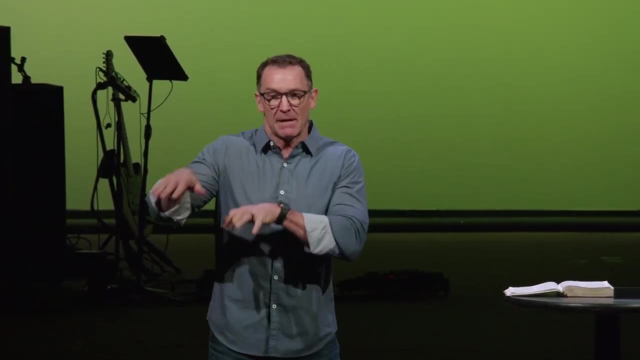 so that they'll take care of you. back, I'm going to help you and you keep score. How many times you help? Wait, I know this is starting to sound like marriage, right? How many times you unload the dishwasher? How many times you unload the dishwasher? 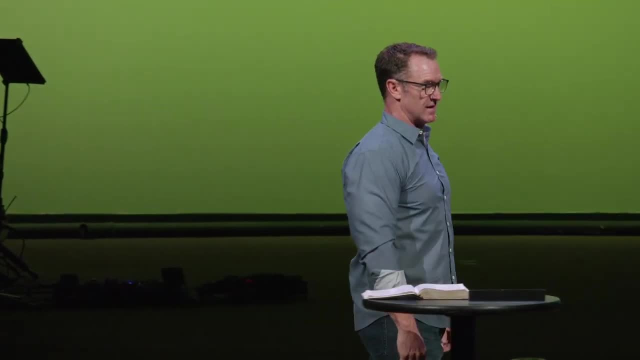 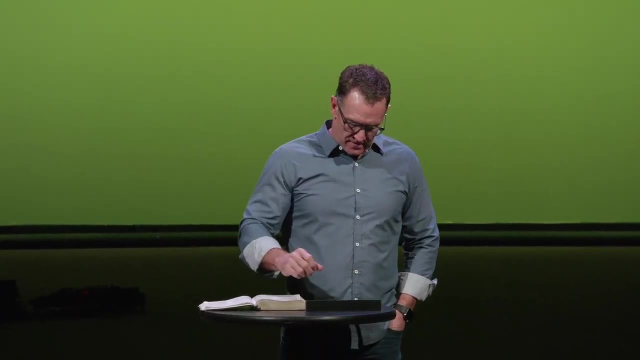 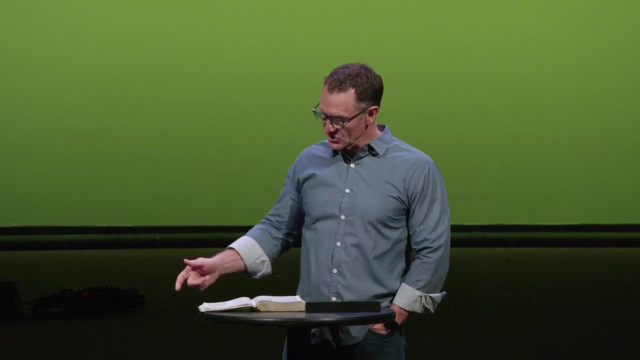 So that that other person will reciprocate something back. right, And we keep score. That's actually false humility. It's not actually real humility. I find it interesting too, though, when it comes to relationships in Paul and what he's writing, being completely humble. 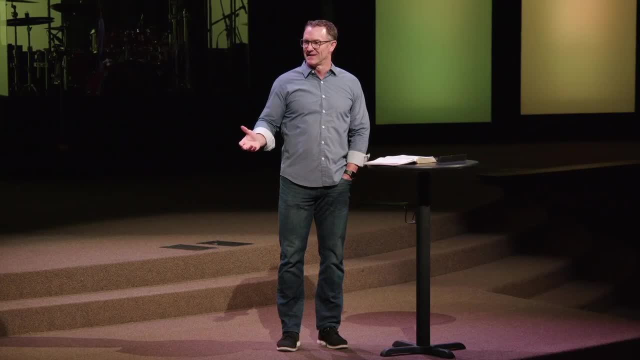 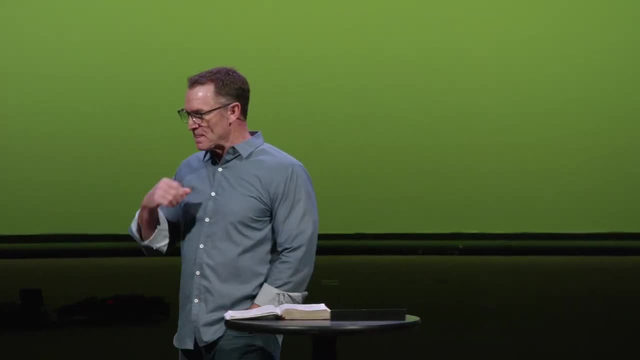 You might ask this question, like: did Paul ever stand up for his own rights? It's an interesting story in Acts 16.. I don't think it's in your notes, but you can just write the reference down: Acts 16,, 35, Paul is arrested for stirring up trouble. 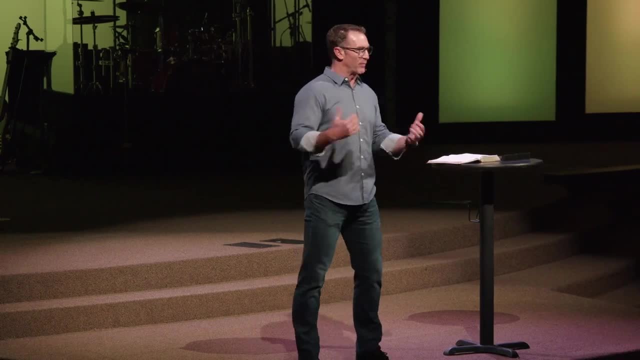 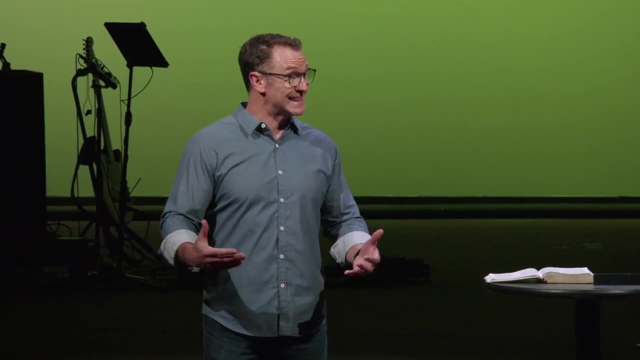 He's just telling people about Jesus. He is whipped and then imprisoned And all of a sudden, the guards and the jailers find out that oh, he's a Roman citizen, which you are not legally allowed. to whip and imprison a Roman citizen. 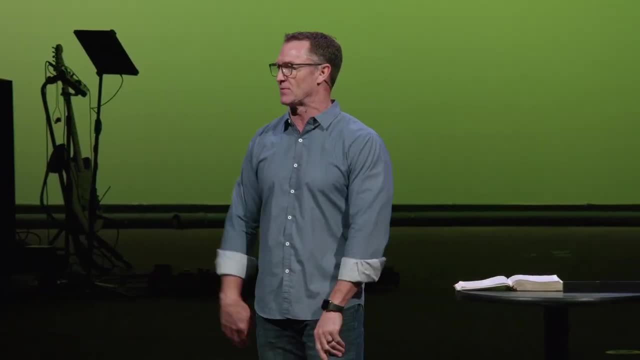 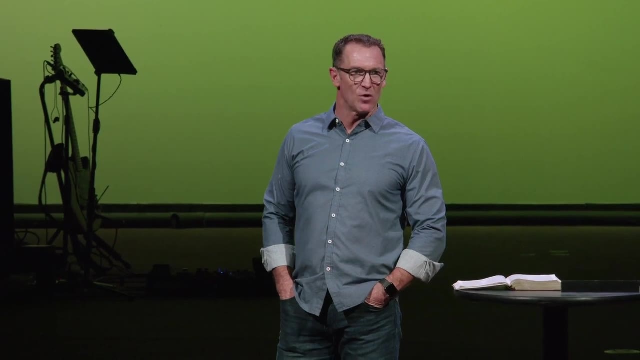 And so they're like: oh Paul, you're fine, You can go, All the charges have been dropped against you. And he's like: I ain't going anywhere, I want an apology. You just whipped and beat a Roman citizen. 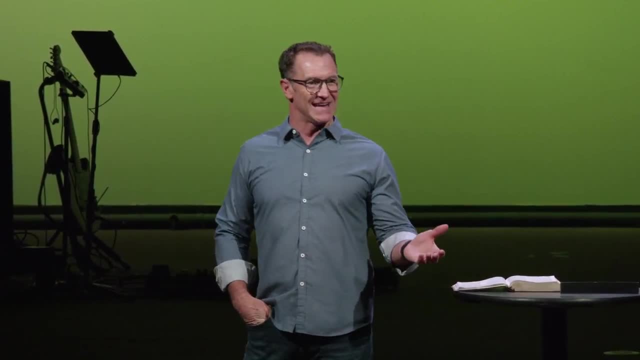 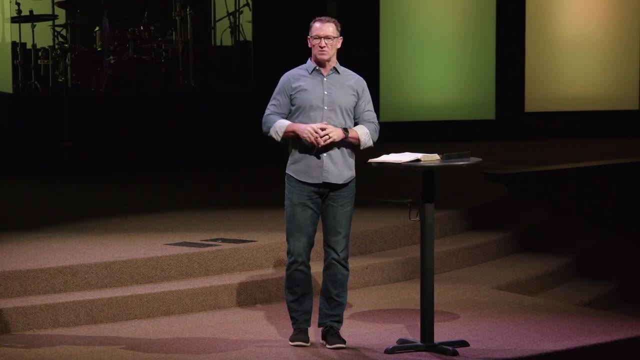 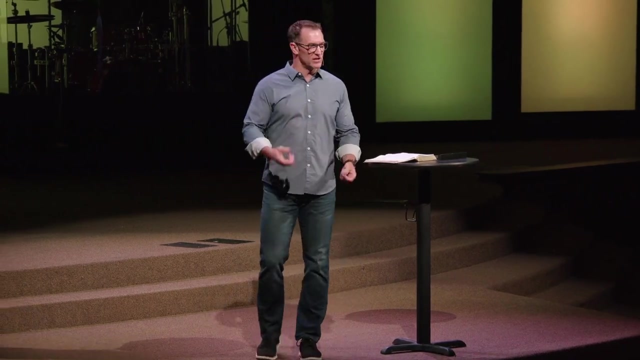 He actually stood up for the rights that he had. It's an interesting dynamic that we have to say when do you stand up for your rights And when do you put your rights aside for someone else? Can I just say this? Sometimes, I think we just want to be told what to do. 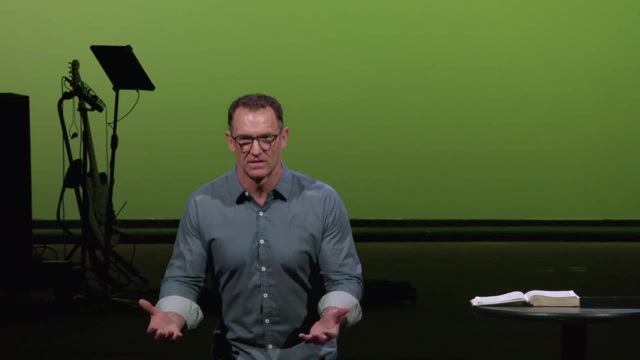 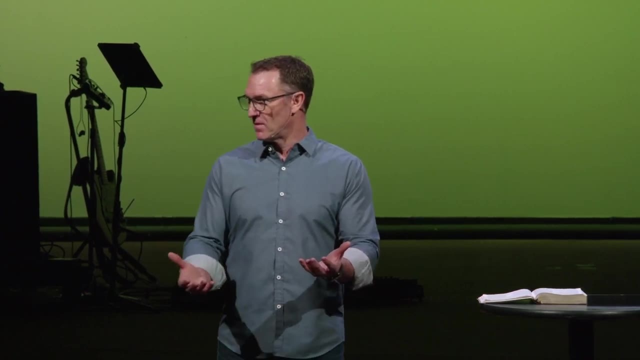 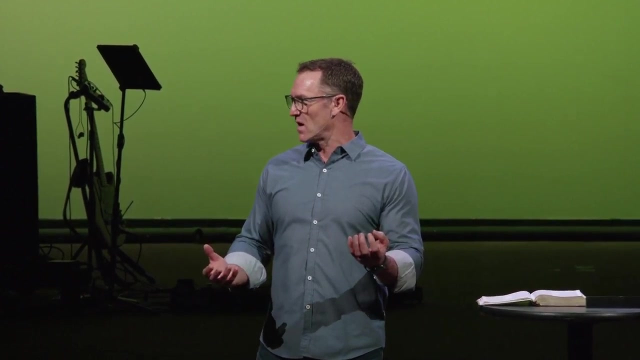 Here's the right thing, Here's the wrong thing. I hope you live in this tension. This says: serve people, love people, be completely humble, And it doesn't mean that you're a doormat and that you can just let all kinds of people walk all over you. 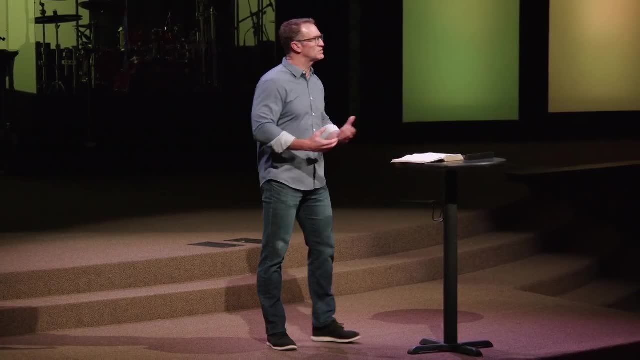 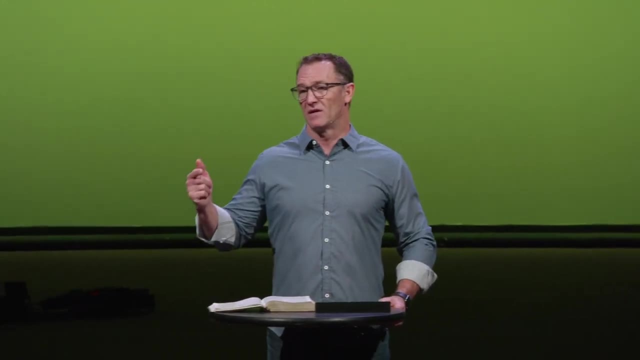 That Paul at some point stood up for his rights. I'm not saying that you can never sue somebody, right? Paul makes it really clear, like when it comes to lawsuits in the church, like you're just embarrassing yourself in front of the rest of the world. 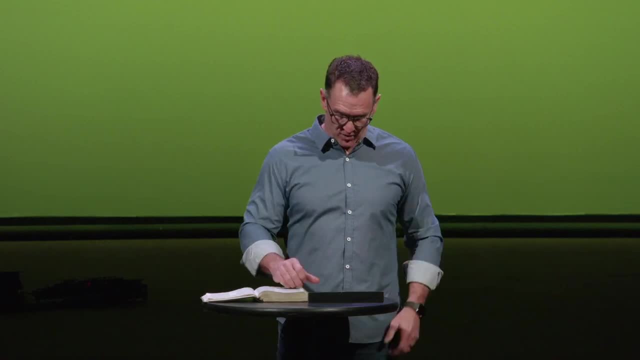 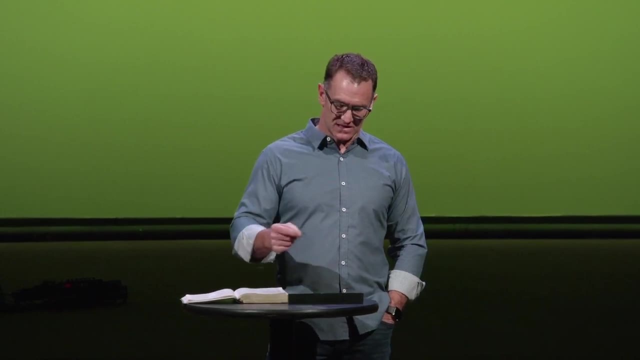 by Christians suing Christians. But Paul, at one point, stands up for his rights. He's like, no, that's not right, It's wrong, Be completely humble. But then he says this: I want you to be gentle. The word is meekness. 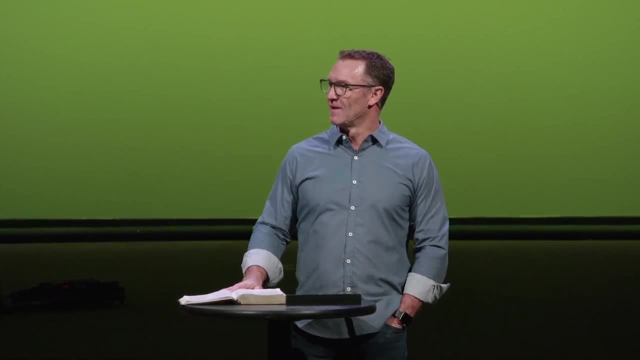 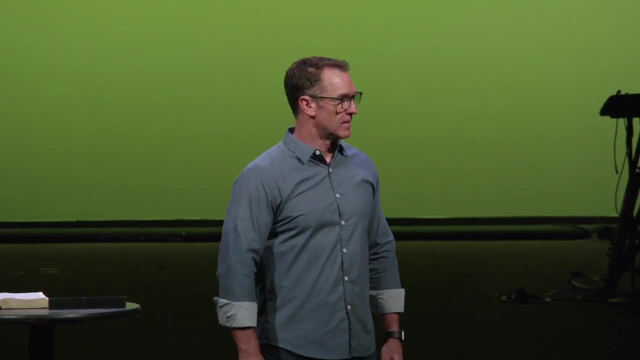 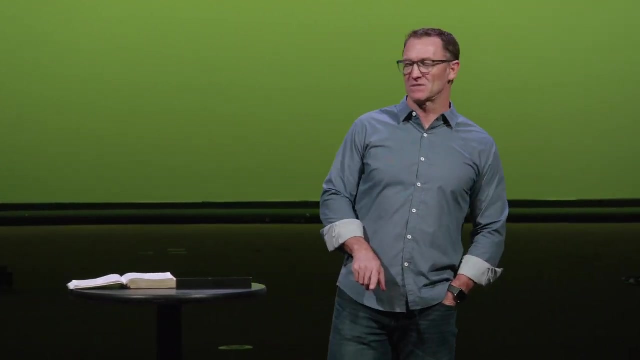 and it doesn't mean you're weak and you're powerless. This concept of gentleness is actually power under control. You could rise up, but I choose gentleness. The problem with gentleness is this, guys: particularly for us, gentleness is sometimes. 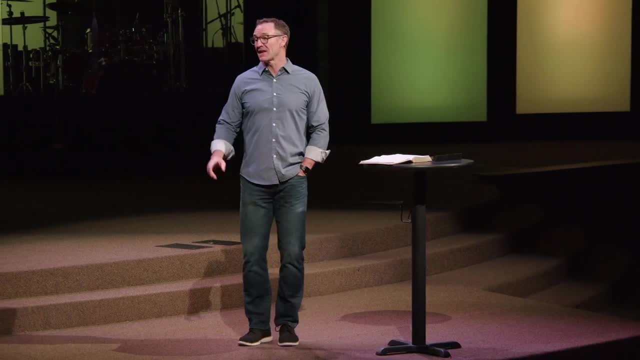 we don't want it to be interpreted as a weakness. And maybe it's not a guy thing, Maybe it's a lady thing too. Don't make it a guy thing, Don't make it a lady thing. Don't mistake my gentleness and my kindness for weakness. 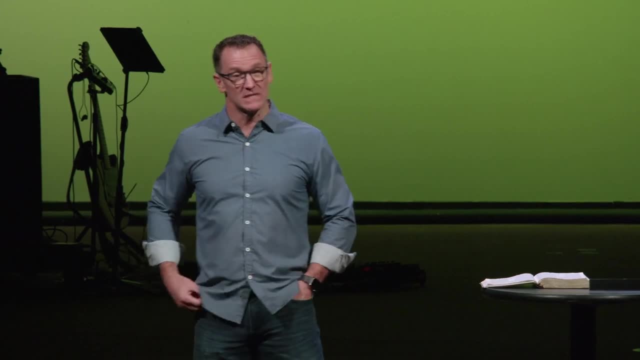 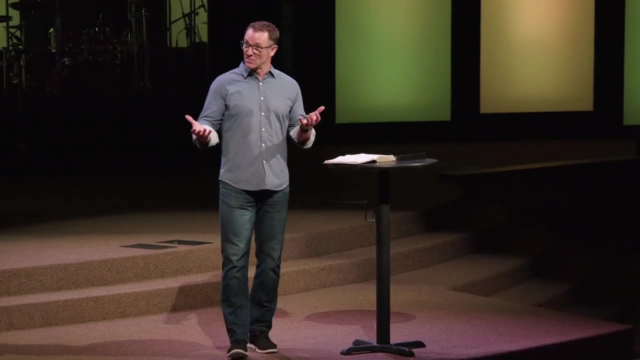 I don't want to have to rise up because there is a time and a place, maybe, for that. We're going to live in this tension of the world. We're standing up for your rights, but also being completely humble and gentle. Now make note of this. 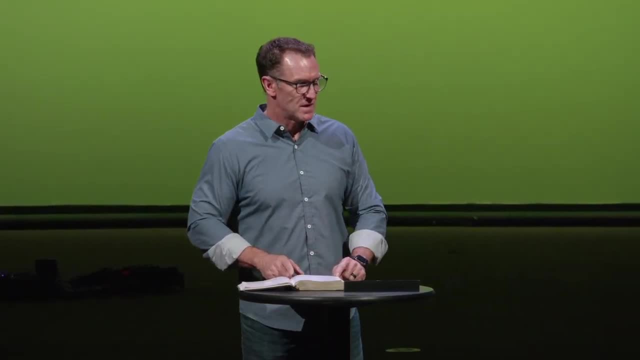 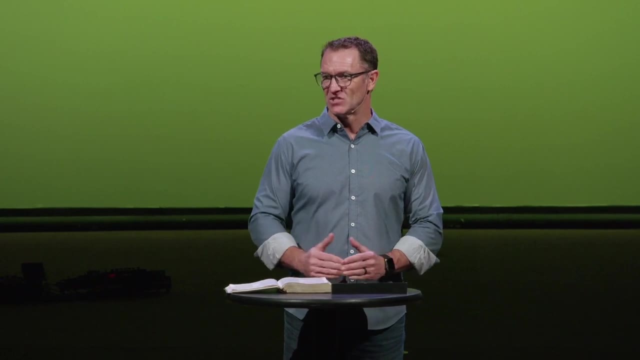 He's writing to believers and Christians in the church: Be completely humble And when it comes to dealing with your Christian brothers and sisters, I want you to be gentle. So imagine you build a bridge to people in your church who aren't like you. 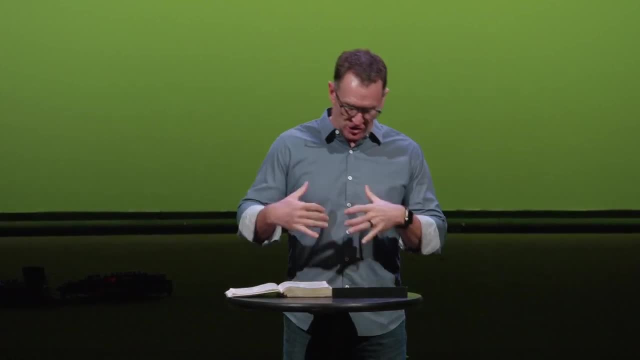 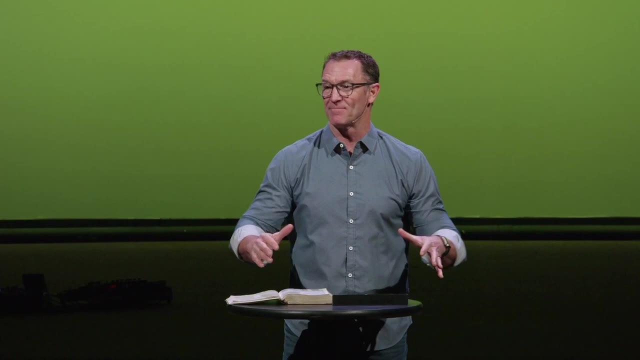 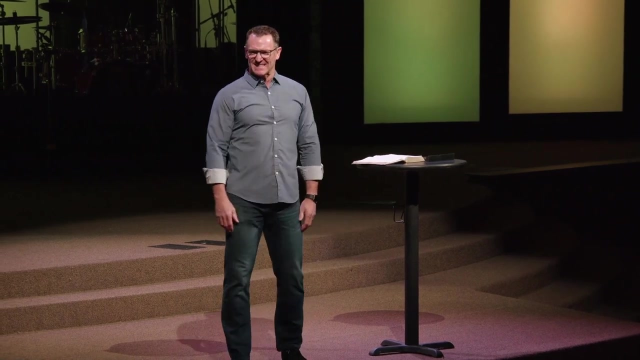 They have different backgrounds. They don't vote like you, They don't look like you, They have different traditions than you. You build a bridge by being completely humble and gentle. And then how do they respond to you? They offend you, They say something dumb to you that hurts your feelings. 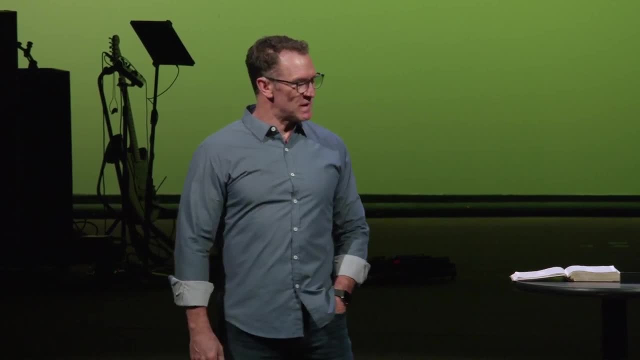 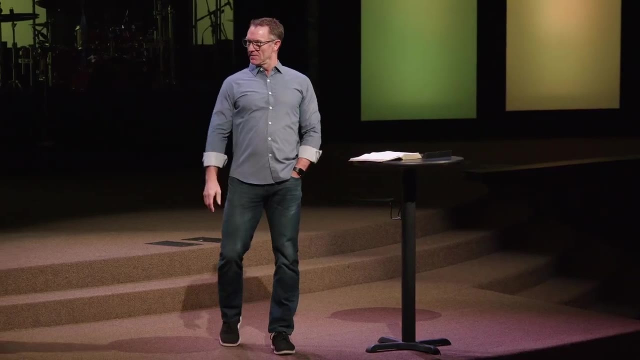 or they ghost you Or you're like man. we have invited those people over to dinner or a house twice. We fed those people and they haven't even reciprocated. They haven't had us over. Not only that, but they walked by me in the lobby. 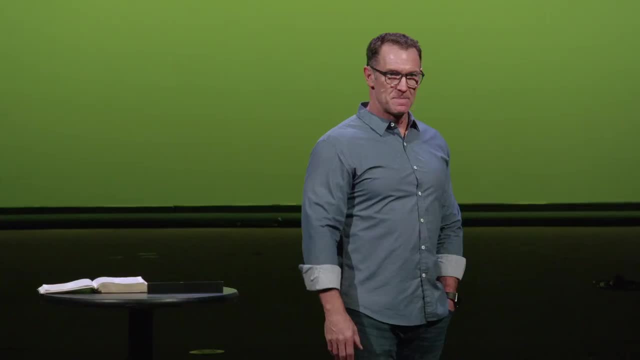 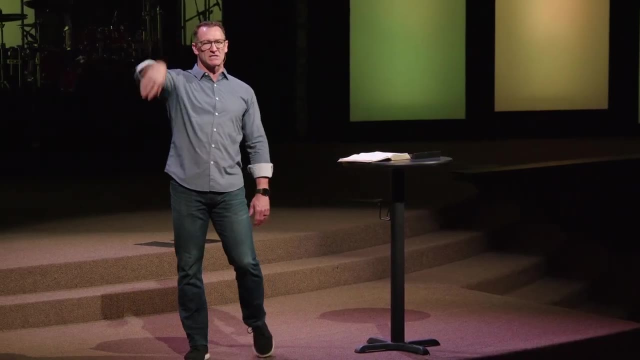 Didn't even say anything like that. I don't even exist. And all of a sudden they start saying or doing things that are offensive And you're like I'm going to get on their Facebook page. And all of a sudden you see that they post things. 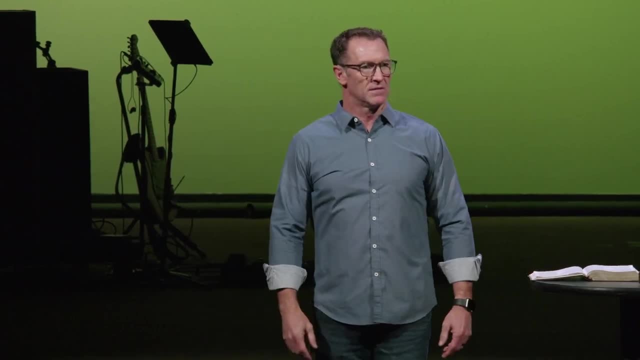 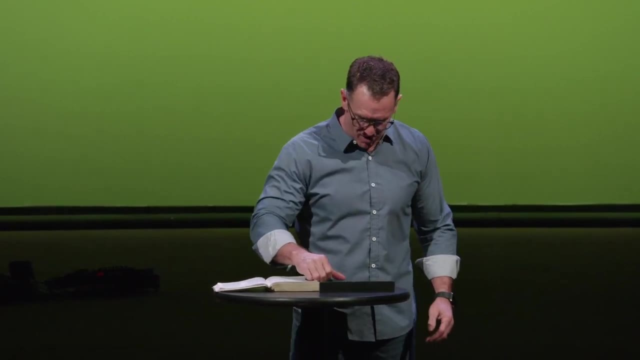 that you just disagree with And you're like we are never going to be friends. Go back to the text here just for a minute, Be completely humble and be gentle, And then what's the very next step, The very next thing that Paul writes on there? 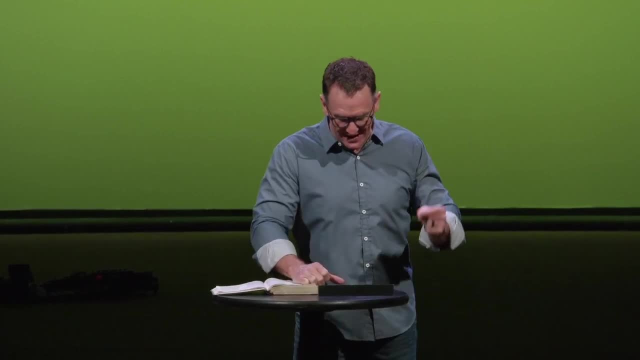 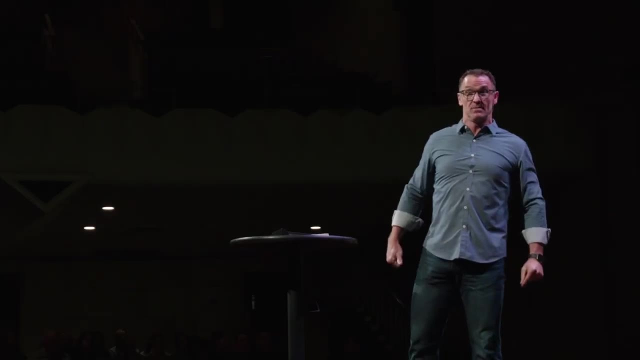 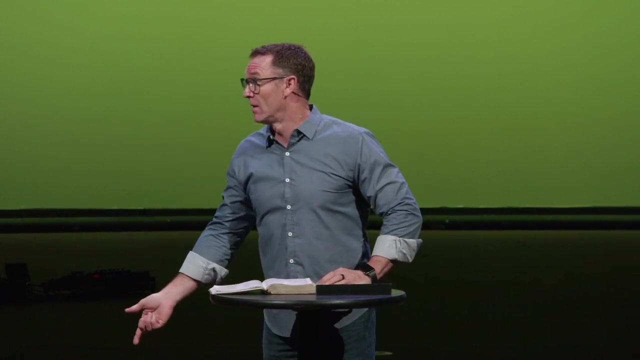 Be patient and bearing with one another in love. Once you imagine the bridge and build the bridge, then you got to fortify the bridge. Why You don't have to be patient with perfect people. You don't have to be patient with people. 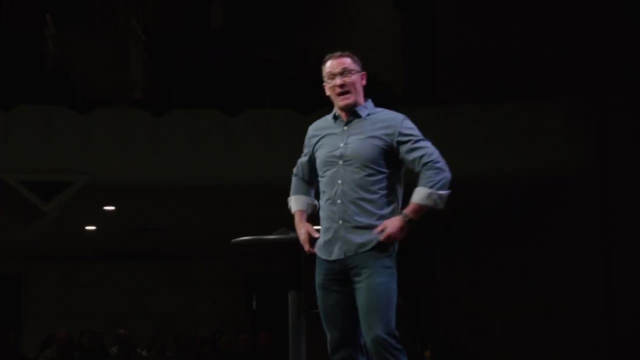 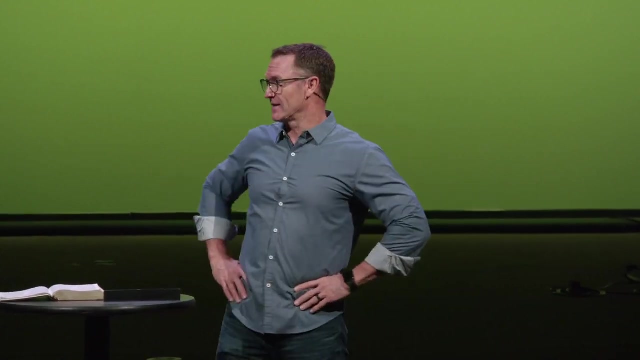 who make you happy. all the time You got to be patient with irritating people. Welcome to church. Look around, Don't look at your family. All right, There's going to be irritating people. There's going to be people here who hurt you. 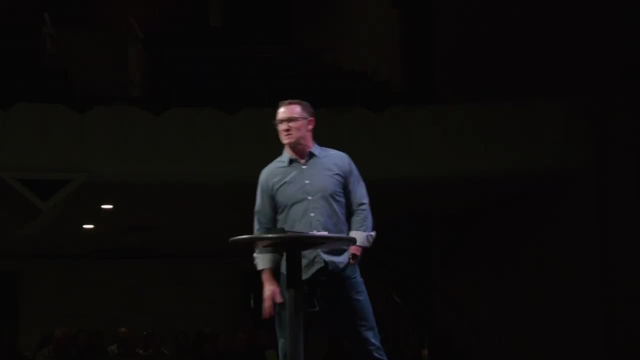 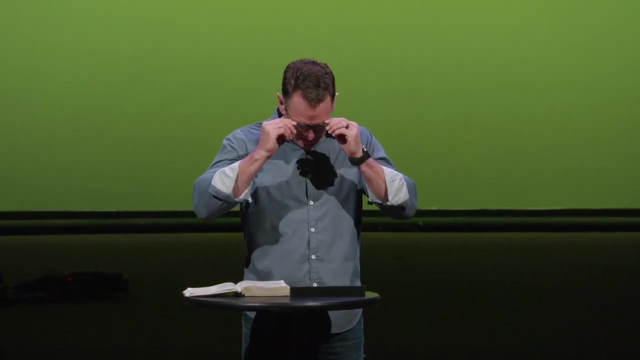 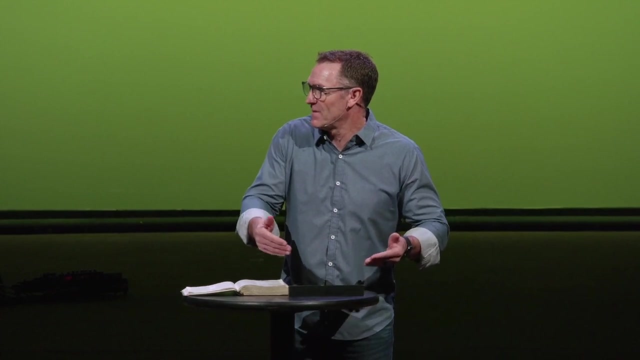 offend you, let you down. Some of them will do it on purpose because God's still working on them, But some of them, unknowingly, are going to hurt you. Paul knows this. Once you build the bridge by being completely humble and gentle. 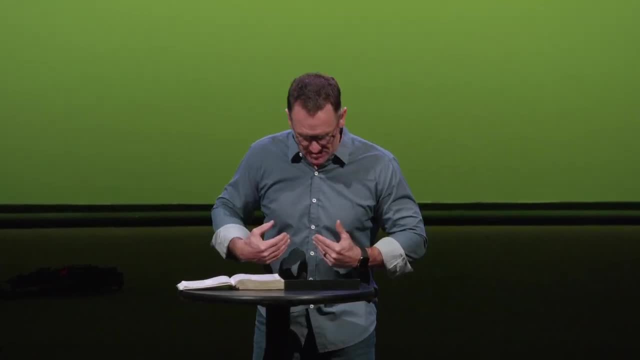 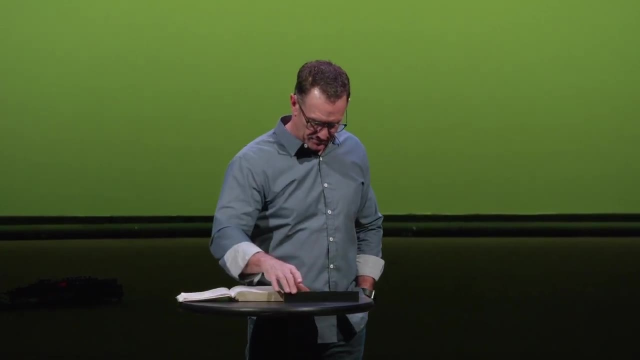 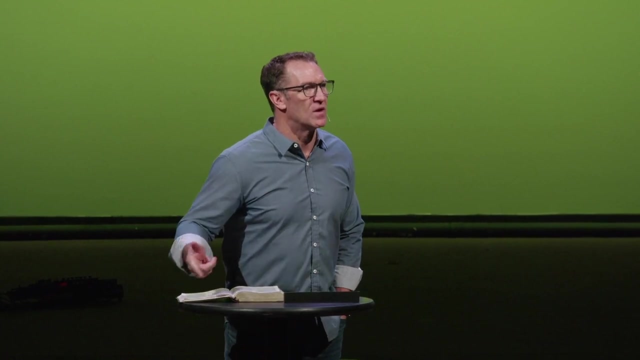 and then they respond with something that's unkind. here's the deal. Now you get an opportunity to fortify the bridge by being patient and bearing with one another in love. I think we have to fortify our bridge by this Anticipate that people will wrong you. 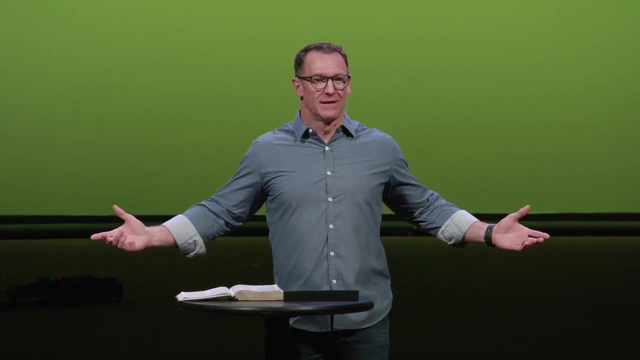 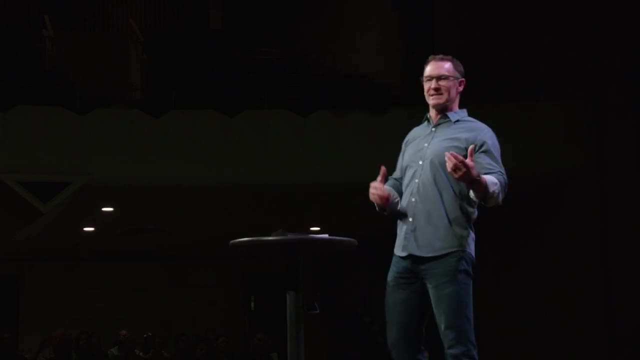 If you anticipate it, it means this: You don't have to react to it Because, come on, we all got triggers, don't we? You got a trigger, And if someone says something to you, comments about something, like, it is your trigger. 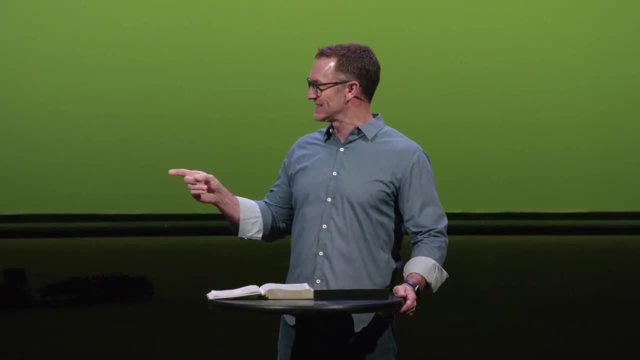 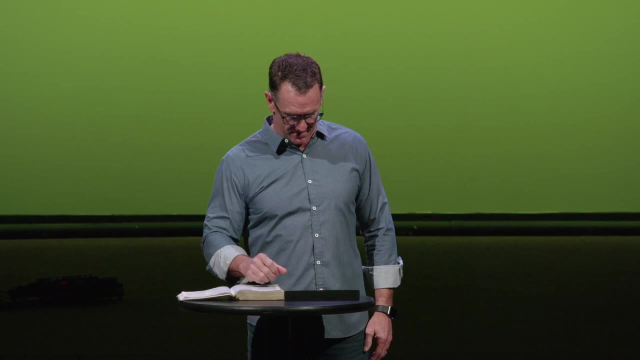 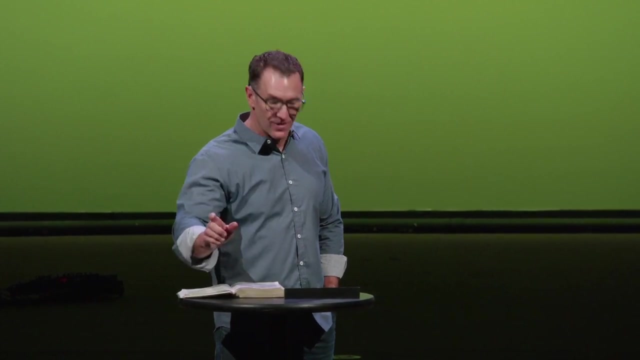 and you're like you're going to react unless you've made the decision ahead of time. I will not allow that trigger to divide me and them. Paul, in this he says: bear with those people. Oh, here's what's so interesting. 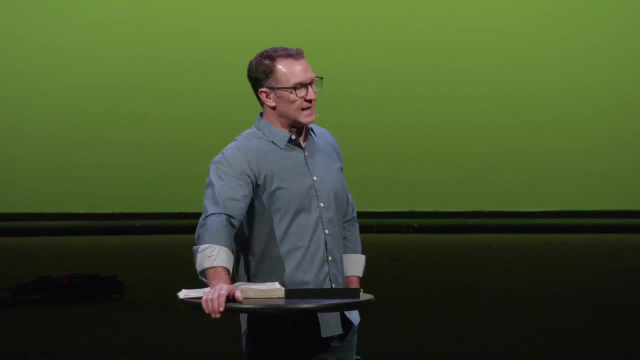 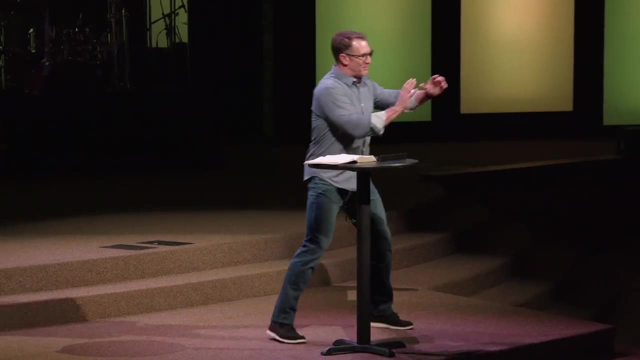 He says: bear with one another in love. He doesn't write this: Bear with those people in love. And there's a difference: Bear with those people in love and bear with one another. What this means is bear with those people. It's like you're looking at people and Paul's like. 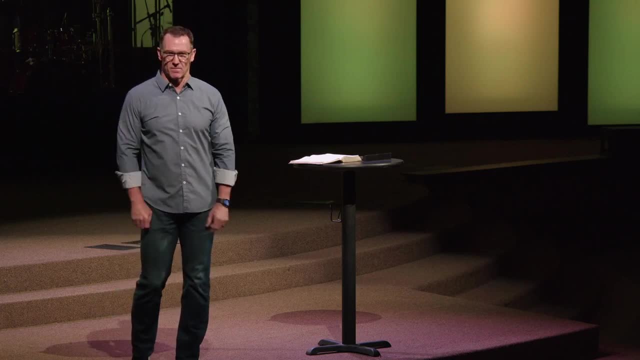 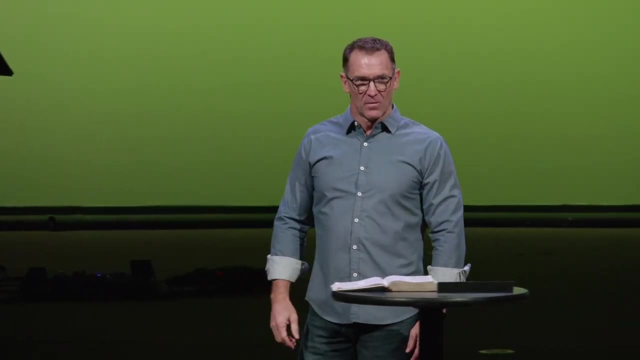 hey, listen, people are going to offend you. They're going to hurt you. You need to bear with them As if they're the offender, and we always get it right. What he writes is: bear with one another in love, which is anticipating this. 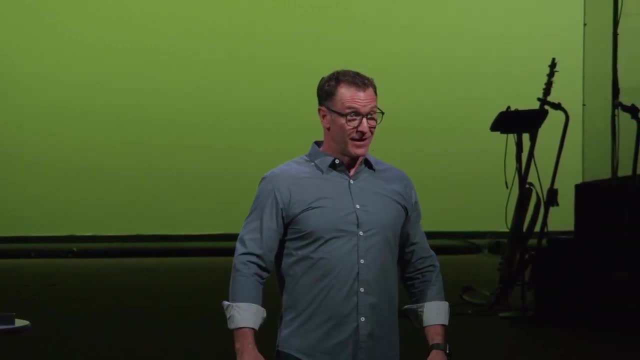 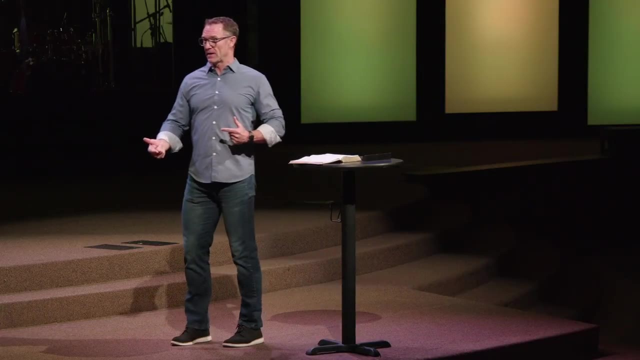 At some point you're going to get it wrong too. You're going to crack a joke that you thought was funny and it's actually offensive. You're going to ignore somebody. You're going to actually talk behind somebody's back. You're going to do something to start tearing down that bridge. 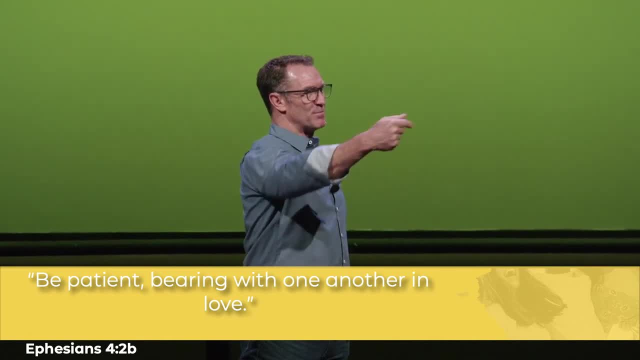 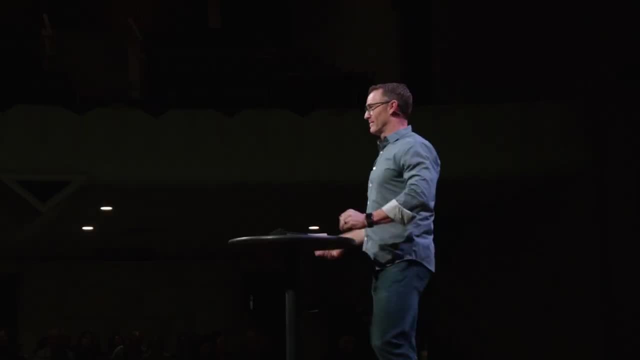 It's not just you bearing with them in love, It's their call to bear with you and put up with you. All the perfect people in the room raise their hand. Okay, good, Uh-huh, Yeah, Not old enough to know. 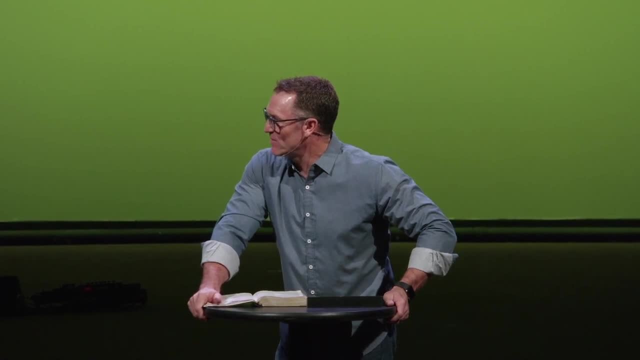 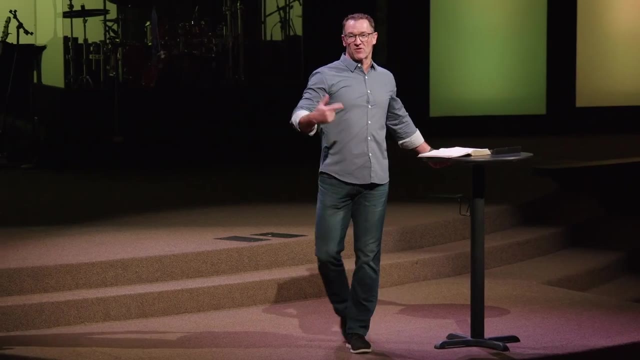 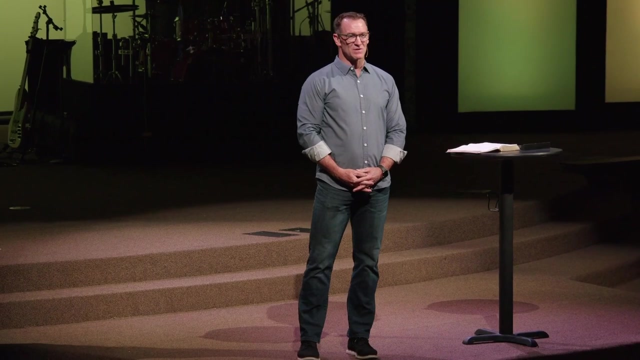 Here's what's great. Think about this. Everybody wants a safe space, don't they? Don't you want a safe space? We want to create safe spaces for each other, but here's the safe space for you. Even if you mess up, the grace and mercy of God covers you. 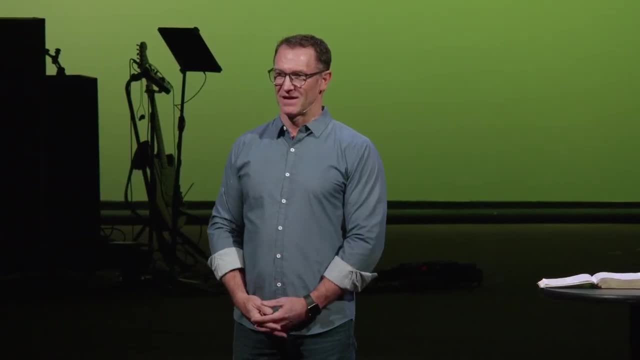 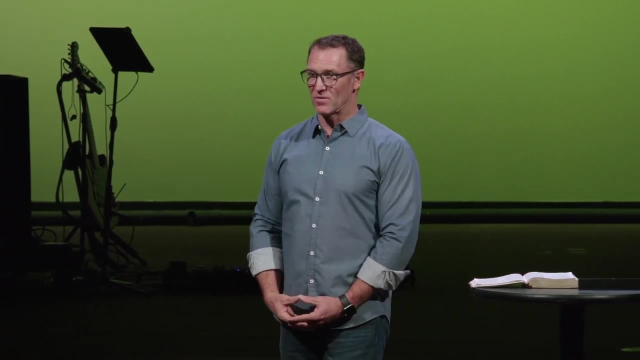 and other Christians will recognize that And the grace and mercy of God will not allow it. It will allow it to disunify you and I. In all of your brokenness, you have a group of people that will love you and encourage you and stick with you. 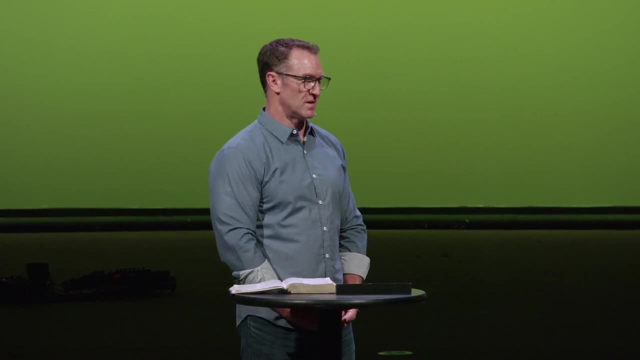 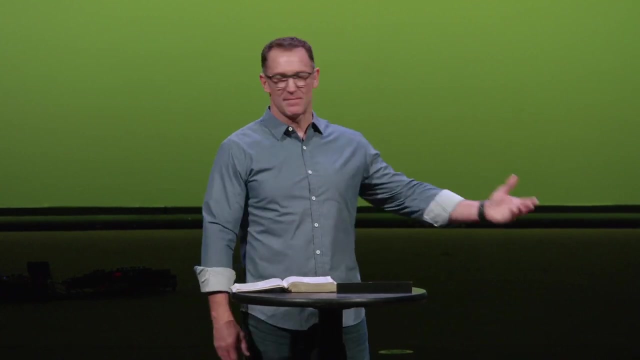 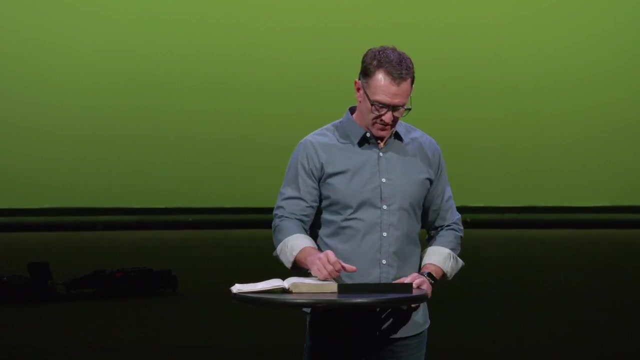 That's what the church was designed to be: to love people the same way that God loves them and accepts them. That you could take a Levi, you take a Simon the Zealot and put them on the same team and they would be defined by their love for one another. 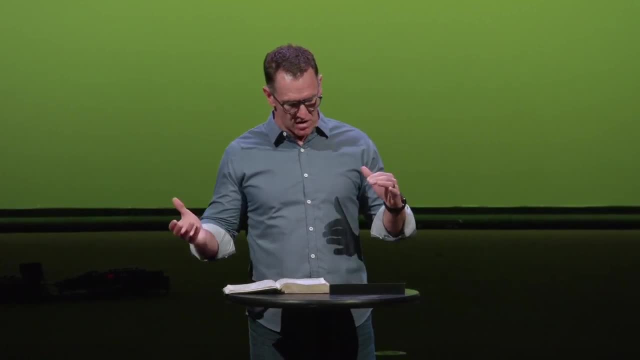 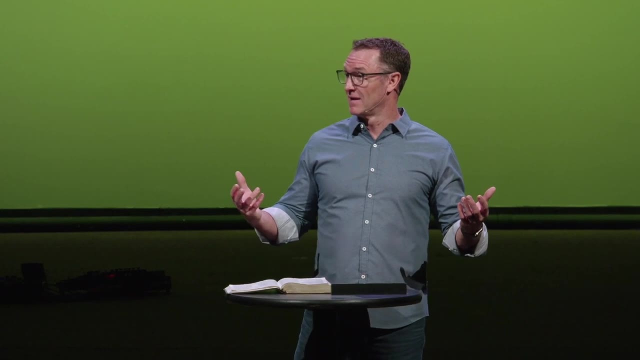 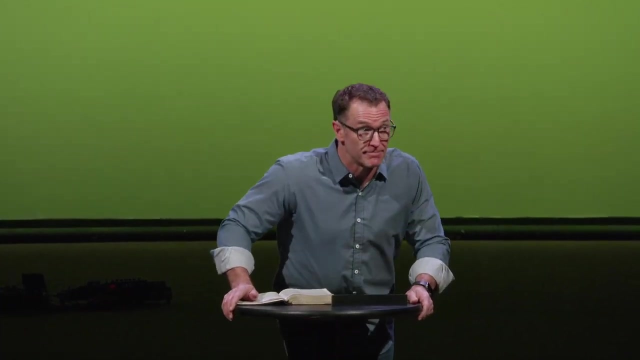 I think the concept is this: Don't allow someone's wrong to produce a wrong in you. When you're wronged, it's so tempting to wrong them back. And there's this deep, deep religious philosophical principle that says: two wrongs don't make a. 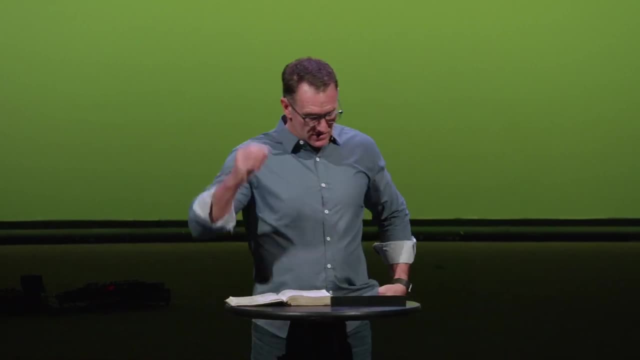 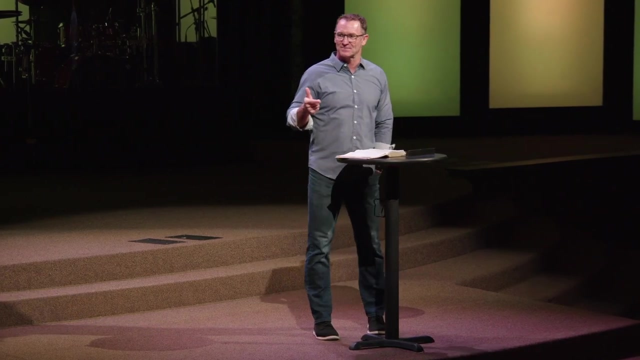 Yeah, you learned it when you were three. Let me hit a quick side note on this and I might run out of time on this. but quick side note, I've mentioned this a lot but in circumstances, sermons like this, where we talk about the unity, 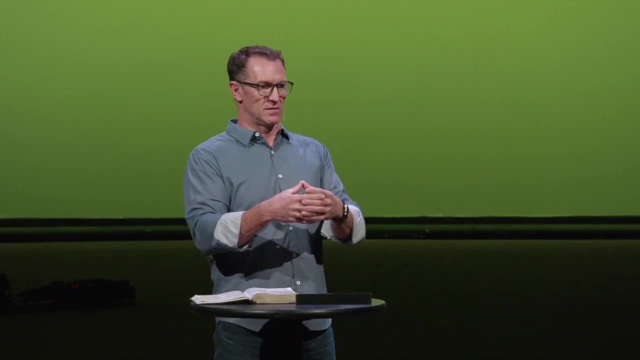 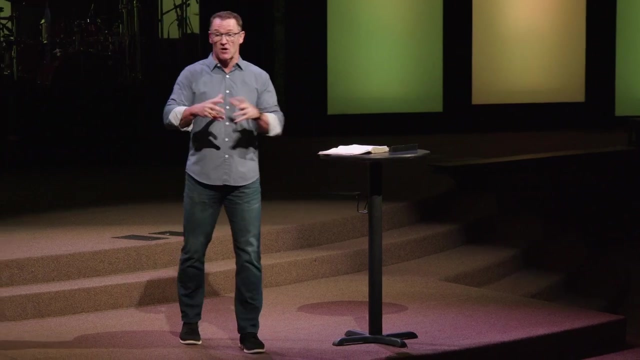 it begs this question: Is it ever appropriate to build a wall? And I want to make sure I hit on this because I mentioned last week that, listen, it's not just about unity in the church. You can take all of this philosophy and put this philosophy into your marriage. 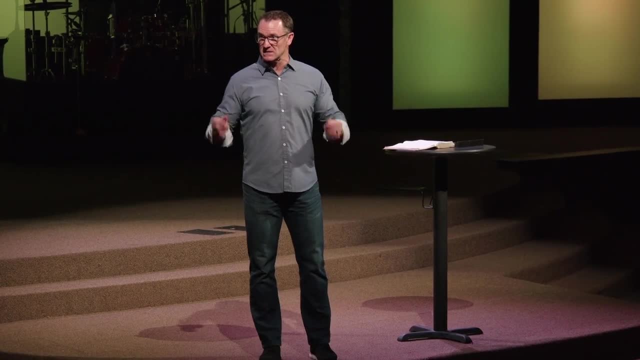 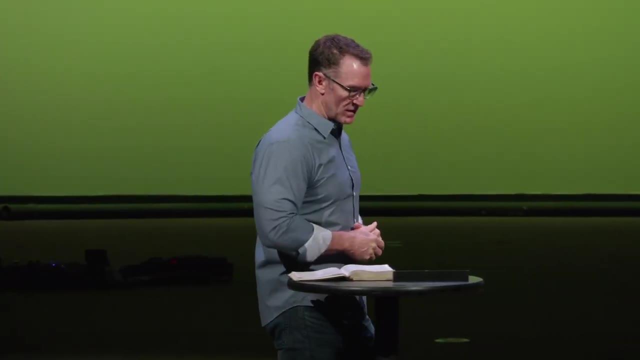 And you're like. well, under every circumstance, am I supposed to have unity in my marriage Question? is it ever appropriate to build a wall? There's a book written by Henry Cloud called Boundaries He's. You've probably heard this. 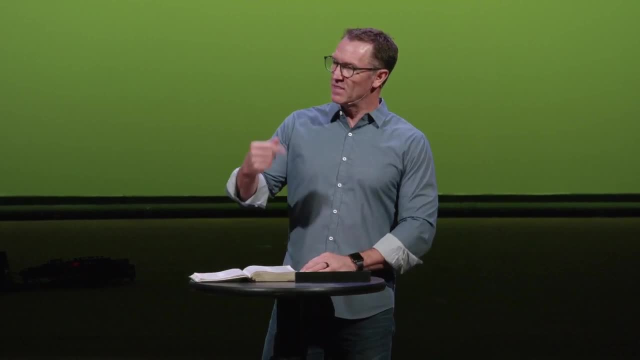 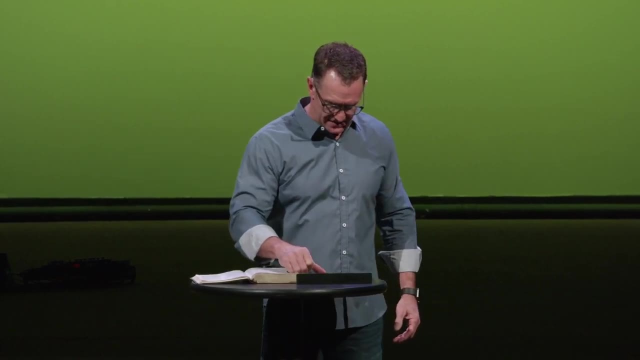 I've mentioned this before, but I think it's worth noting again. In this book he describes three types of people that are from the book of Psalms and the book of Proverbs. The three people are the wise, the foolish and the wicked. 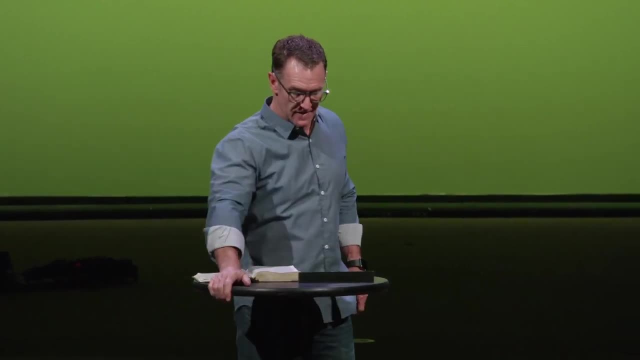 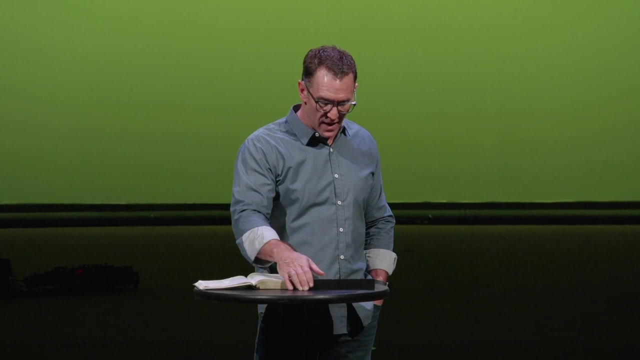 Give you a verse here: Proverbs 12,, 15.. And this is in the back of your notes. Fools think their own way is right, but the wise listen to others. A fool is quick-tempered, but a wise person stays calm when insulted. 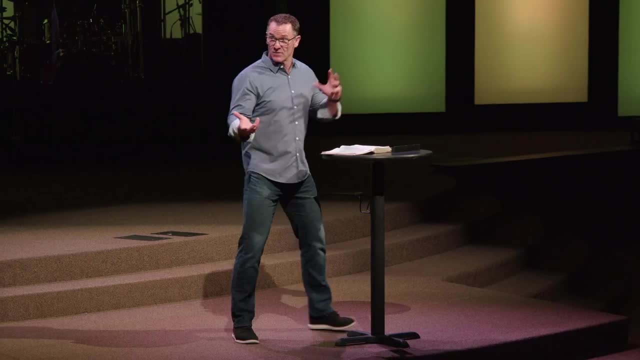 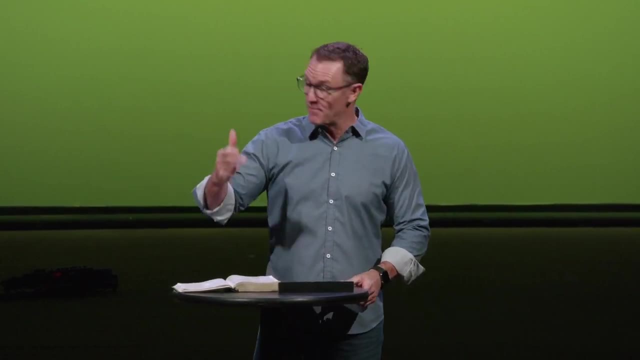 So there's There's the wise and there's the foolish in this verse. Here's the wise. They're humble, They're not perfect, They receive feedback, They apologize when they've done wrong And they restore relationships. See, the wise don't need walls. 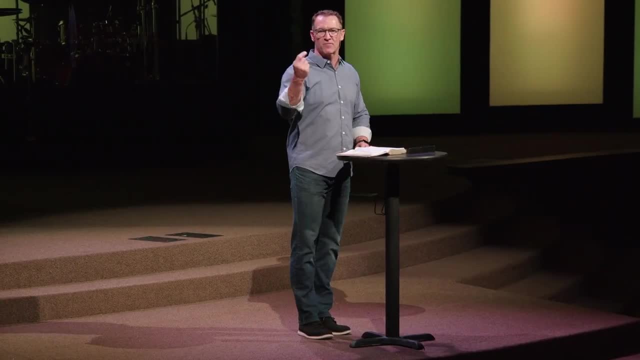 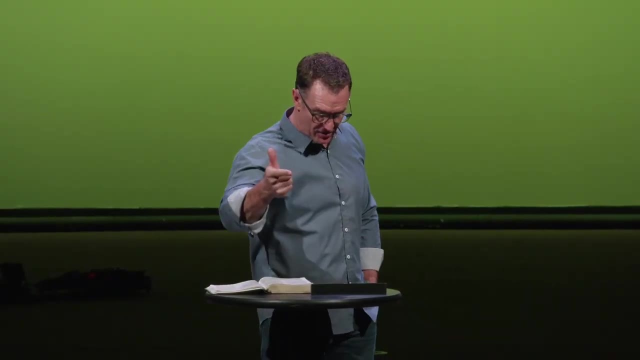 The wise just need to hear the truth from you in a loving, safe way And they'll respond appropriately. But then there's the fool, The foolish people. they don't listen to feedback, They respond in anger, They remain contentious. These people need some kind of walls. 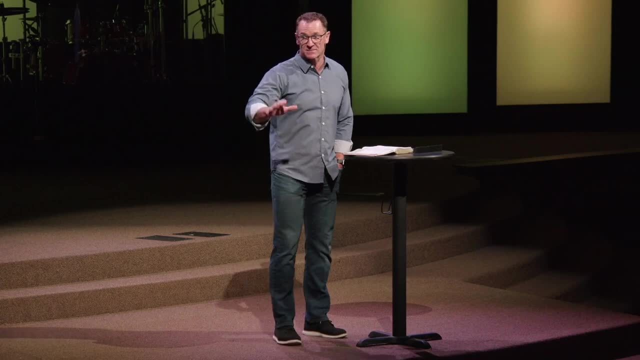 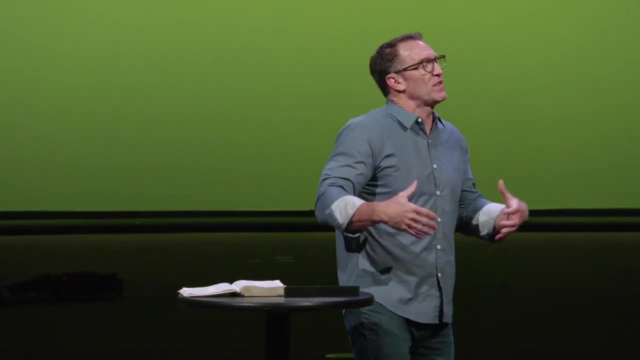 that are called called consequences. Sometimes they need physical walls between you and them, But the walls that you put up are consequences to behavior so that with the hope that they might become wise people- I mean, when you're raising your kids- don't you put consequences in front of them? 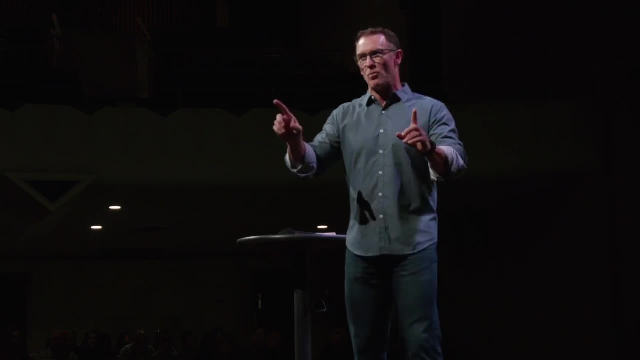 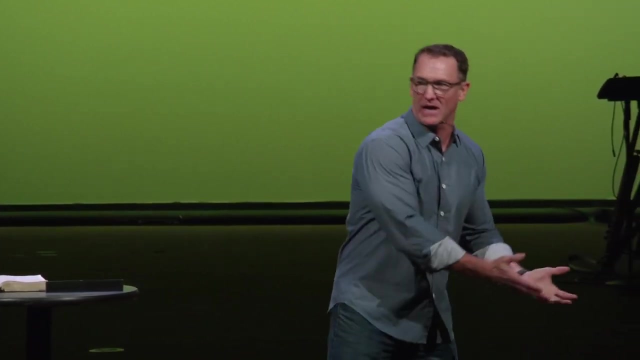 that are walls, to say no, you keep running into that same wall. My hope is that you will become not the fool for the rest of your life, but that wall of consequence will allow you to gain some wisdom to say, oh, I don't want to live that way anymore. 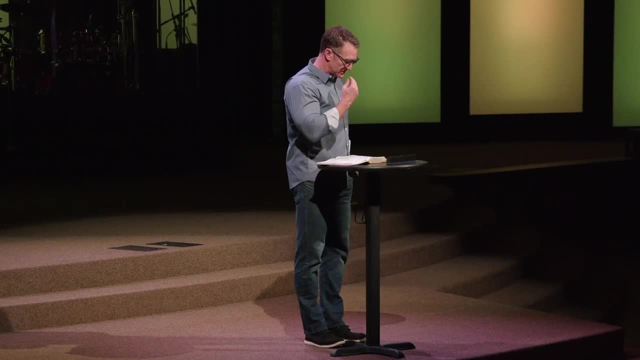 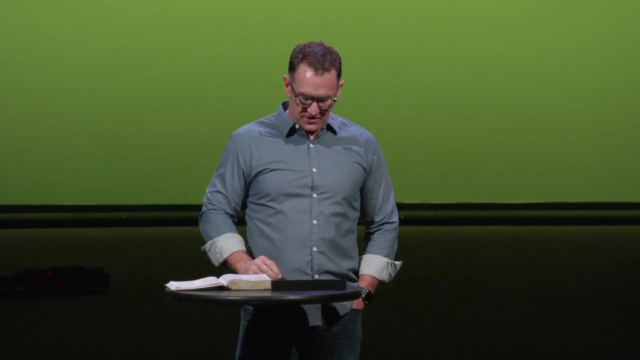 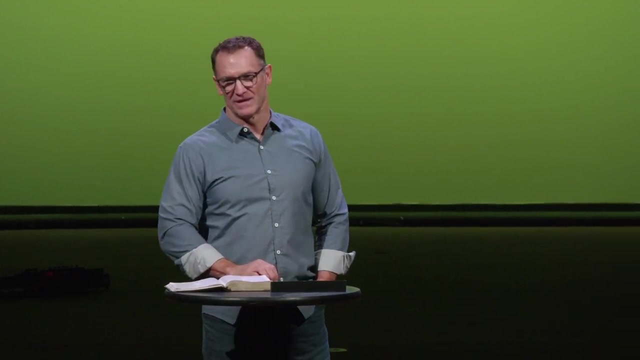 You also have a group called the wicked. Psalm 37 reads this way: The wicked lie in wait for the righteous intent on putting them to death. Wicked people: they enjoy hurting people and they need walls, Things like prison walls. You don't treat everybody the same. 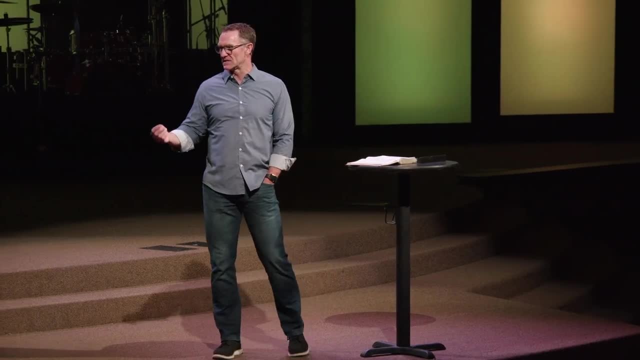 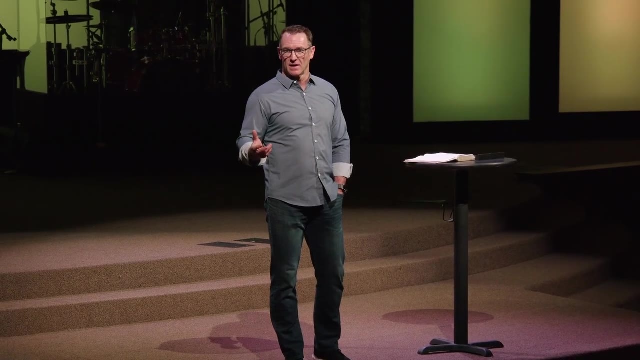 So here's why I bring this up in a message about unity. My concern is that some of you are like: well, listen, I'm married and in my situation there's abuse happening And I don't want you to be like. 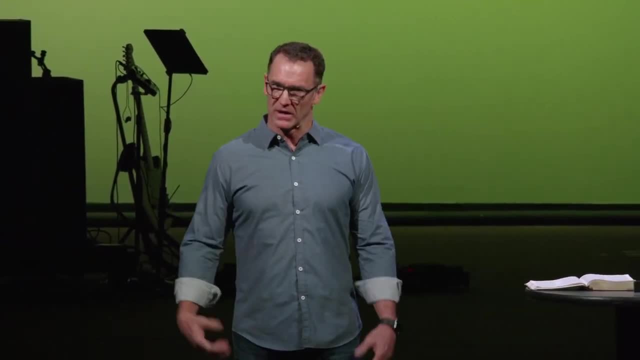 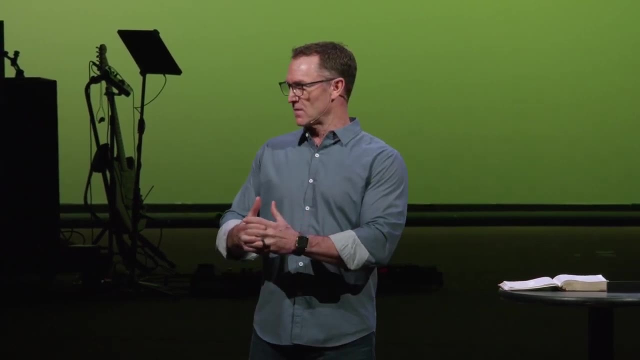 I don't want you to misinterpret this. to say, hey, there's unity, at all costs, I mean be completely humble. No, no, no, no. The assumption is that when we're talking about unity, that you're with either wise people. 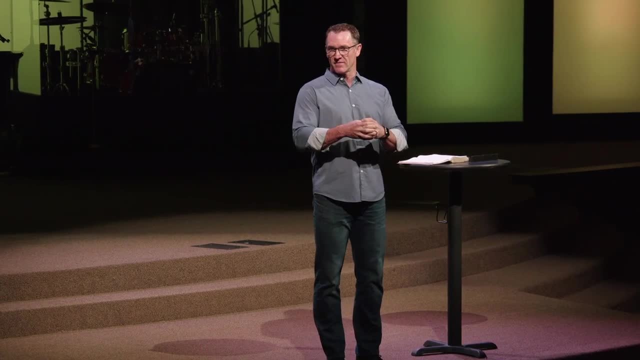 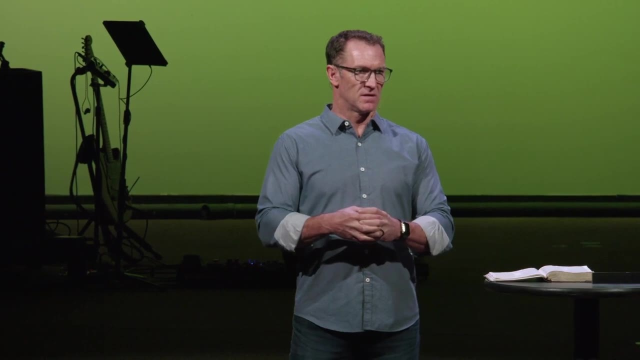 or maybe foolish people, so that you can have unity there. It's never with wicked people. You have an abuser in your house. You need some walls there and you need some safe boundaries. Are we okay in that? I want to make sure that that's clear. 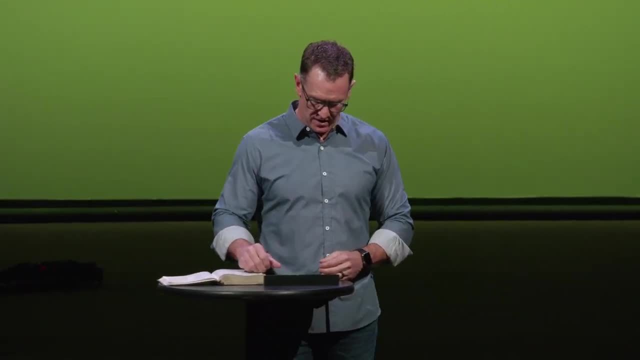 so that no one misinterprets what I say: The pastor's never telling you that God is okay with abuse. So let's go back to the bridge. We imagine the bridge, build the bridge, fortify the bridge. Here's the fourth thing. 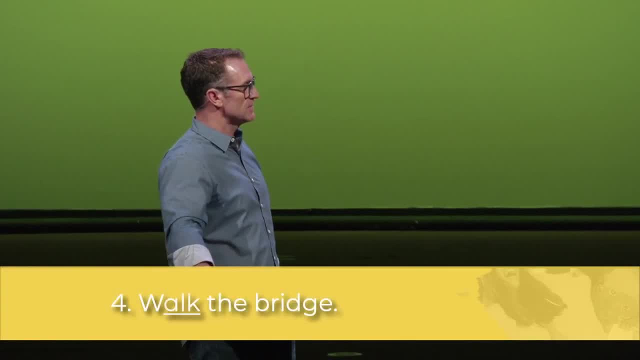 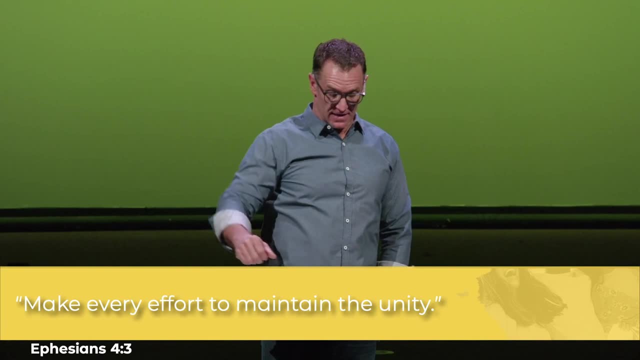 wrap up with this. maybe We need to walk the bridge. The text says this: make every effort to maintain the unity We can say: I built a bridge. Listen, I tried, I made an effort. They need to meet me partway. 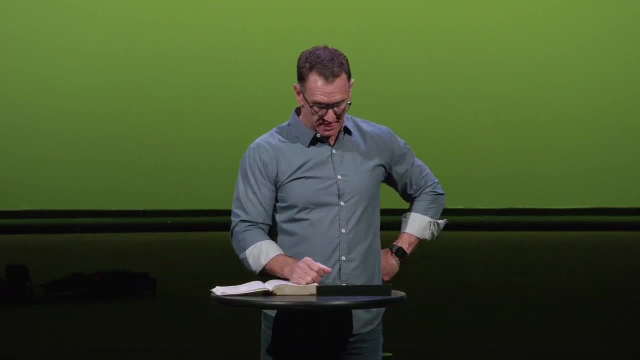 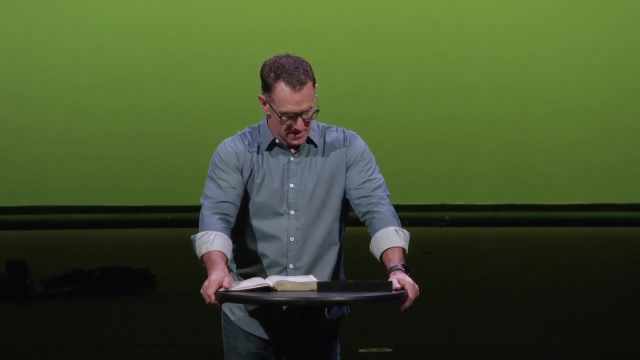 or I built a bridge. They can walk over it. now, Make every effort to maintain the unity It means. it means this: I think You better keep walking that bridge. We keep walking over to the other side, even when it feels unsafe and unreciprocated. 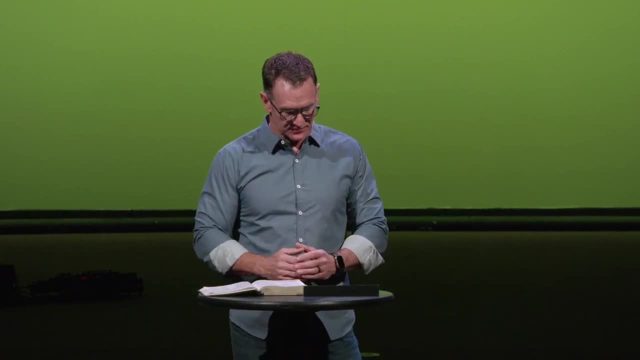 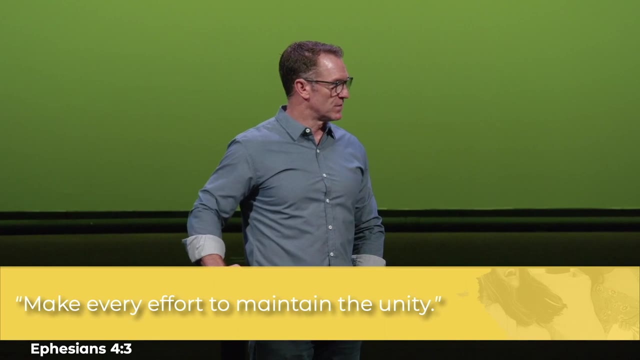 Make every effort to maintain unity and connection. See, I think there's two major threats to us in 2024, this year, particularly in this political year, an election year. The first threat is aggression. People don't know how to talk. 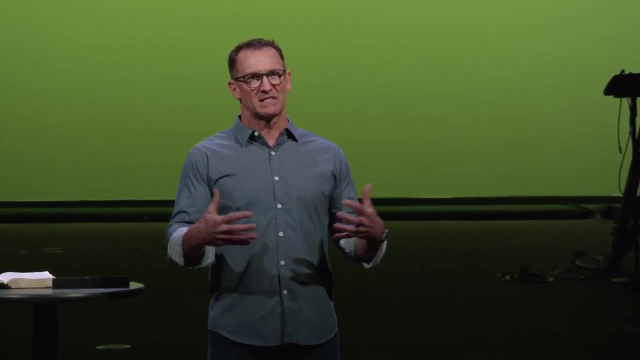 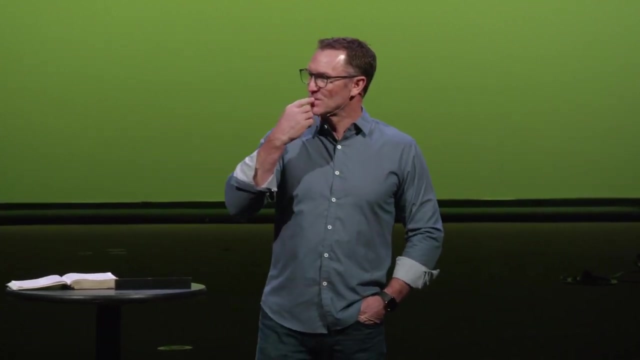 They don't know how to disagree. They don't know how to agree on things without the aggressive nature, And so there's this, but that's not the only enemy. I think there's another enemy in the church that is actually the opposite of aggression. 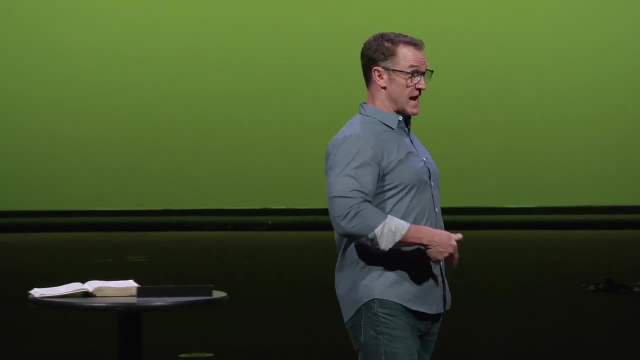 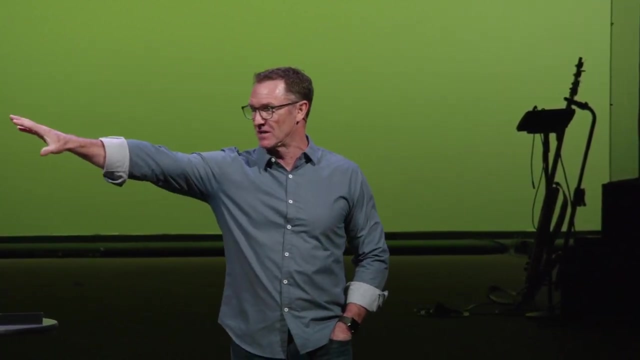 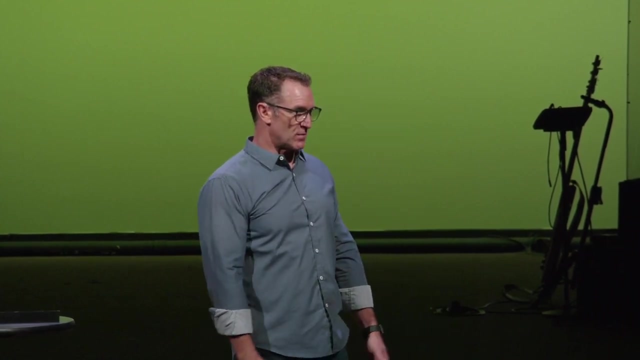 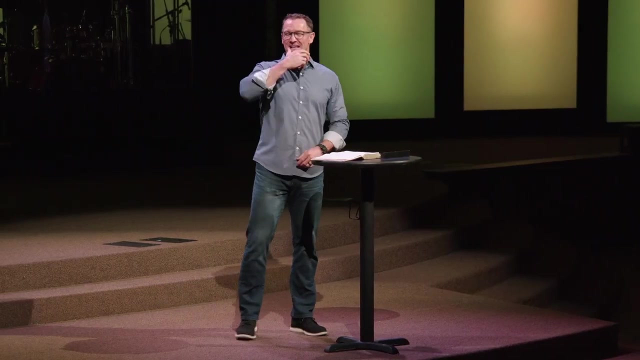 and it's isolation. Creating unity, making every effort to maintain unity in a church is not about a lack of aggression, because a lack of aggression can simply lead to isolation. God wants you to build a bridge to people so that they're not isolated and you're not isolated. 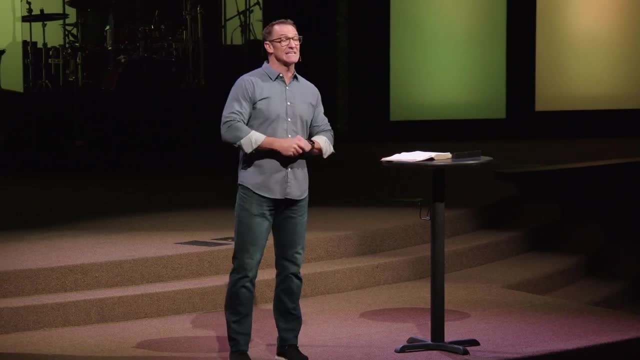 And I know, listen, there's some of you in church like I love you And you say things like I just don't need a lot of people, Like I got a couple of people around me, like I'm good. 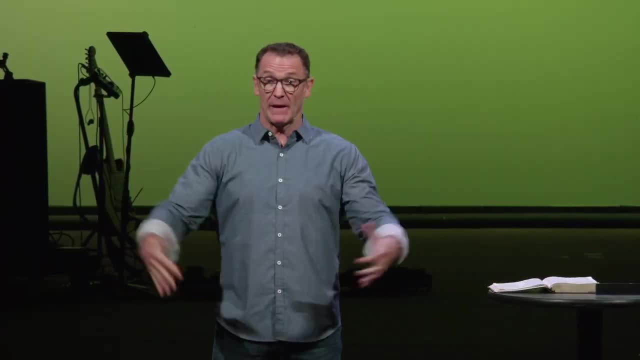 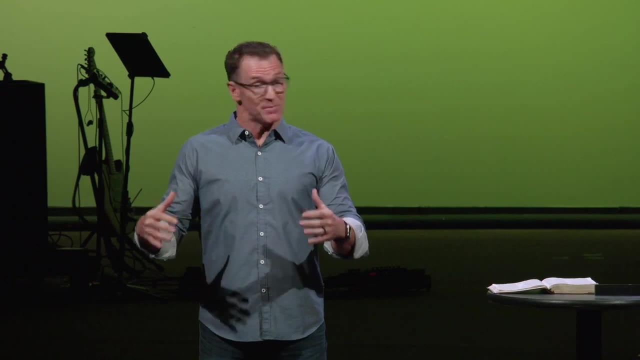 I don't need to build bridges, Like I just don't need a lot of people. And I just want to just remind you, like it ain't about you, If you're thinking just about your needs. what if there is someone in this church? 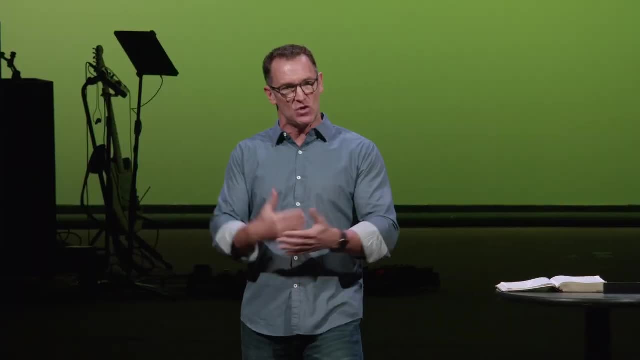 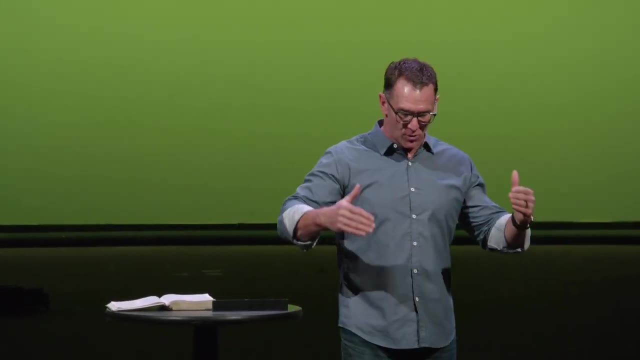 that is so isolated, but you have things in common with them that you might be able to build a bridge of relationship so they might feel finally like they belong. And I know it's safer, It's more convenient, It's more economical, It's more efficient to have two people. 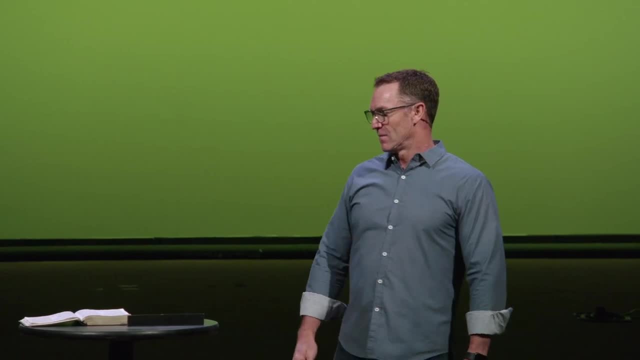 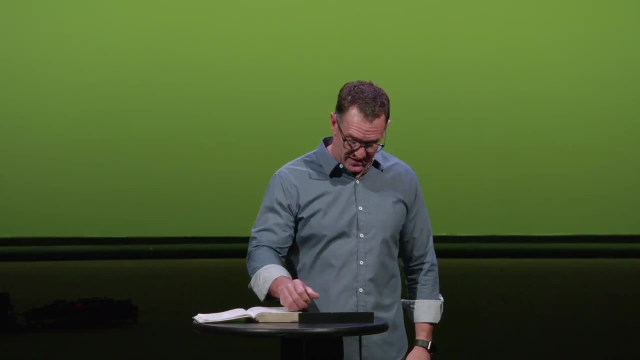 that you know and spend time with. But you have to read this and say it says: make every effort to maintain the unity of the spirit in the bond of peace. Are we Community groups in this church? they're bridges. Courses are bridges. 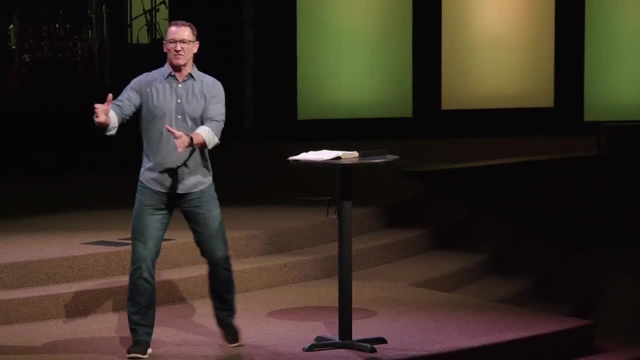 Divorce care bridge. We have these things called stage of life gatherings- All of our kids like when you get kindergarten parents together, we call that a stage of life gathering. When we get middle school parents together, that's a stage of life gathering. 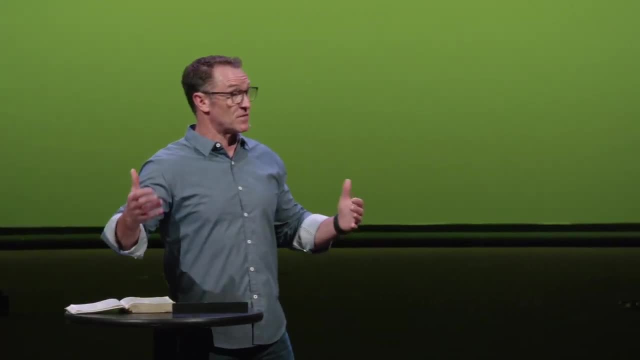 Some of you who don't have kids there, like you, don't even know we do this right, But we do this for these parents. Why? So they're not isolated. Those are all bridges. The parties on the patio are bridges. 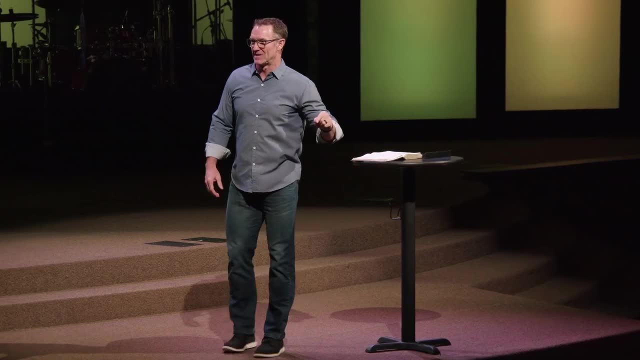 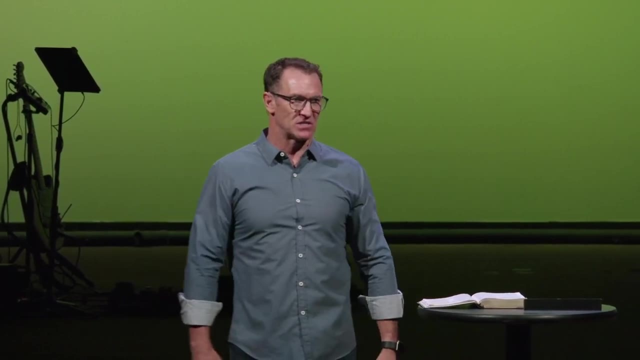 Our lobby is a bridge But question: it takes people Who are focused on connecting those bridges Walking across that bridge to get to know people Meaning this. you can walk through that lobby and it might've been a bridge, but you didn't cross it that day. 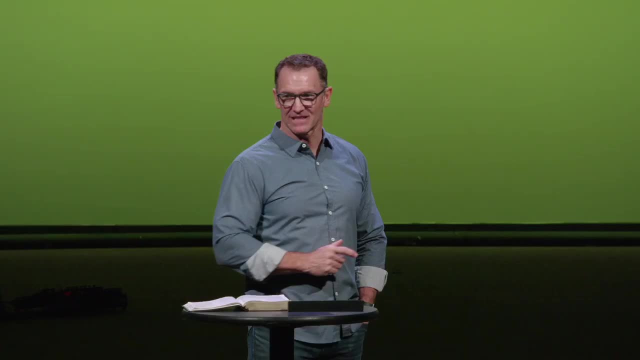 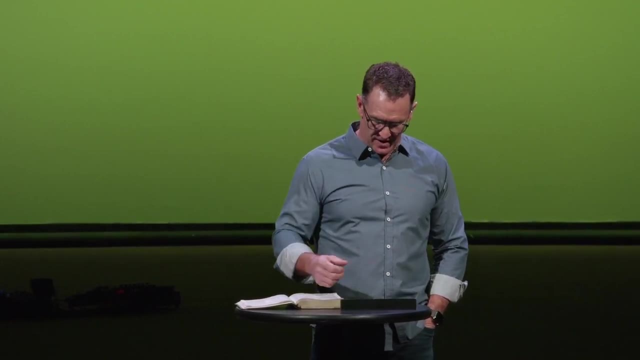 It's about connecting with people, Not in isolation, not in aggression, but connecting people so they feel like they belong and they are loved in this body of Christ. You know, I'm gonna, I'm gonna put off the rest of this until next week. 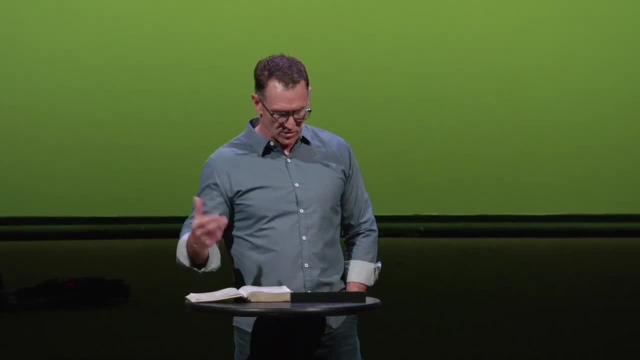 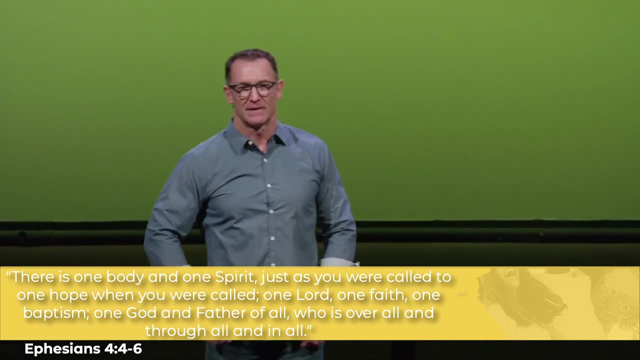 Where it says there's one body, one spirit, one Lord, one faith, one baptism, There's one hope. He says there's seven of these one things. I'll just point out one real quick. When he says there's one hope, 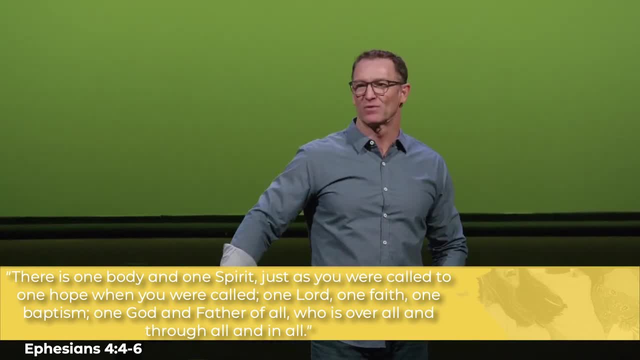 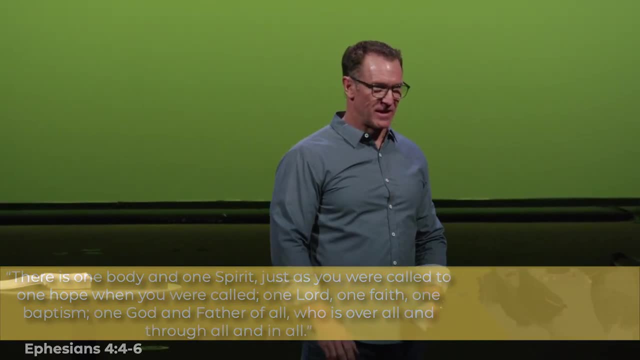 this political season you're gonna hear all kinds of hope presented to you. There's a new hope in town, right? Any politician that you hear in a speech quoting the word hope. just when they use the word hope I. I hope this phrase comes to mind. 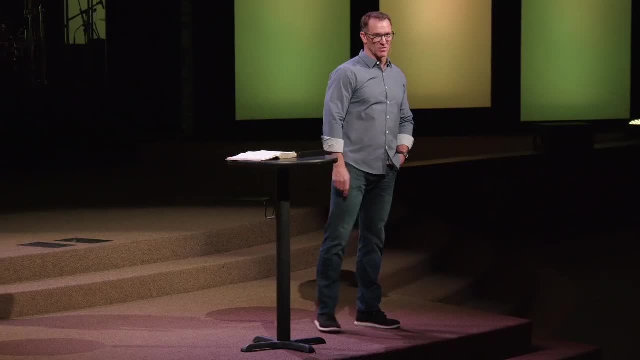 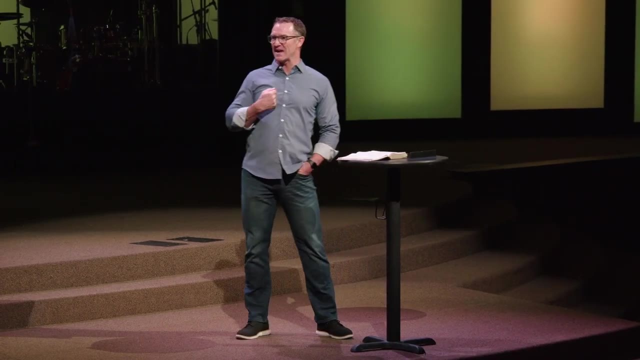 There is one hope, There's only one actual hope in the world, and it's not a political leader. Our one hope has a name, and his name is Jesus, And when he enters people's lives, he saves them and then transforms them. Our one hope in this world. 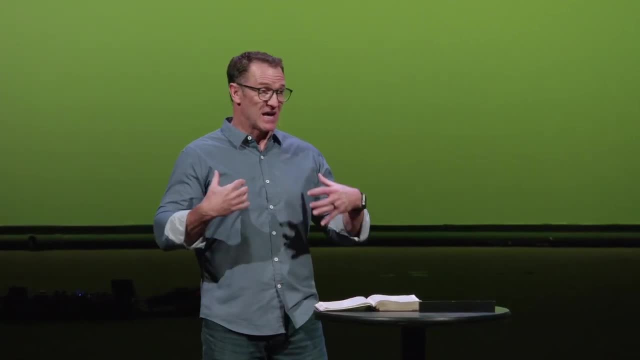 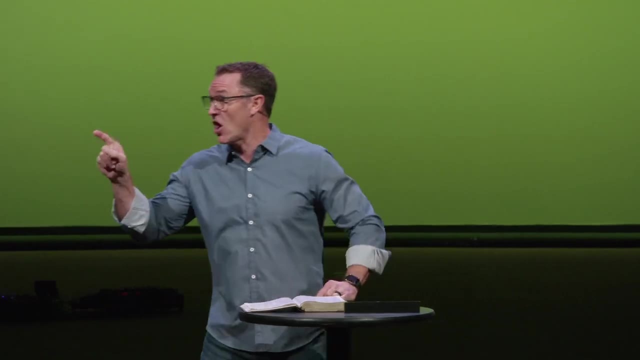 is that Jesus has paid for our sins And, because of that, his love for us, that we are so drawn to him that he starts changing our hearts, And the scripture says: he'll take a heart of stone and turn it into a stone. 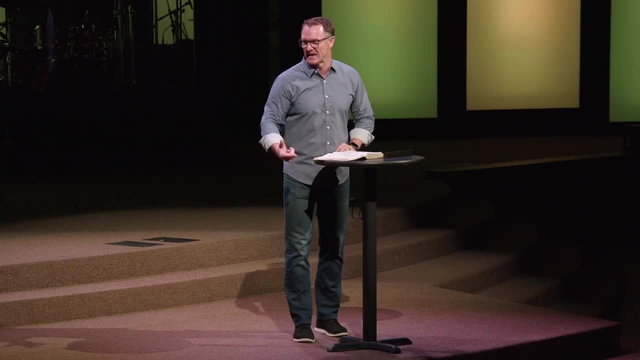 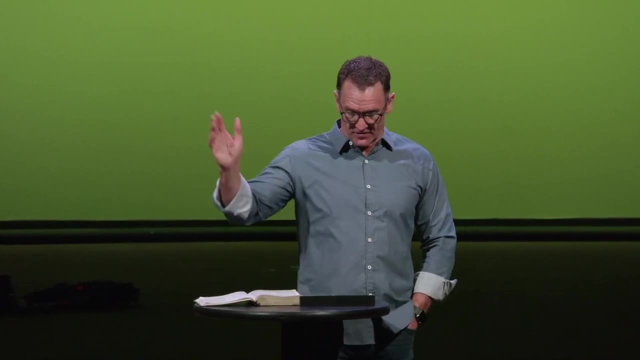 He'll turn it into a heart of flesh, giving it feelings again, giving it love once again. Jesus is our one hope. And, by the way, if you're doing fill-ins, I gotta hit five or you're gonna come after me, I know. 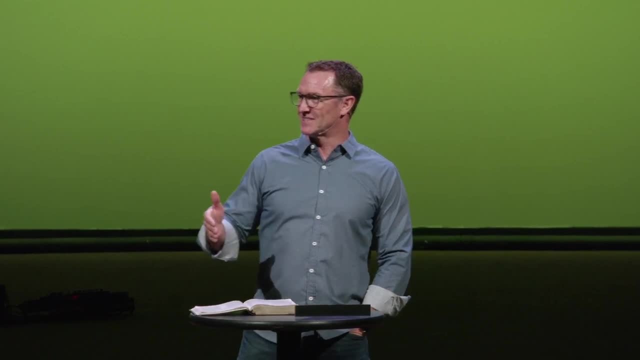 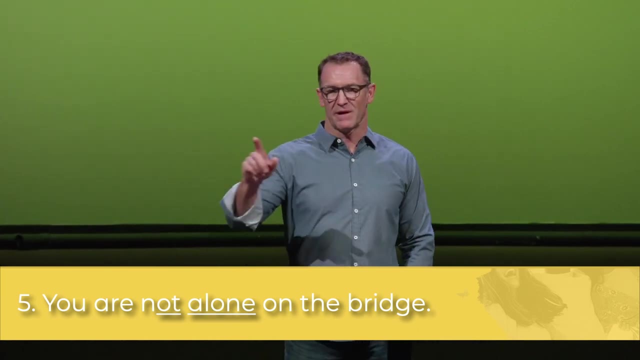 I'll just say this: You're not alone on that bridge, because it says that Jesus is in all and it means that he's in all believers And he's our one hope, That person you might have conflict with if they're a believer. 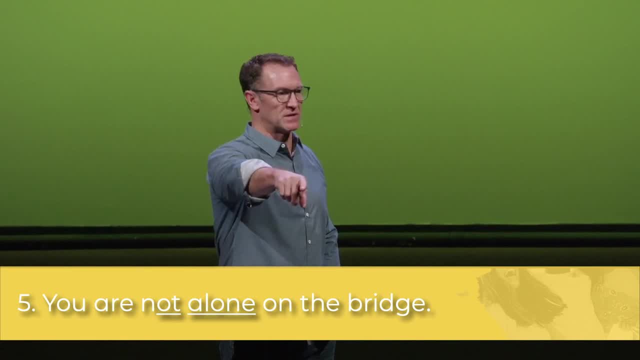 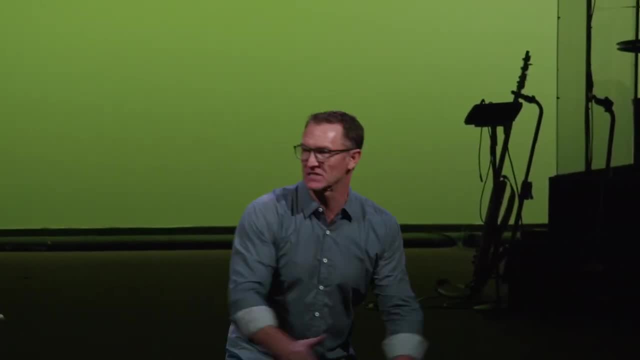 the Holy Spirit of God lives inside them. I just want to be super clear on this, because in an argument and a disagreement, everyone's wondering this: Whose side is Jesus on? Is he on their side or their side? Let me make it super clear. 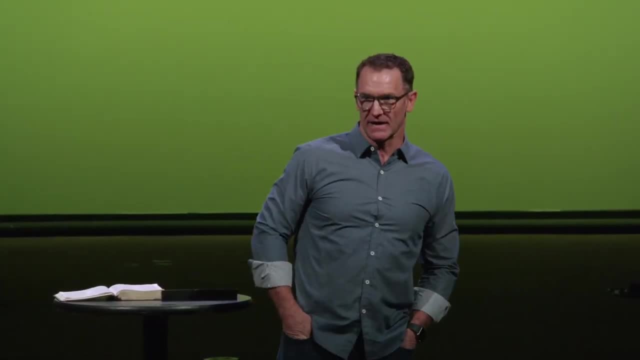 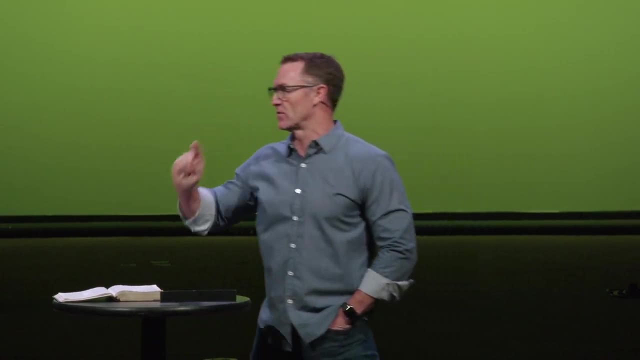 Jesus is never on your side. How's that? Jesus is never on your side? You can only be on his side, And if you choose the unity of the church, you will always know that you're on his side. Want to know what's crazy? 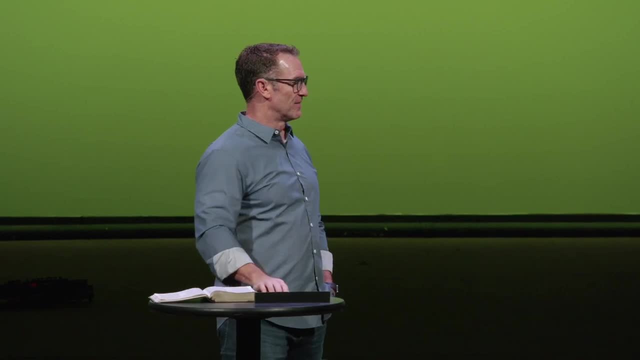 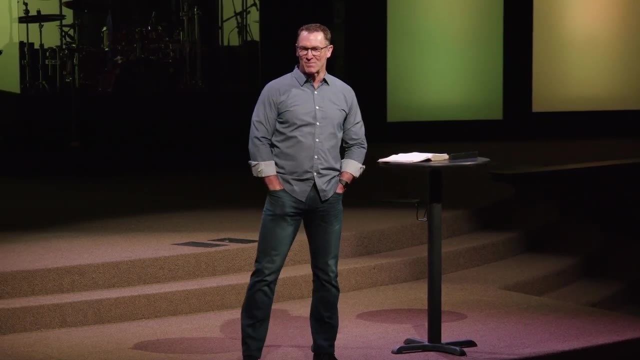 This afternoon I'm gonna get in a car with a friend of mine. He's a pastor And he and I were gonna drive about an hour from here today And we're gonna go meet with a church. There's a pastor there who's been there like three decades. 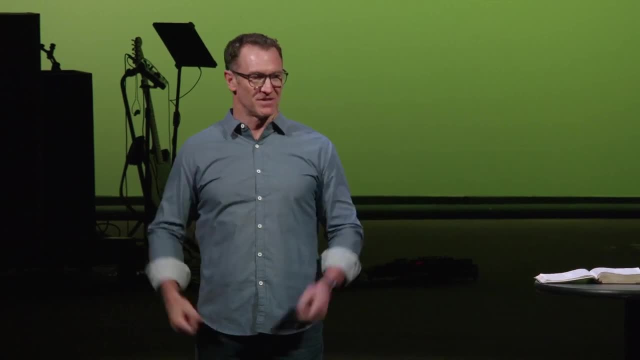 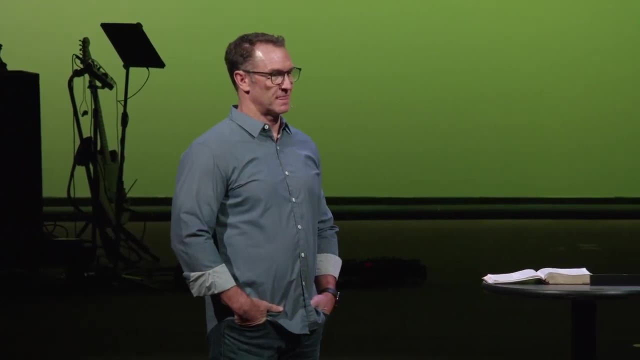 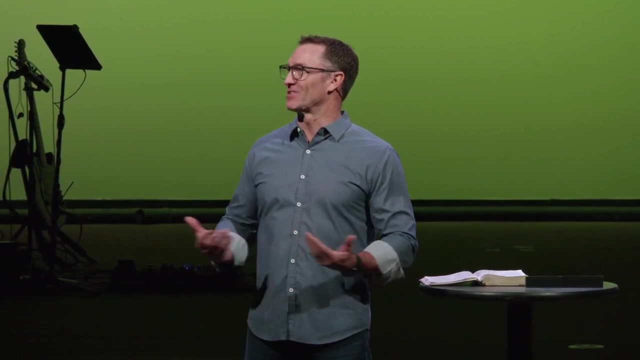 And the pastor and this church. they're at odds with each other right now. It can't get along. They don't see it the same way, And so my friend and I are going there and we're mediating- We're actually mediating his departure. 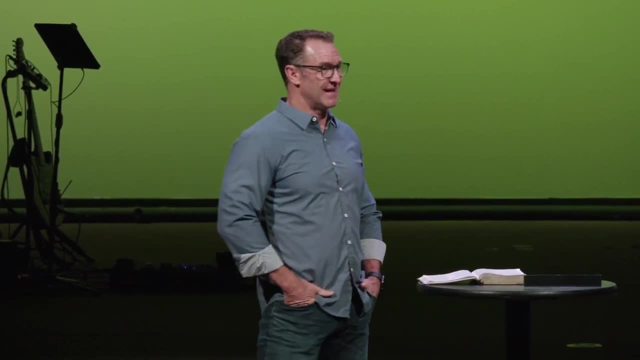 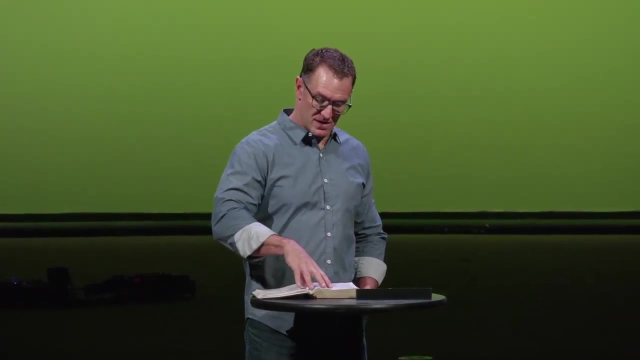 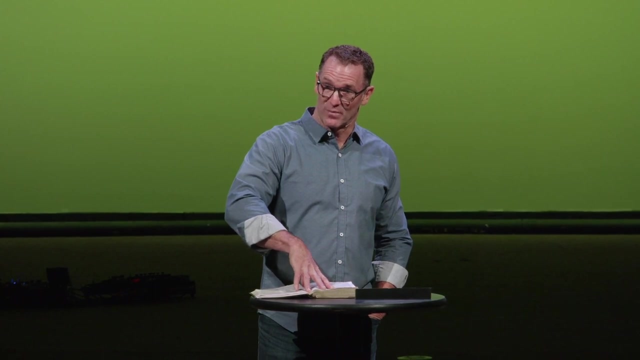 I don't know what that does to you, but being a pastor, that wrecks me inside, Knowing what it costs Jesus and knowing what it's supposed to cost us- complete humility and gentleness, patience and bearing with one another. And yet there's been such a lot of people. 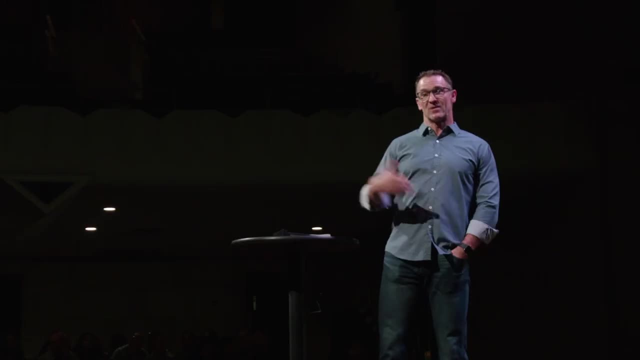 that have been there. And yet there's been such a lot of people that have been there, And yet there's been such a lot of people that have been there. And yet there's been such a breakdown for so long in this church that now we're gonna go drive down there today. 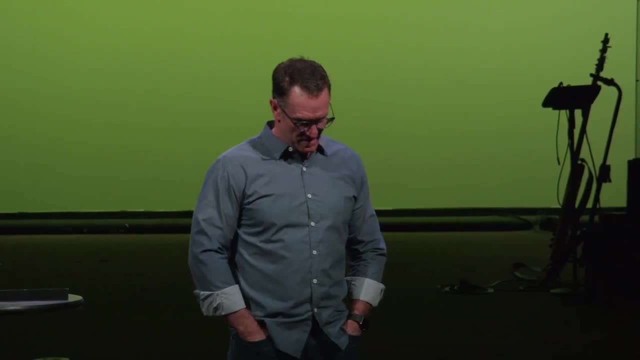 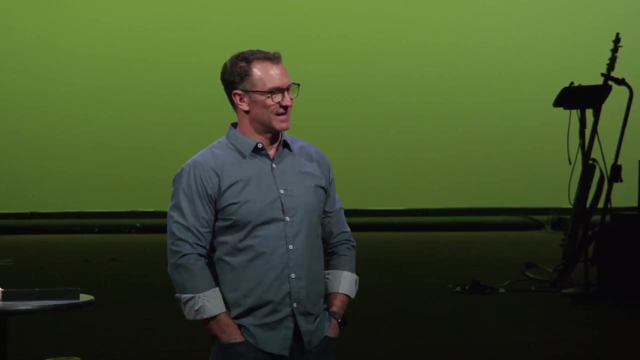 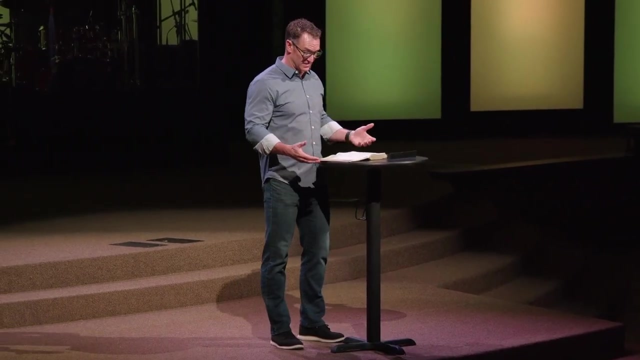 and just go mediate this thing tonight. But it's actually mediating a breaking apart instead of a coming together, which is just wild to me: That God knew that this day was coming, that I would be a part of that And somehow that this text would land in front of us today. 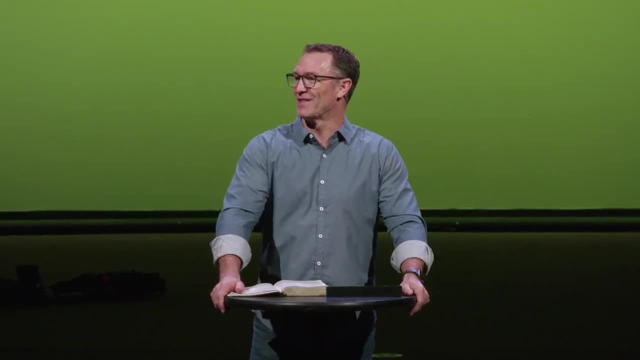 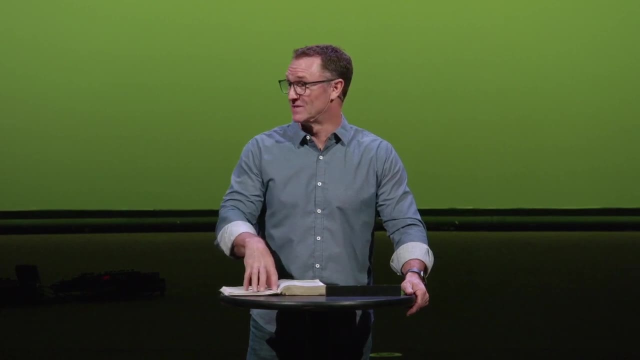 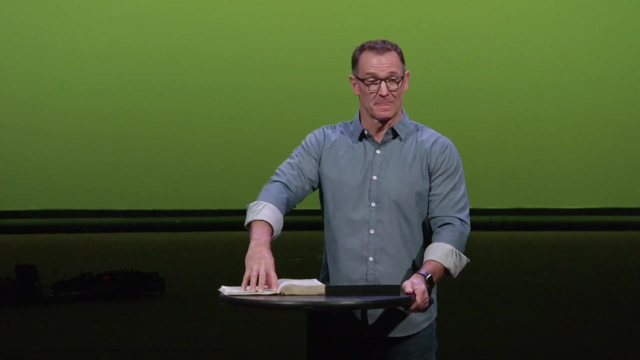 I guess, maybe through all of that, I would just be reminded of this, that we have a lot of work to do in this department. Don't be that church that I'm going to tonight, Whatever it takes. Complete humility, gentleness. 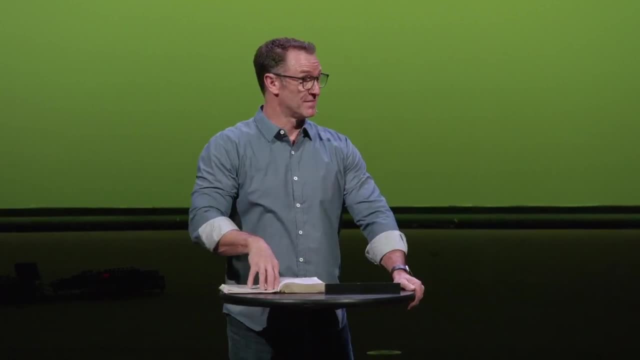 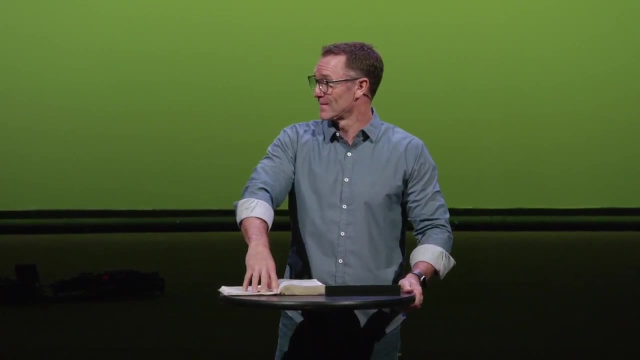 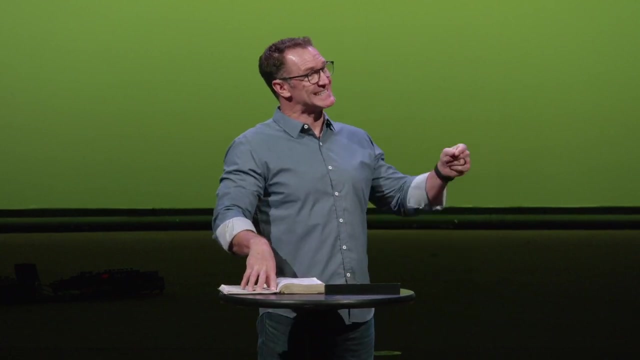 setting aside your rights for somebody else's, even if they don't deserve them. That's the gospel: Being super patient with people, Bearing with one another in love. Doing that, knowing that our reputation, our expectation is at stake in this town. 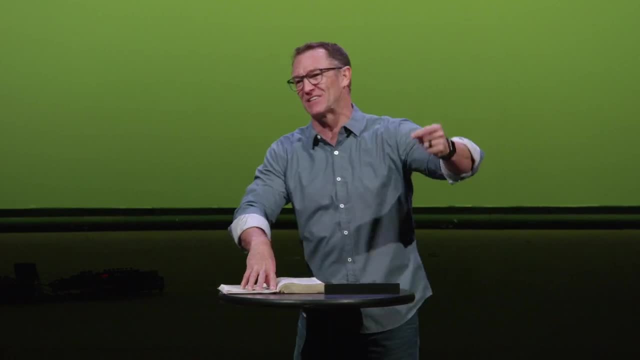 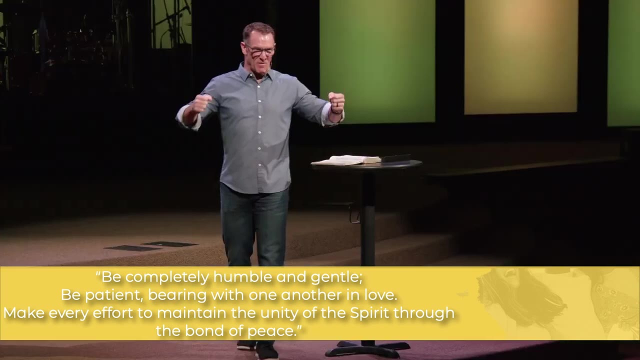 So that when outsiders look at us and they're so sick and tired of an election year marked with isolation and aggression and conflict that they walk in these doors. you are prepared and ready to build a bridge with them so that they belong and they are loved.